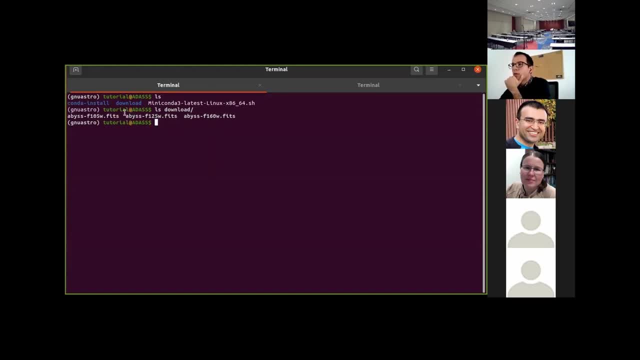 more complicated things, and I will show how to use, for example, different images for painting color images. Okay, so let's start step by step. Once you have installed GNU Astro, you can use all of the programs that correspond to the GNU Astro collection of programs this way, So you just 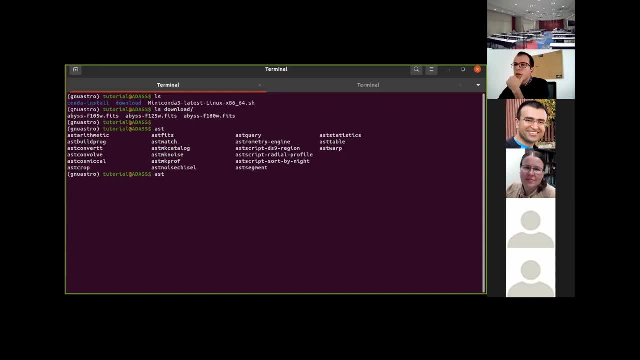 have to type in the command line ast and then you will see all of the programs that belong to GNU Astro. All of them start with the letter ast. So you have here different programs with different purposes. The only one that is not part of GNU Astro is this. one is a strometry engine. that corresponds to the 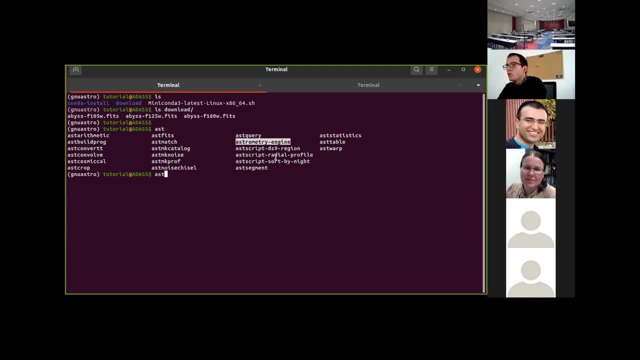 to the astrometrynet software for obtaining the astrometry of the images. But the good news is that right now we are working really hard in order to include all of the necessary libraries and programs in order to make the astrometric, to obtain the astrometric solution of the raw images. 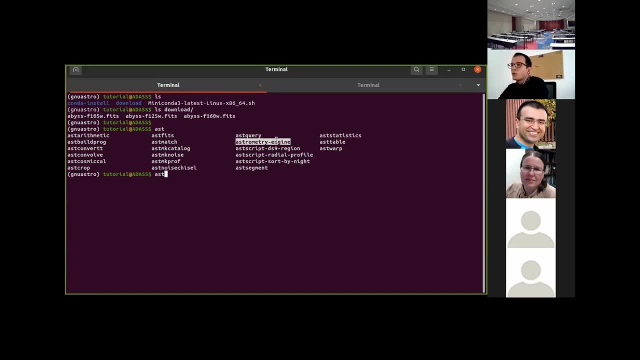 of astronomical raw images just using GNU Astro from scratch. So we hope to have everything ready in a couple of months, And now we will start reviewing the programs of GNU Astro. So the first one that we are going to use is astfeeds. 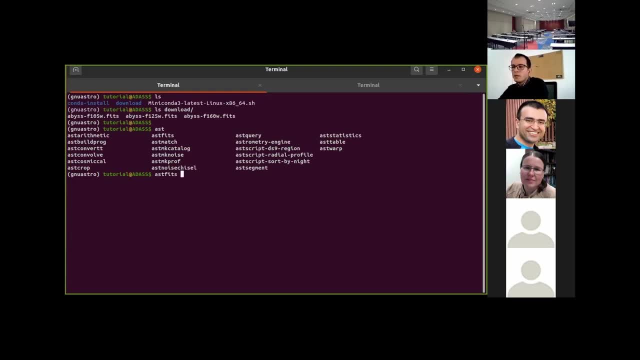 This is one program that we use a lot because it main purpose is to check the metadata of the images, the headers, and manipulate that metadata. So the way you have to use this program is just to type in the name of the program on the command line. 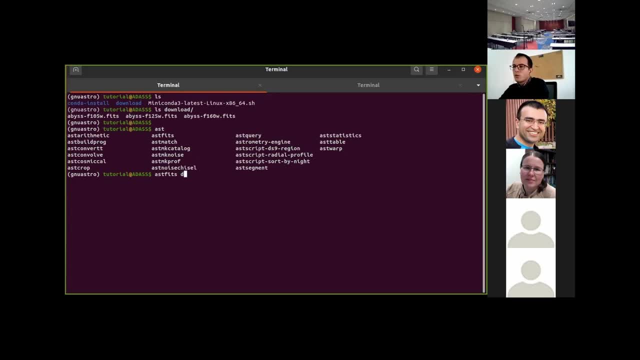 And now the name of the image that you want to check. So, for example, the image in this image, in this filter, And the first thing that you will see is that it prints on the command line the name of the program, the version of the GNU Astro. 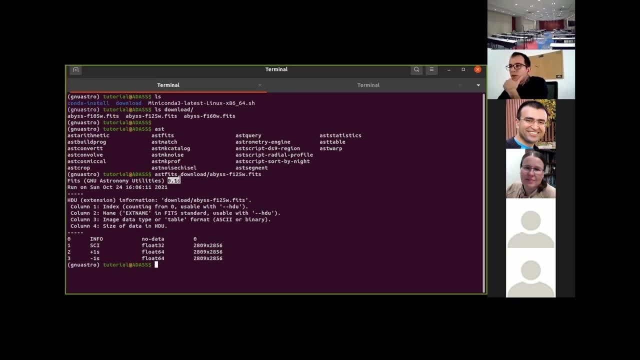 in this case, we are using the latest one, 0.16.. And then it gives to you all of the information related with this with this file. Okay, So in this case, it says to you that you have four different extensions. 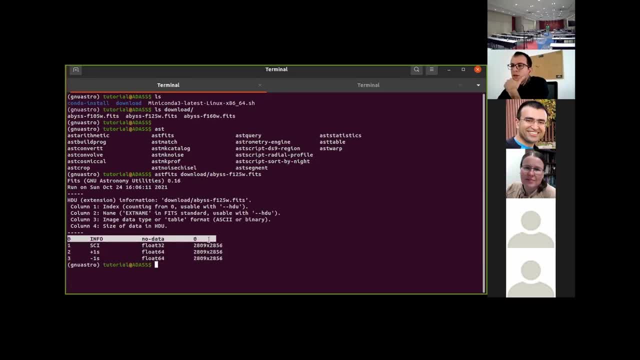 The first one is just the information. It contains no data- And then the next. the next one correspond to the two images, So they are a type of fraud: 32 images with this dimension. Okay, So now, if you would like to have a look at the inside of uh, for example, the first extension. 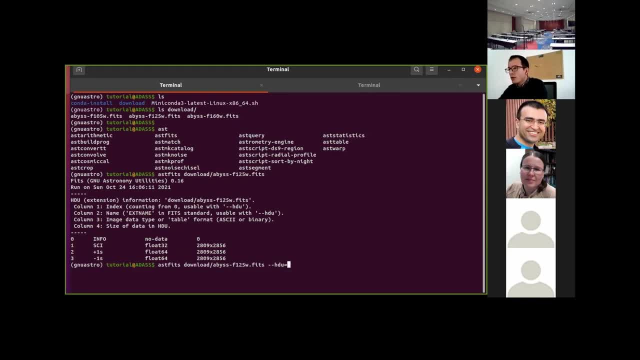 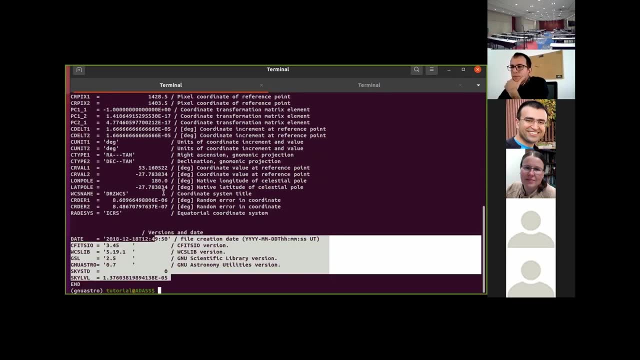 you just have to type here: dash, dash, H, U equal to one, and then you will obtain the header of this first extension. Okay, So this is really simple. Then, the way you have to specify this, you can. you can let the here one white space. it will give exactly the same, or with shorter. 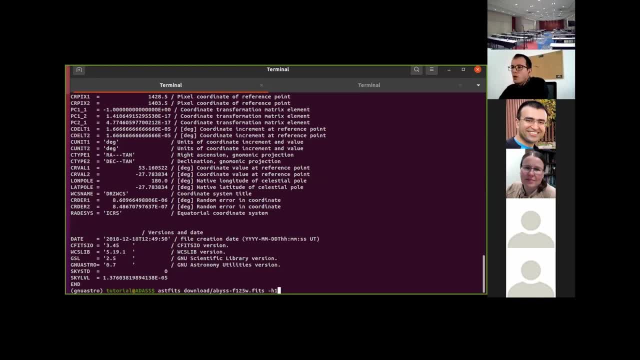 options. So for example, H one or H white space and one. So they are the different ways we have to specify the arguments of uh, of the Denoastro programs. So let's continue on little by little. So one of the things that we another very interesting thing is that uh is the option, for example, dash, dash. 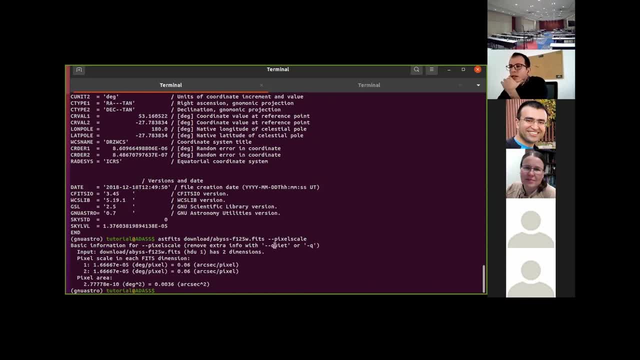 pixel scale And, as you can see here, this is going to give to you some information related with the world coordination. Okay, So, for example, the size of uh, of the pixel along the two different dimensions, in degrees or in arc, second per pixel, which is more common in astronomy, And then also another option: 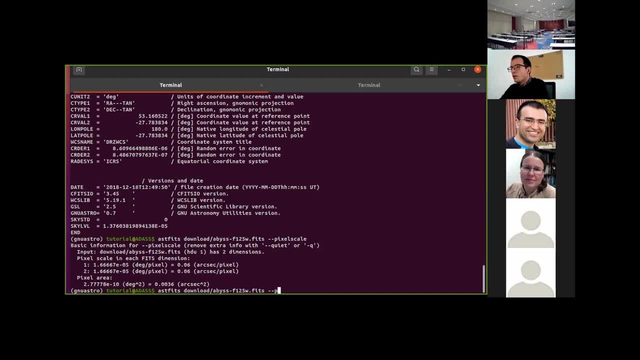 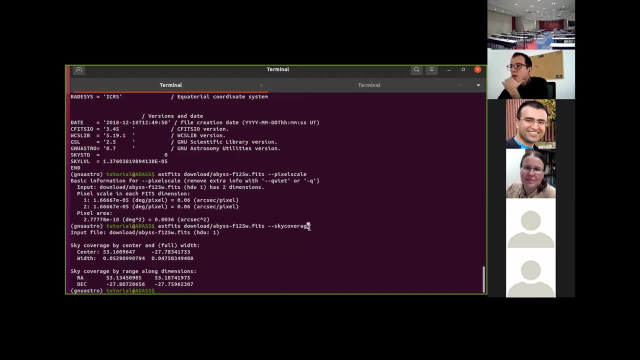 that, uh. another interesting option that you can use is the sky coverage. Okay, So if you type here sky coverage, this command line, then it gives to you all of the information about what is the region of the sky. Okay, So if you type here sky coverage, this command line, then it gives to you all of the information about what is the region of the sky. 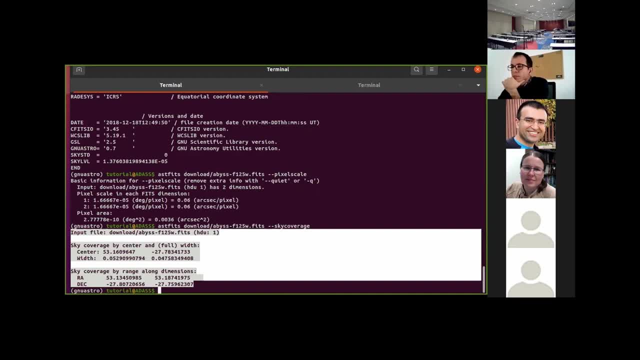 Okay, So if you type here, sky coverage, this command line, then it gives to you all of the information about what is the region of the sky that is covering this, uh, this image. Okay, So all of the different options that are. 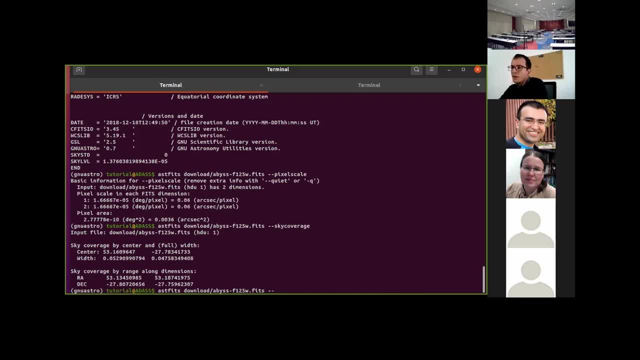 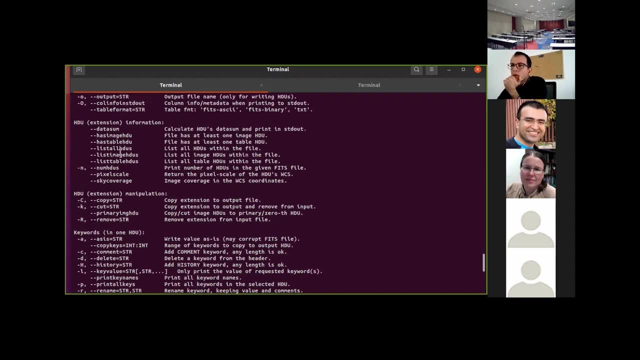 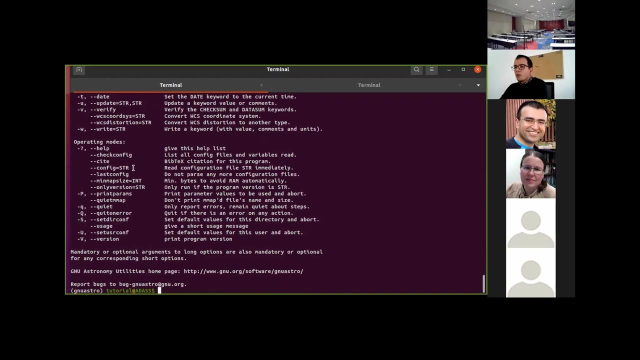 available for each program of Denoastro can be seen with the option dash, dash help. So by doing this, you will see all of the different options that you have that you can use with this particular problem. Okay, Okay, Let's continue. Let's go Um. now we are going to manipulate. 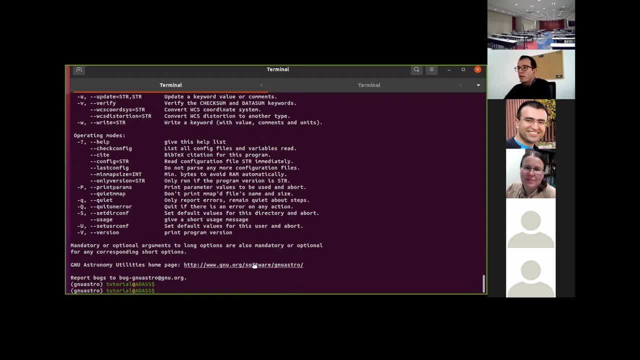 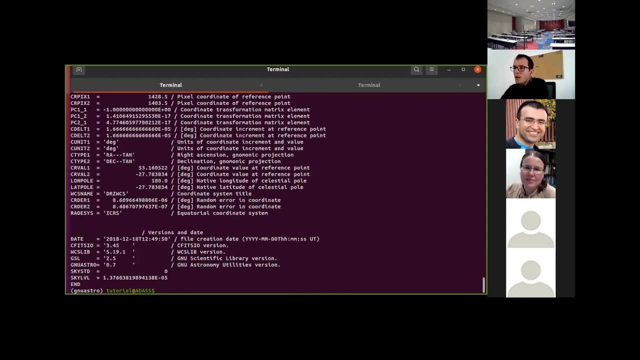 some of the keywords that are inside of the of the of the extension number one. So, for example, let let's have a look at the extension number one again and now we are going to buy these into prep, just to have a look at which lines 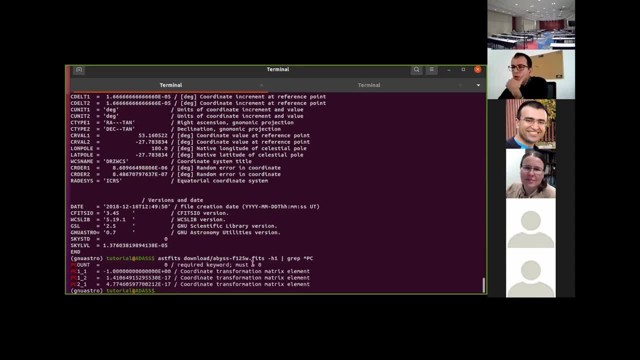 start with the keywords PC. Okay, So you will see that here we have four different uh lines, and now consider, for example, that we would like to remove these two different keywords because the numbers that we have Here are very small or for any reason. you just want to remove these two different lines. 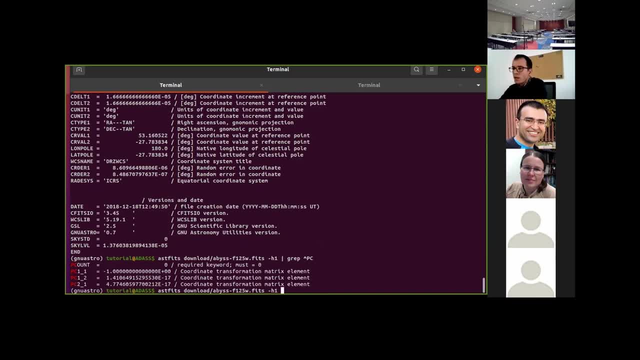 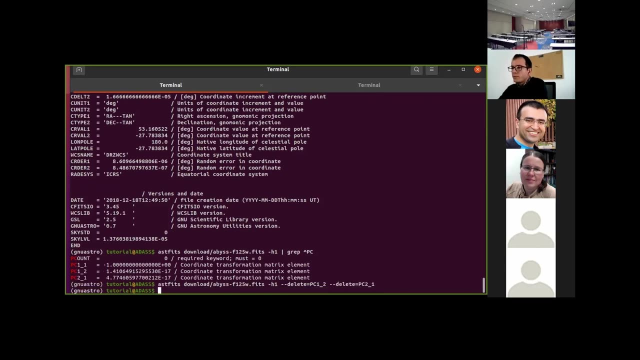 So the way you have to do that is just specifying here dash, dash delete and then the keyboard: PC one, one, two and dash dash delete. easy to one, Okay, And if you have a look again at the image you will see that all they have been. 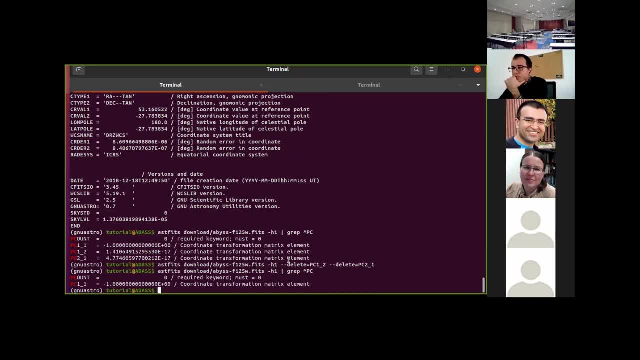 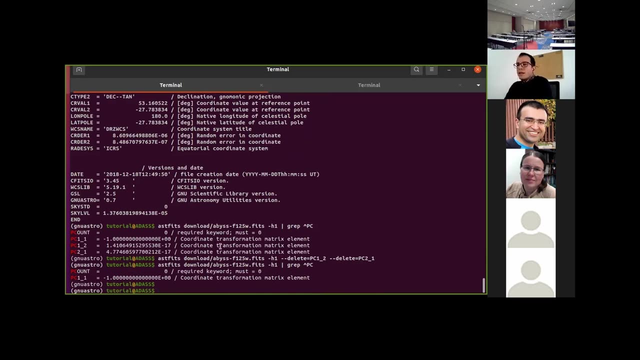 removed. So this is very powerful And you can see that just directly from the common line we can manipulate and also obtaining really useful metadata from from our images. So now let's have a look at the image itself that we are going to use along the tutorial to do that. 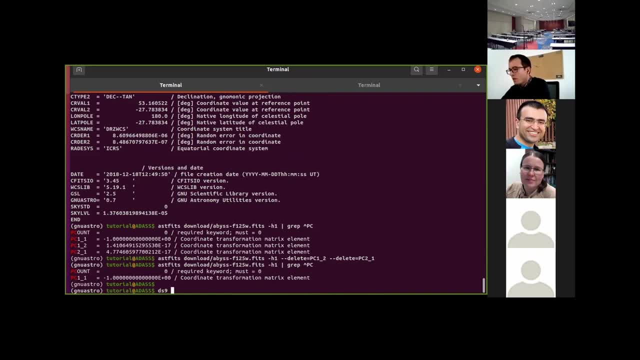 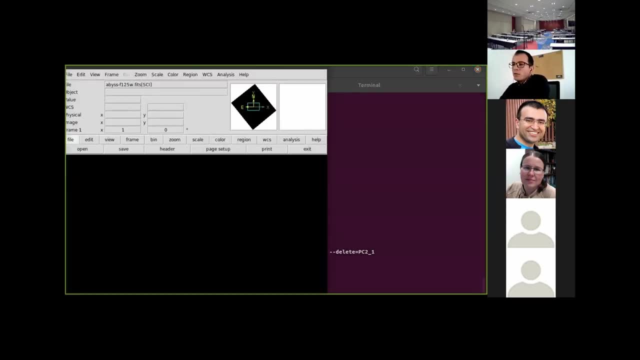 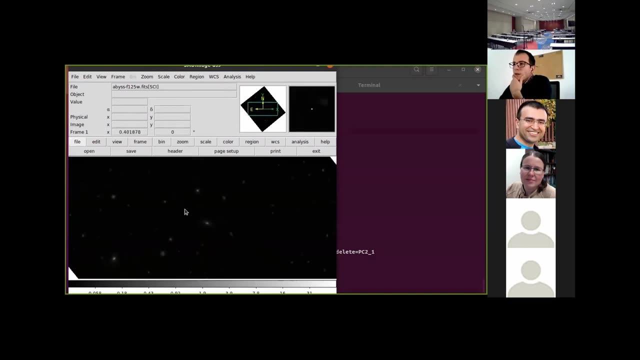 We are going to use DS9, this program for visualizing the astronomical images. So this image again, just to have a good feeling of what we are going to use, uh, along this tutorial. Okay, Just to see the object, the astronomical objects, in this image. let me change the scale. 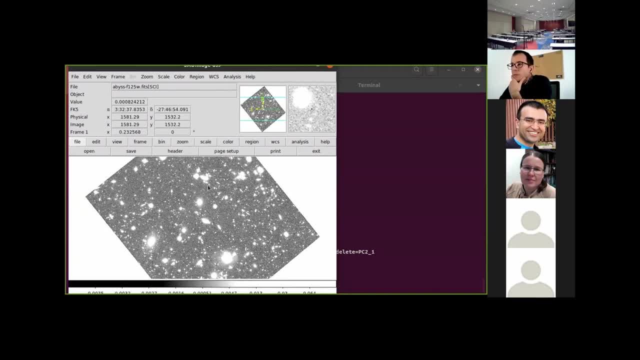 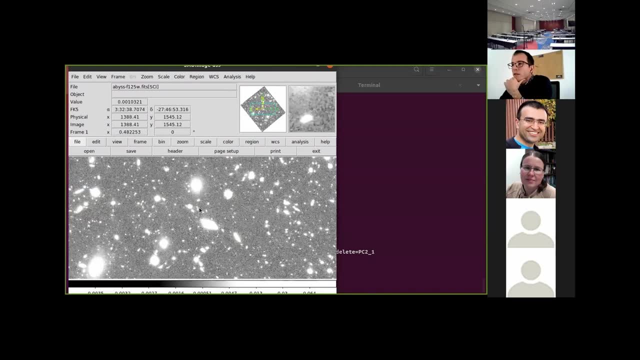 Okay, And here you can see that, um that this image correspond to the Hubble ultra deep field And, in this particular case, these images was, uh were reduced by Alejandro Burlap by the time he was, uh, PhD. 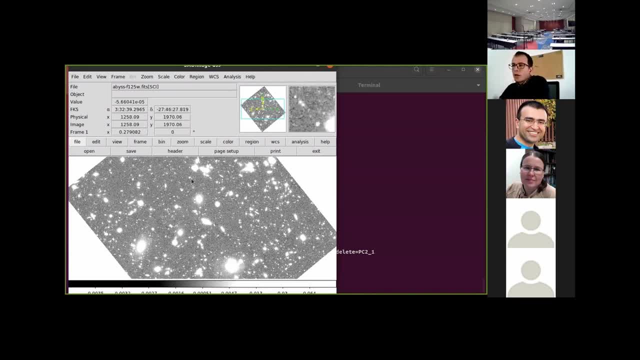 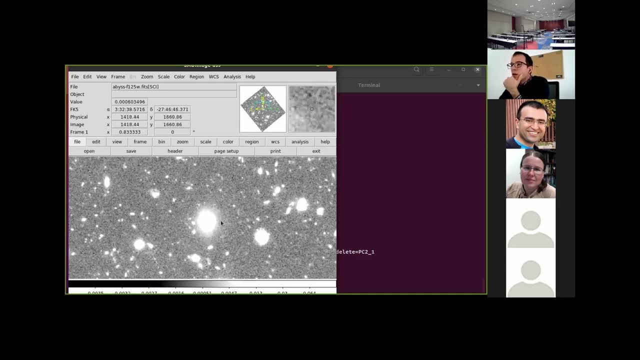 a student at the Instituto de Astrofísica de Canarias, and the main goal of this work was to reduce completely from scratch all of these images to preserve the low surface brightness structures around the galaxies. So he used many different programs from the new astro in order to model. 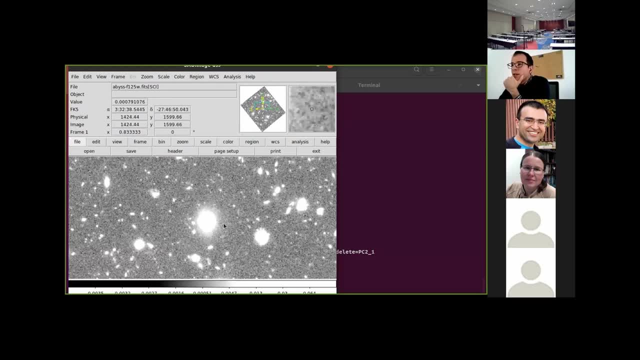 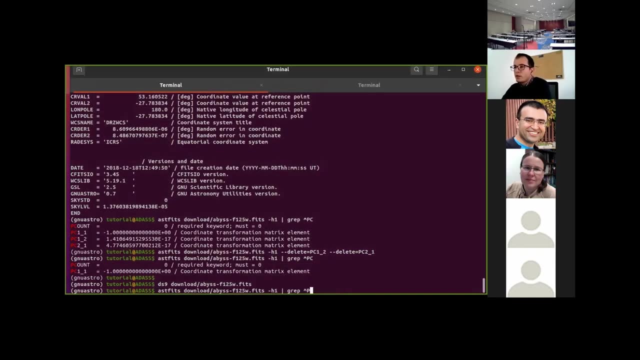 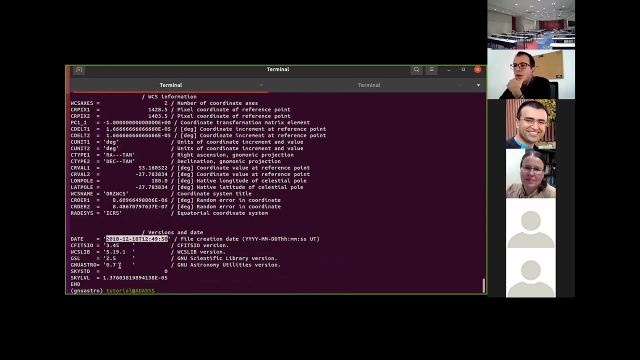 the sky appropriately and then preserve that kind of very low surface brightness structures. And, as you can see here, if I do again, AST feeds dash one. you can see that, but that time Alejandro Volar was using GNU Astro 0.7 and now we are using 0.16.. So since then we have improved. 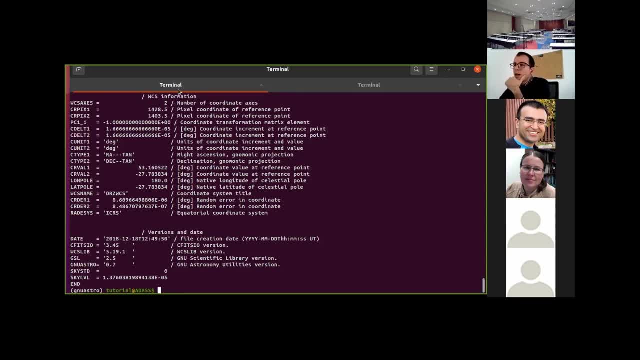 a lot GNU Astro, all of the GNU Astro programs and libraries- and it is much more mature and it can do very powerful things, as we are going to see. So let's continue with the next program I want to show here. It consists in the AST. 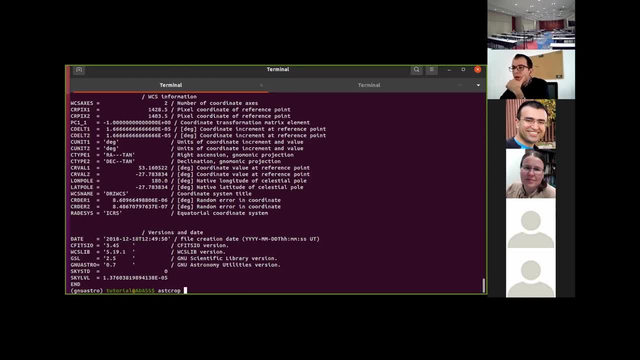 Drop program and the main goal for this program is to make cuts of images, So just to select the different region of one image. So, for example, if we specify here again an input image which is going to be exactly the same, then we can give some coordinates and some width. 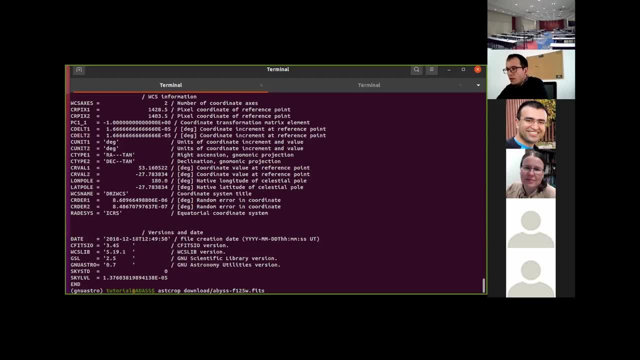 in order to have a crop of the of the image. So, since we are going to provide right ascension and declination coordinates, we have to specify here that the mode is in wall coordinate system. And now we have to provide the center, And I will give this center, which is centered in one 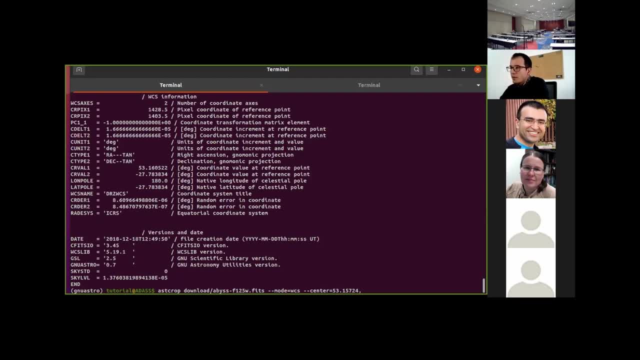 particular galaxy. This is the right ascension, the declination 27.. And eight to five, to three. And now we specify the width, the size of the inch. We say we want 20 arc seconds, So we have to divide this by 3600, which is how many? 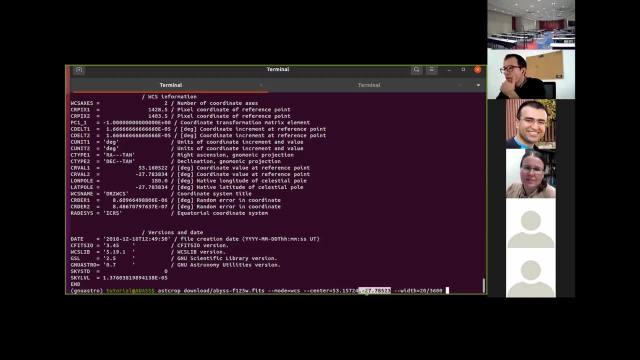 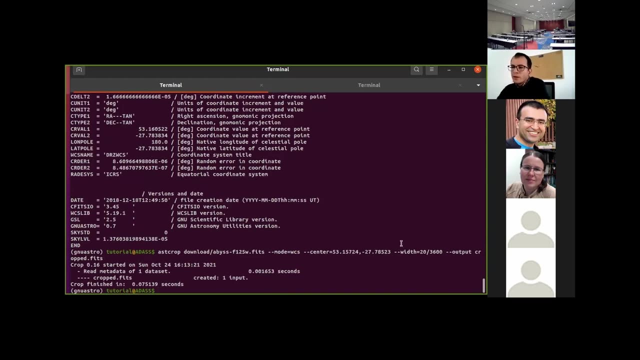 arc seconds are in one degree, because here we are specifying the coordinates in degrees And now we can give an output name. So dash, dash, output. And for example, if we run this, you will see that just in less than 0.1 second it has computed the 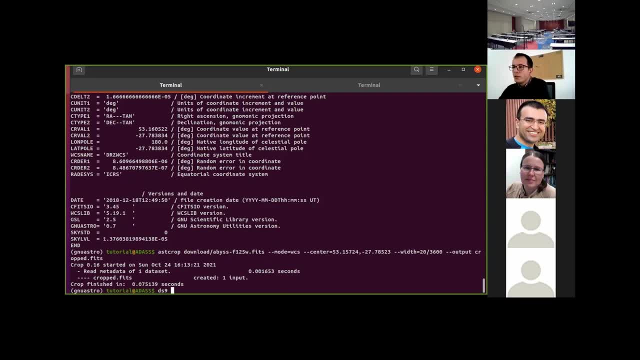 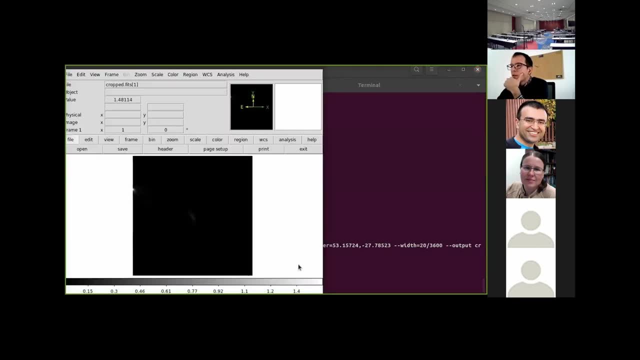 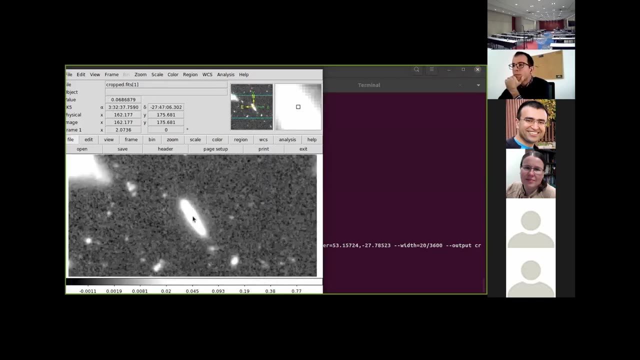 crop from the original image. So now let's have a look. This is really really fast, as you can see, And this is the result that I am obtaining, So a smaller image that I was able to construct just directly from the command line. As you can see here, we can have a look now with AST. 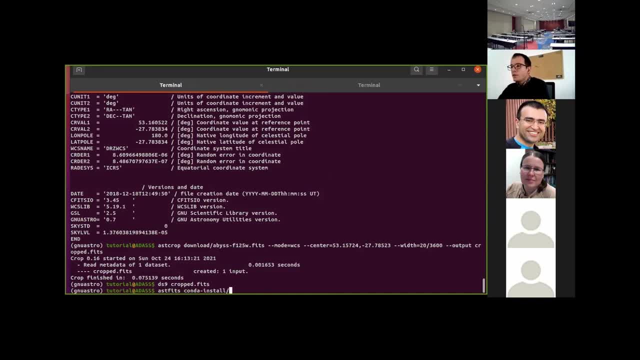 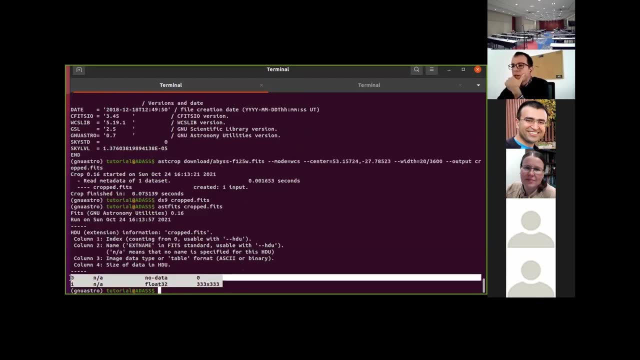 that fits at this image. Just to sorry crop, Just to check that again. we have two different extensions: The first one just with metadata And then the size, so the dimension of the second extension and the data type. So now let's do more complicated things. So let's open again. 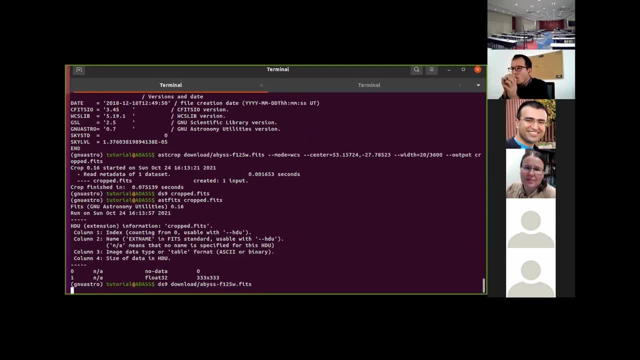 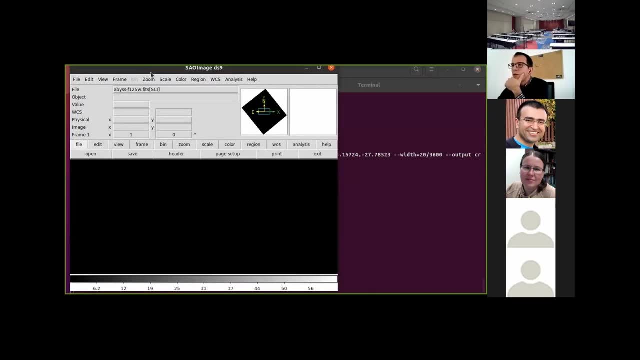 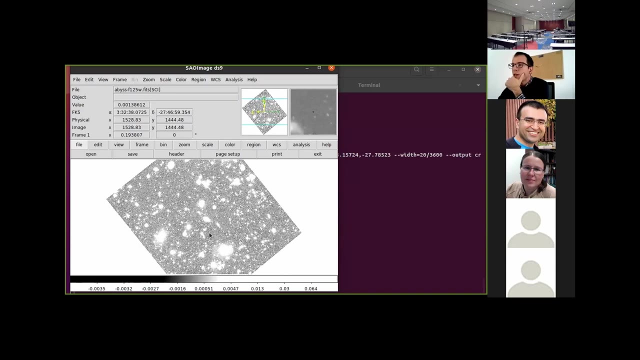 the same image just to show you how we can obtain a more complicated the crop regions, Because a square one was really easy to do. So here again, let's make, let's change the scale. So, for example, imagine that I would like to crop a very 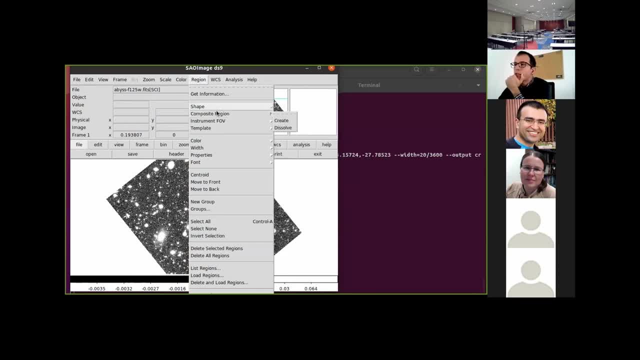 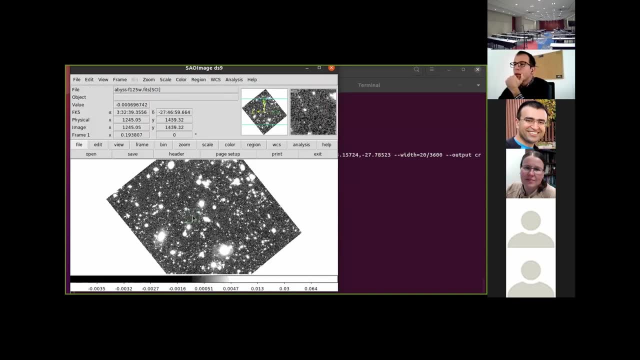 strange shape of this image. So go to region shape. and now we are going to change the shape to polygon. Okay, And now we are going to define here a very strange polygon on the image. For example, you made your, your the shape of the polygon as you want, Okay. So for example, 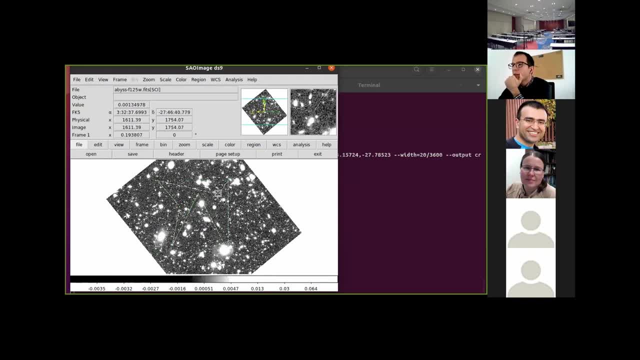 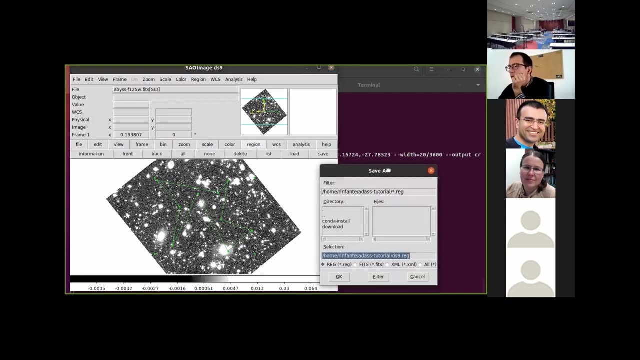 something really strange, which in principle, makes no sense, But this is just to show an example. Okay, So now that you have defined this, this very strange polygon, you just have to go to region save as a DS9, as a DS9 region. Okay, I also put here also: 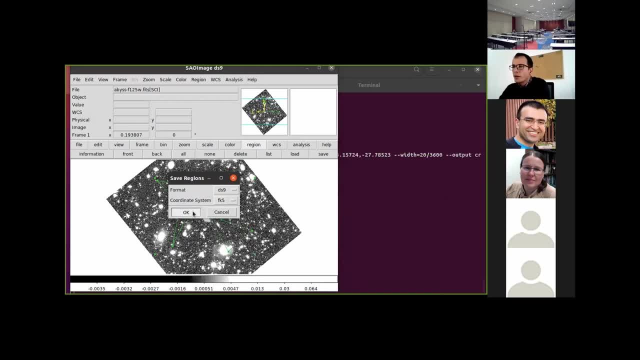 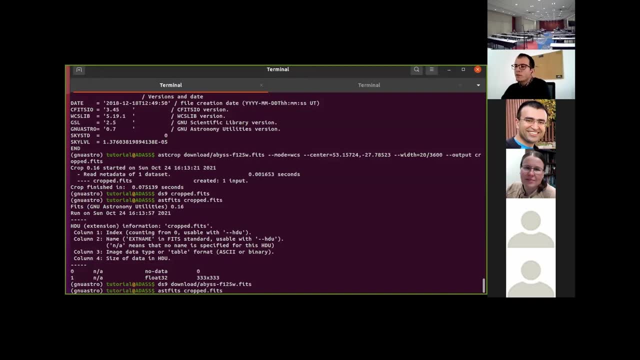 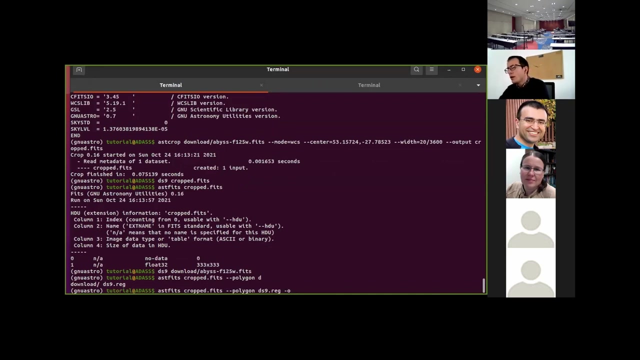 I always put here degrees. Okay, I save this, Plus remember the shape, which is really strange. And now you just have to specify this very strange region with the option dash, dash polygon, and then DS9,, DS9 region, And let's put a good name. So, for example, dash output polygon. 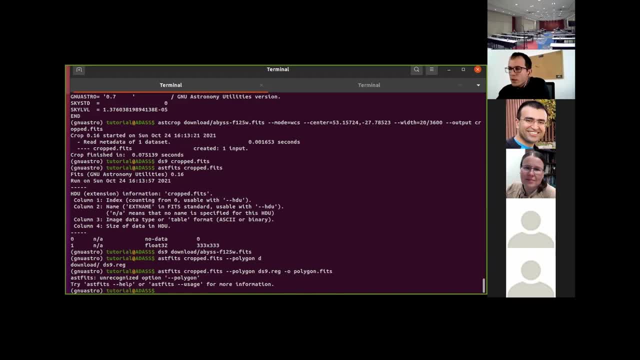 Fits What's happening here. I'm having here the bit the AST fit, So AST cropped the original image. Sorry, I was specifying the already cropped one. So, just very briefly, AST cropped the image that we want to crop. So the original image. 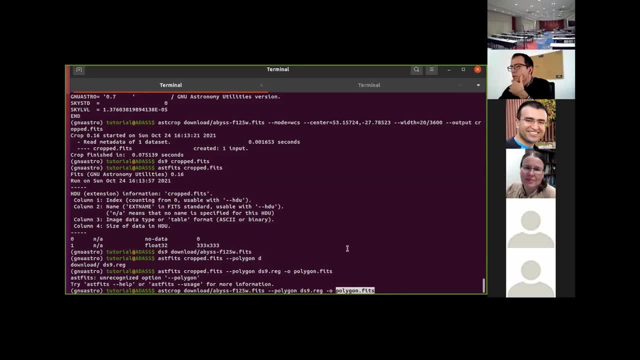 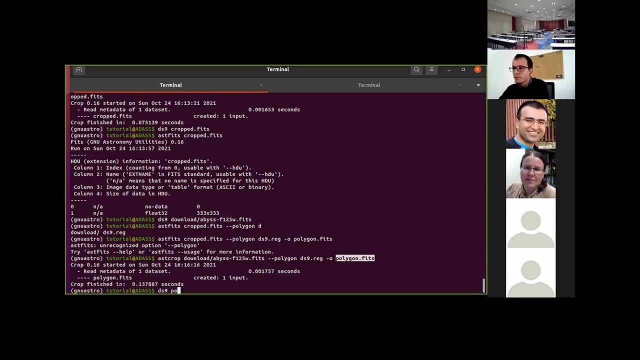 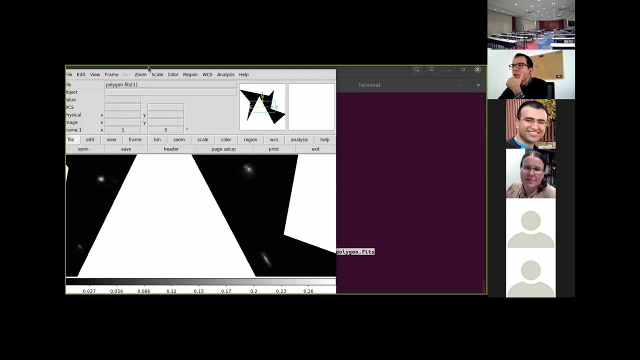 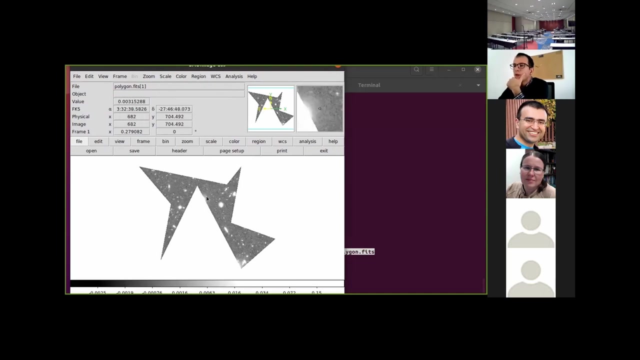 then the option polygon, with the regions, and then the output name. So if I execute this, you will see that in this case- polygon- we have the output image with that region that we have previously defined. Okay, So very strange. but this is just to show that we can make very complicated things with this. 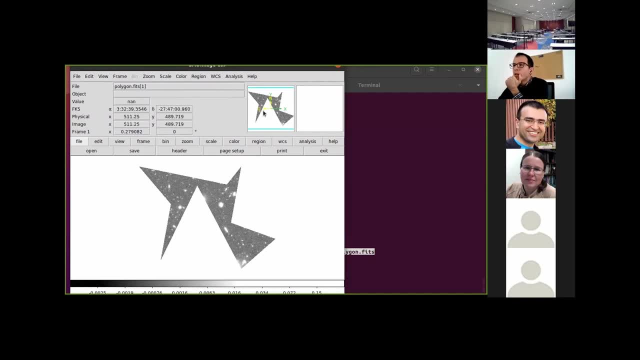 with this problem. And another very interesting feature is that it preserves by default the world coordinate system, So it doesn't matter on which region of the sky you make the crop that it is going to compute the necessary new information about the astrometry of the image. 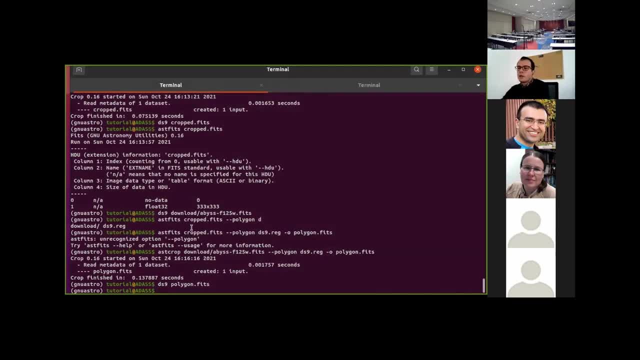 Okay, that's good. Now let's continue with another program, which is Noise Chisel. So Noise Chisel was presented. the name is this one, so AST: Noise Chisel, as you can see here. So it was presented in ADAS 2015 in Sydney, but that time this was at the very first. 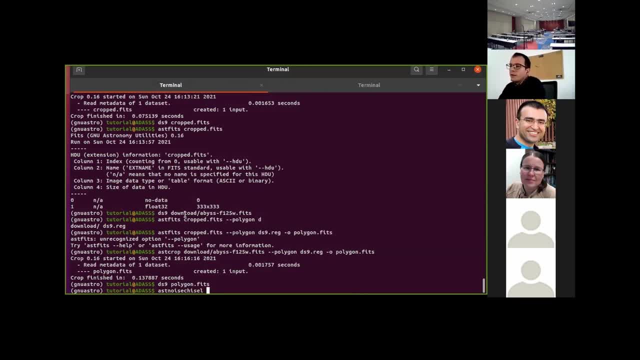 moment which Mohammad presented to the public. and since then it has evolved a lot and now we are going to see how we can use this program for making the detection of the signal of our astronomical images. So again, let's specify here the input image, that 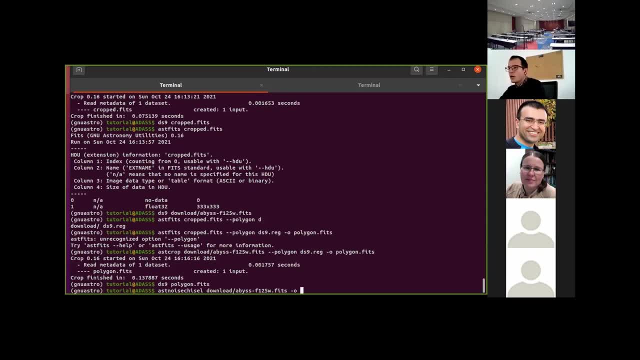 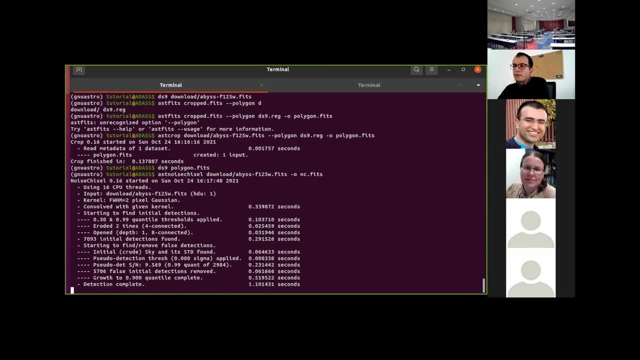 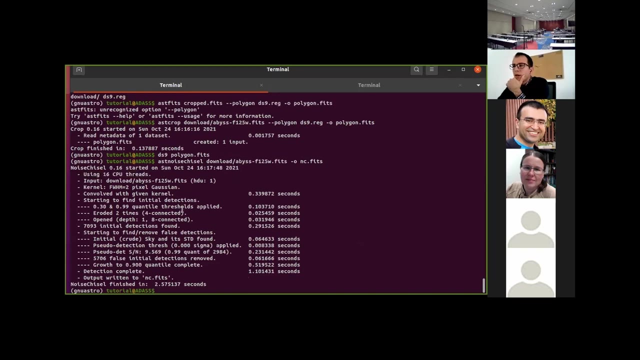 we are going to use. and now let's give a good output name, so for example, Chiselfits, And just let it run. as you can see here it is using the 16 CPU cores that I have in my laptop. Now let's have a look at the output that it has computed. So DS9, in this case, I am gonna 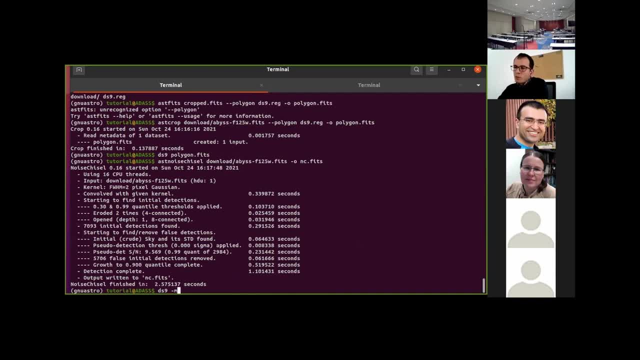 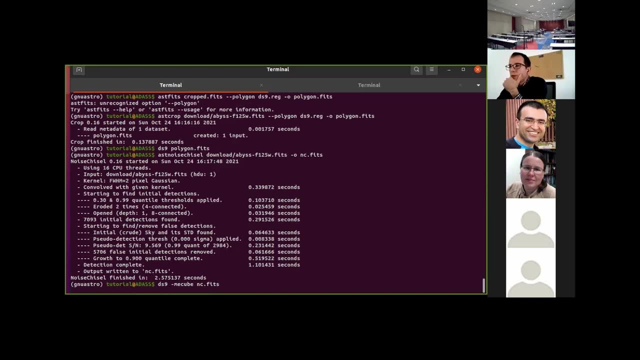 have a look at all of the different extensions, so I will type here: Multi-Extension Cube and then the Noise Chisel Output: Noise Chisel Output. press enter and now we will see the different extensions that Noise Chisel has computed. 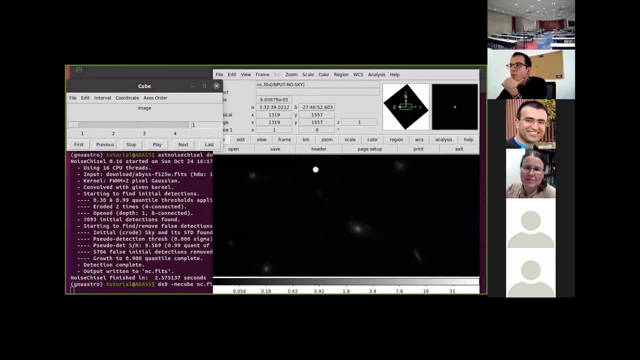 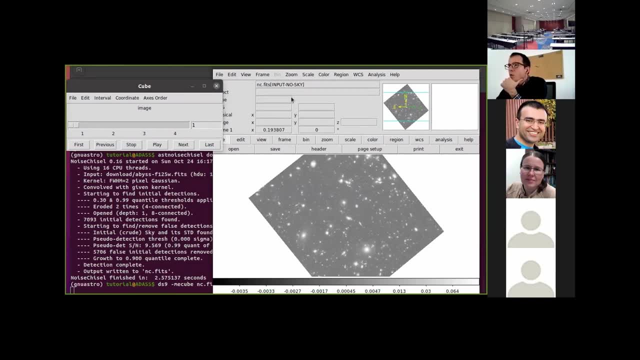 Okay, so the first one. let me change the scale once again. So the original one. sorry, the first extension is the same as the original one once Noise Chisel has subtracted a sky background model that it computes internally. Okay, so this is the very 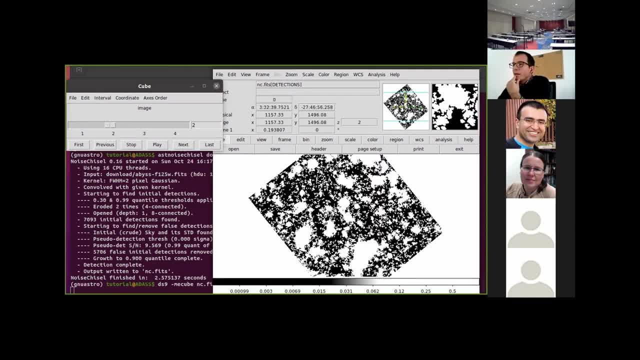 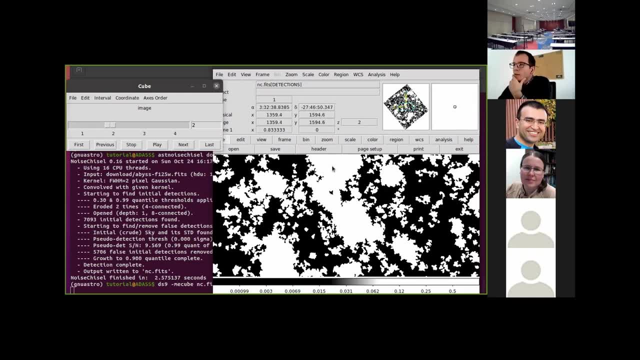 first extension that we have. The second one is the detections that it has computed. So this is a binary image in which all of the pixels that are white correspond to ones, and that means that here we have signal, and then the zeros which correspond to the black pixels. they are sky. 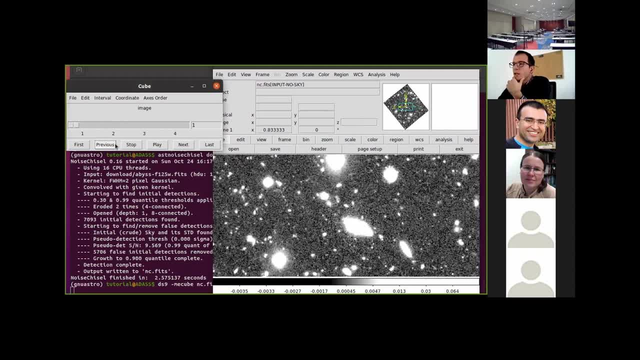 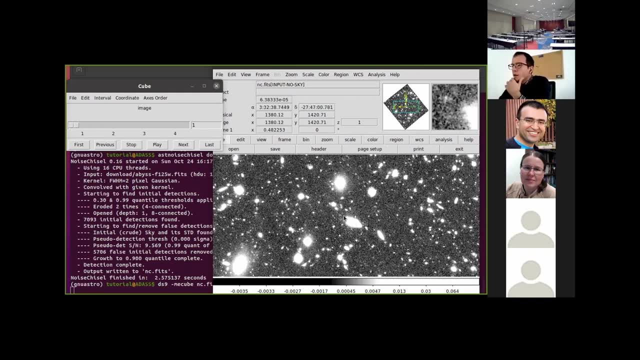 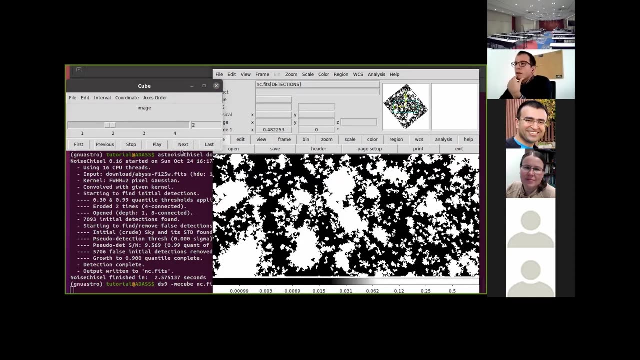 background. So if I change in between the original image and the mask, the detection image, you will see that all of the different signals, all of the objects have been detected as signals. And then the third extension is the sky background model that, when she is to compute, 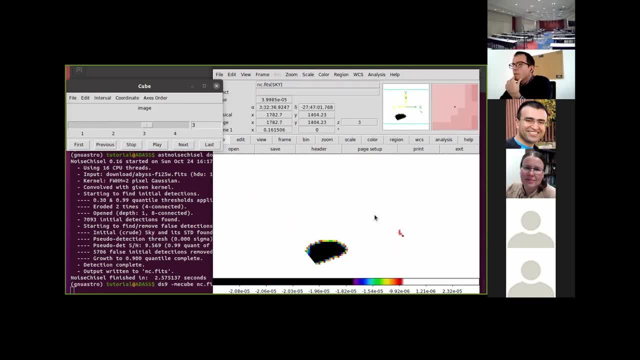 by default may be a change in the color, you will see it better. And then the last extension is the sky standard deviation. So it automatically computes this from the original image without any assumption on the shape of the detected region and so on. So this is non-parametric. 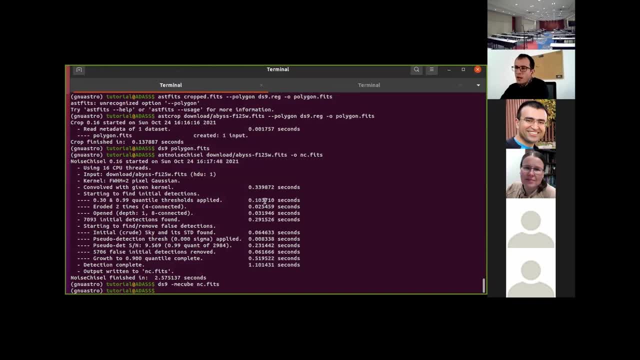 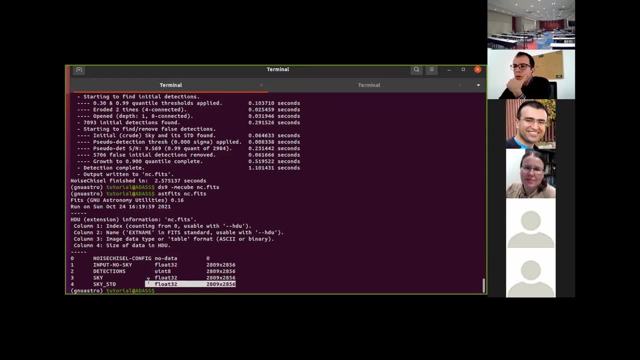 And now we can have a look at the files with AST fits once again, And this is actually what we were having a look with DS9.. The first extension is just the information that the parameters that my chisel has had used for obtaining this detection image. 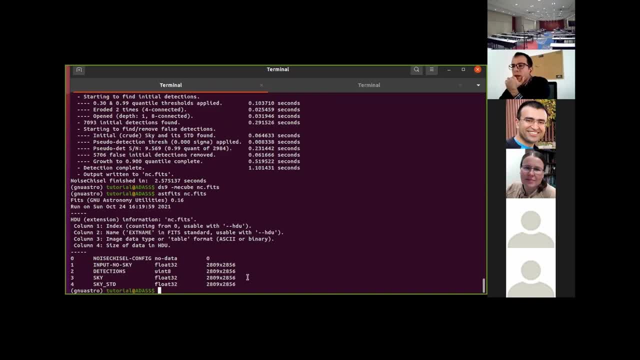 Now let's move to the next program, which is AST arithmetic, which is a program with the goal of for making calculations, the manipulation of astronomical images. So the first thing that I want to note here is that it uses the reverse polish notation. So that means that, for example, if you want to multiply two by three, 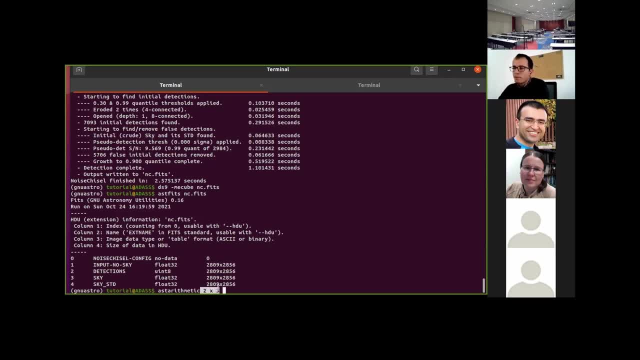 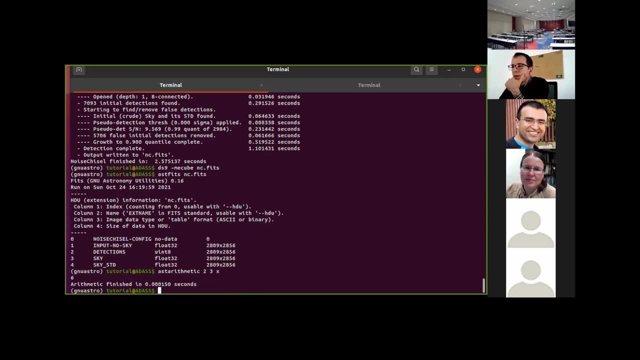 you cannot specify like this the order of the operands, like this, but you have to do two, three and then the operator, which is the multiplication, And then it is going to give to you the result. So two by three, it is six. 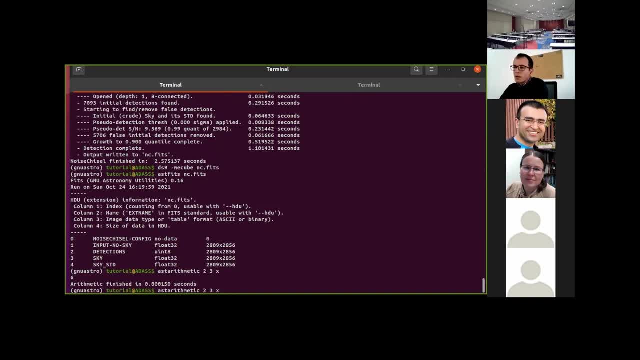 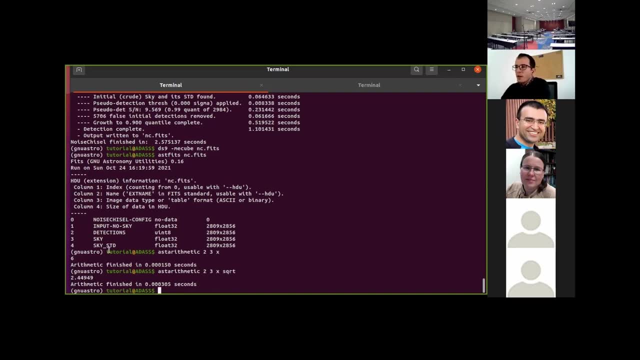 So then we have many different operators. So, for example, here we will take, for example, the square root of six and it will give to you this number. And then, for example, if you don't want to have this information, so this additional information, you just have to run in quiet mode. 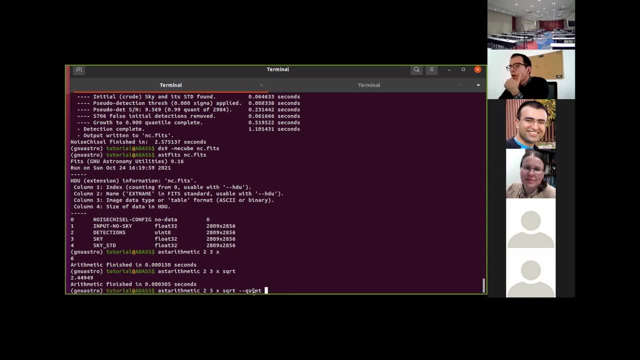 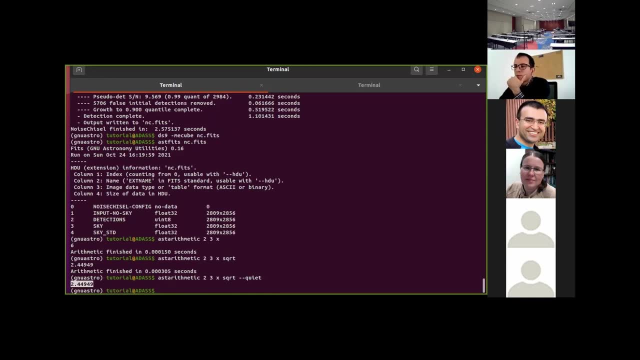 This is also common for all of the GNU Astro program, this option, And in this case it's going to show you only the number that you are asking for. Okay, this is very simple, but, once again, we can make very powerful things with this program. 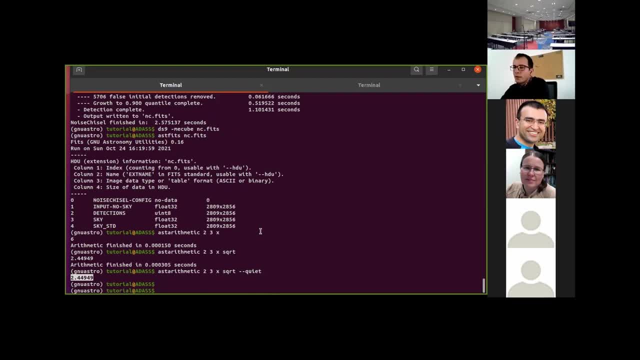 So, for example, the sum of two different images. To keep the thing easy, let's do it AST arithmetic. Now let's specify one image. We have to specify also that we want to sum, sum the extension number one of this image and then the other image, for example the. 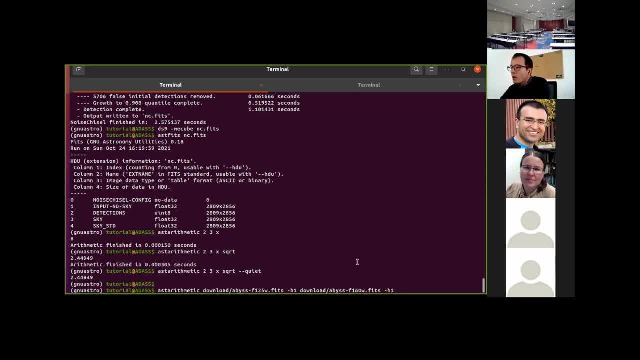 other filter, the extension number one, and now the operator that we want to use for making the operation. So we want to sum these two images, so to specify here plus, and now let's give an output name and just press enter and it is going to compute the sum of the two different. 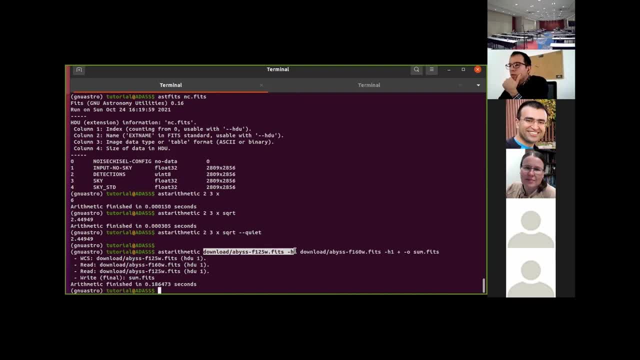 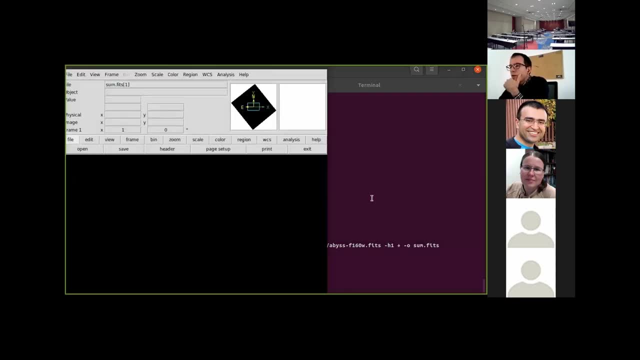 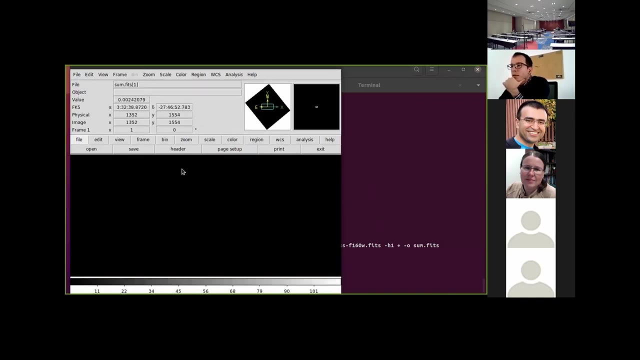 images that we are specifying here as an input. Just let's have a look very fast here to the sum image. of course this is just summing two different images, which is easy to do, but in the same command line you can sum thousands. 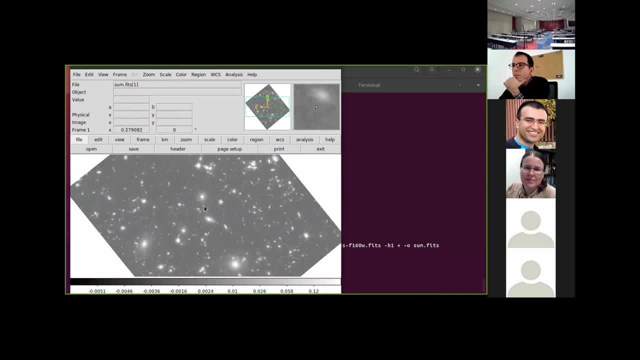 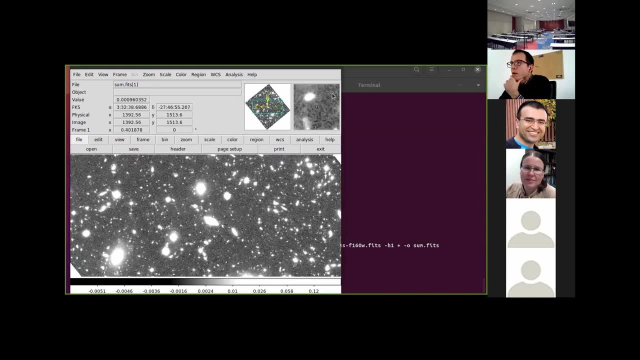 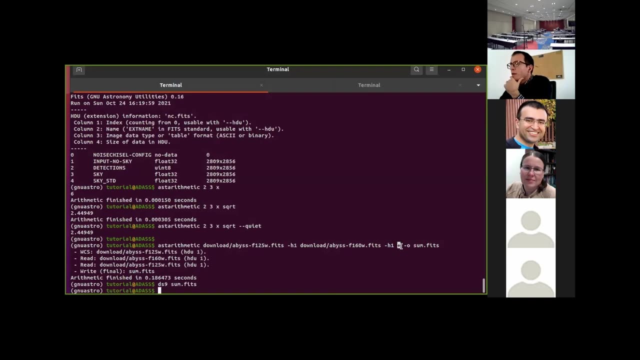 or hundreds of images, and it will be done in parallel, just with one single command line in the terminal. Okay, This is the result. this is the sum of the two different images, and you can use many other operators. There is not only sum or median or something like this, but we have many, many of them. 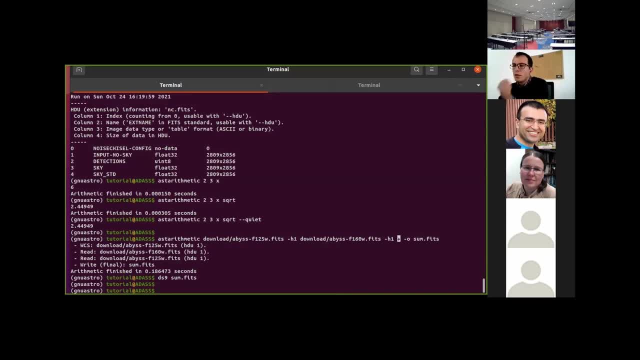 Just to have a look at some of them, you can go to the book, into the website of the Nuastro, to check all of the different options that we have, but you can also have a look without going out of the terminal, So just type here images. 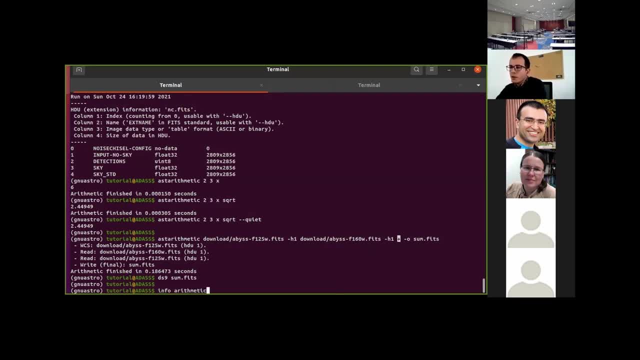 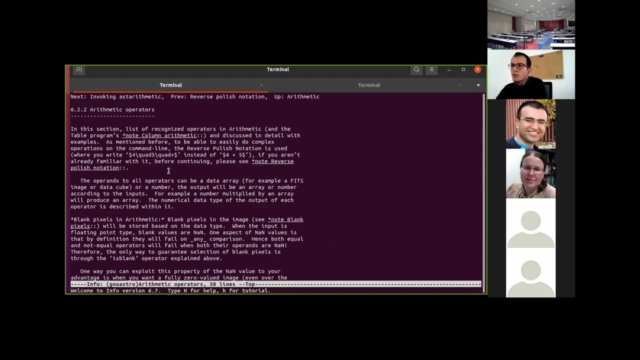 You can see that we have info arithmetic, which is the program that we are using, and then, for example, arithmetic operators- And here you will see a very nice explanation on all of the different things that you have to take into account- and then all of the different operators that we have. 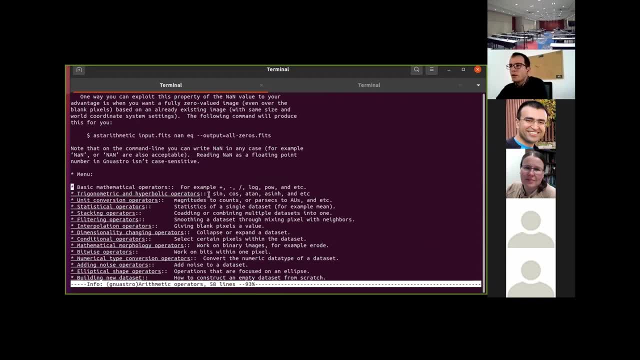 So, for example, we have trigonometric and hyperbolic operators, the statistical units, conversion, Filtering operators, stacking operators and so on. So you have many, many of them. So, for example, if you would like to stack many different images, you could stack all. 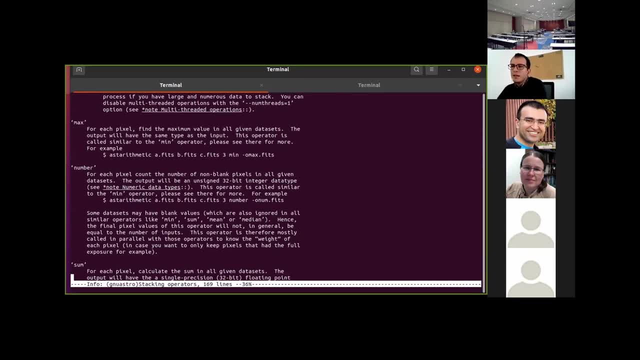 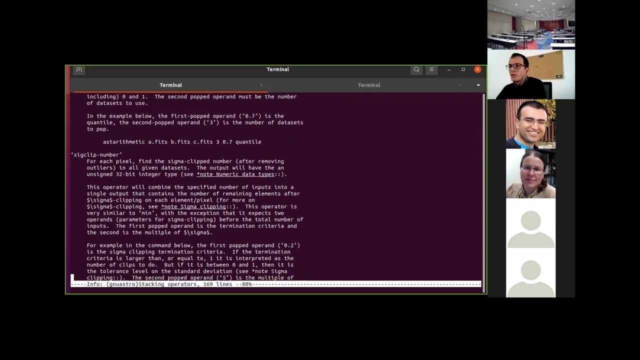 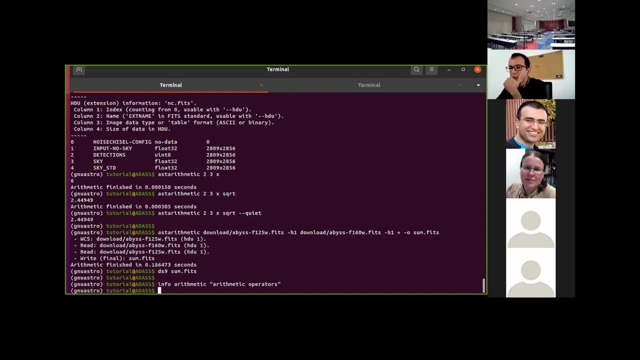 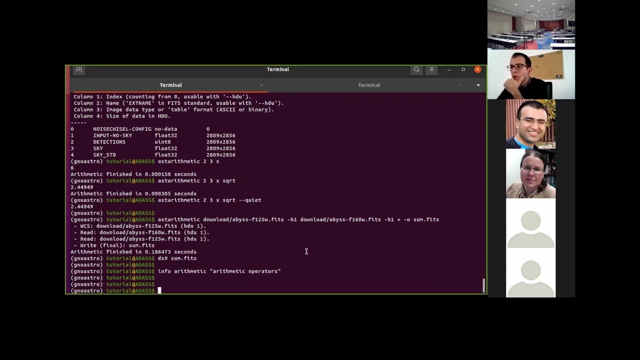 of them using the mean, the median value, sigma clipping, so rejecting outliers values, median standard deviation, and so on. So this is really powerful and you just have to type the command into the terminal. Now let's Let's go and use arithmetic for making something more complicated. 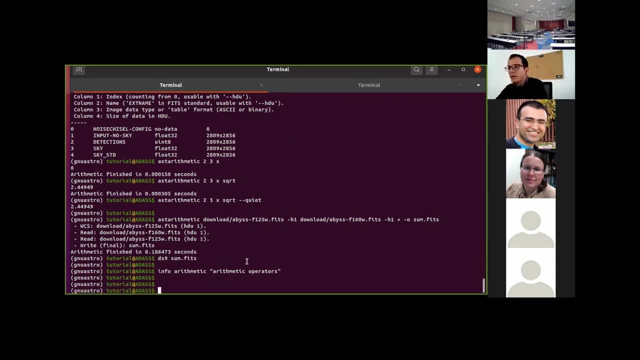 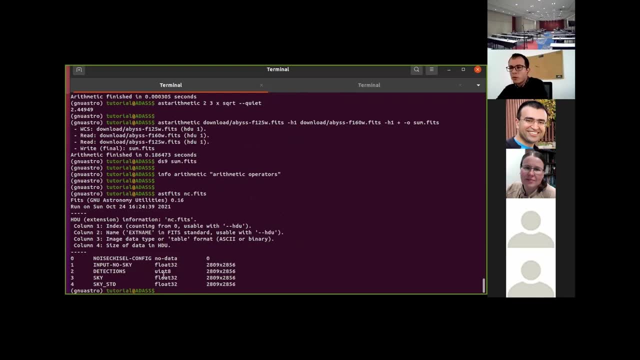 So, for example, we are going to use the detected image of my G cell. So, once again, let's have a look at this, at the different extensions that we have in this output. So you can see, here we have the detected extension. 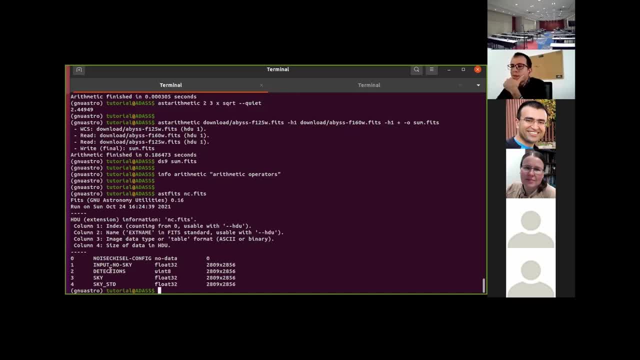 And now the thing that we want to do is to mask all of the pixels in the original image that correspond to the, to the signal in the detected image. Okay, So we can do this with AST arithmetic. So we have to specify the images that we are going to use. So, noise chisel extension number one: this is going. 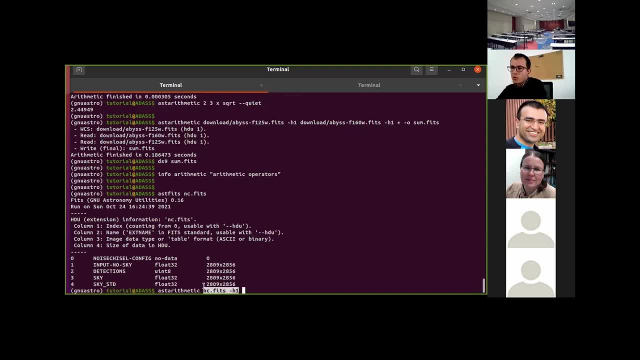 to be the data that we want to mask, and then specify the second extension, which is the mask that we are going to use. Okay, And now the thing, the operation that we want to make. So this: since this is a binary image consisting in one and zeros, we can just say: here we have. 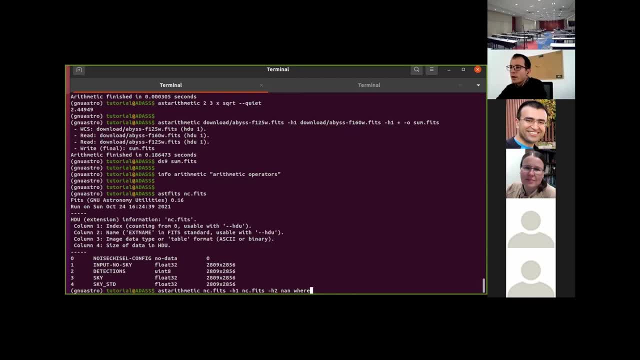 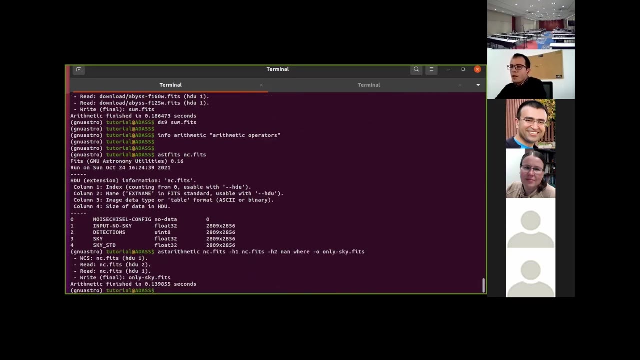 we want not a number of values, where, where the second image is equal to one, Okay, And then we just have to give an output name again. So let's call this only sky, for example. and you are really fast. We have computed the mask of this image. Let's have a look. 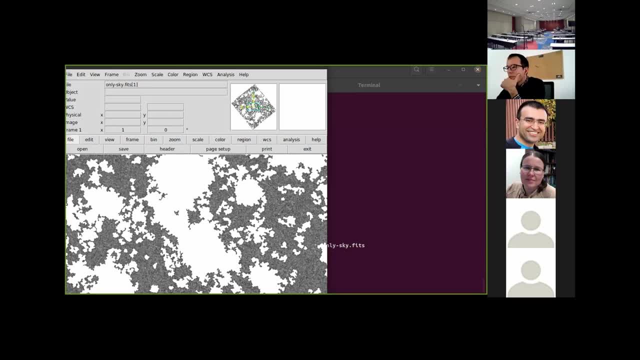 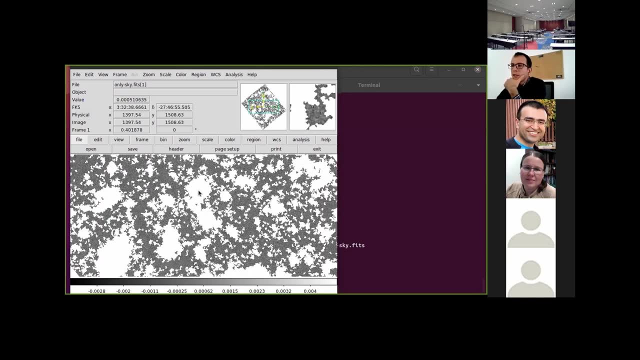 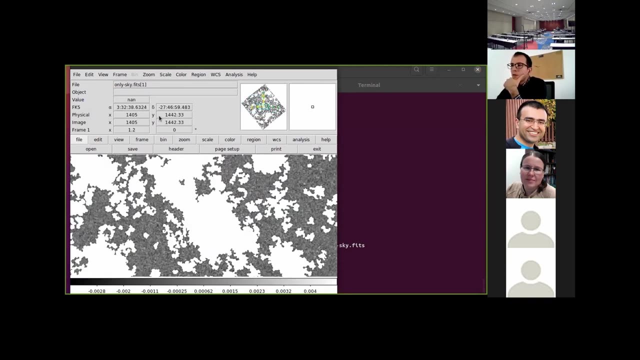 only mask and you will see what's happened. The original image has been so all of the pixels that the word considered to have seen now in the original image has been set to not a number, values, as you can see here, and the rest. So you can see the values here. 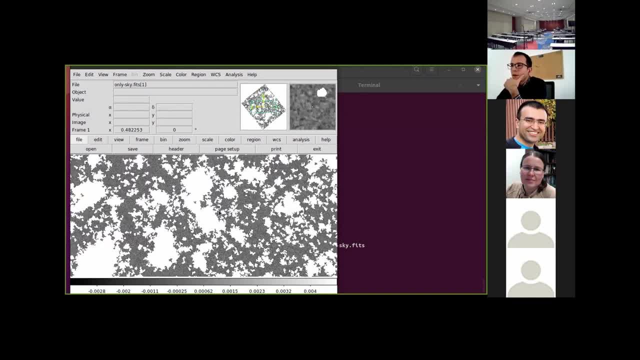 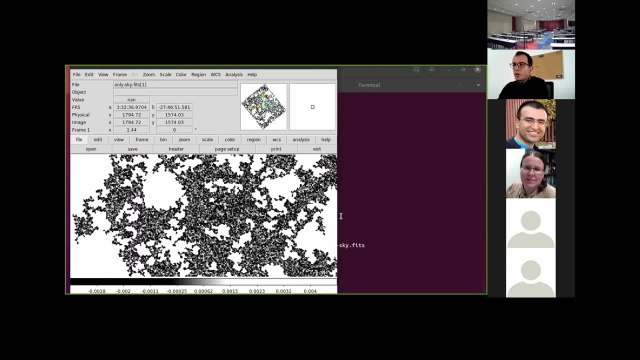 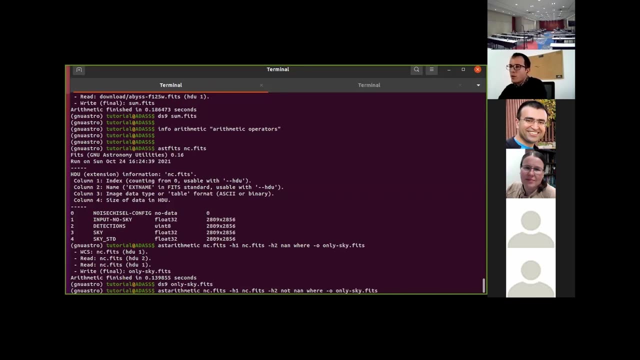 and then the rest of the pixels remains as they were at the very beginning. okay, So that can be done. with arithmetic, We can do exactly the same, but the other way around. So, putting here: not this is another operator, In this case we are going to make the detection. 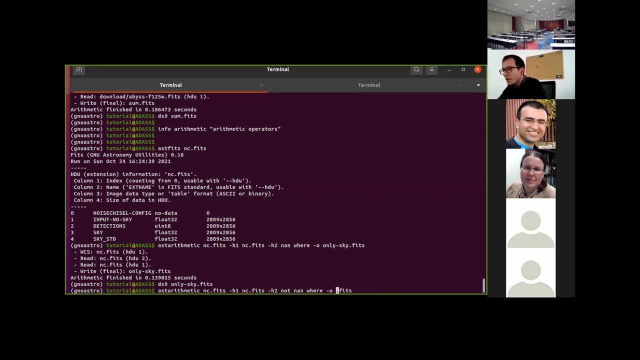 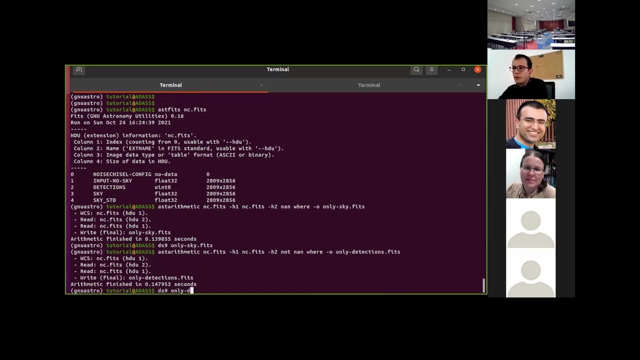 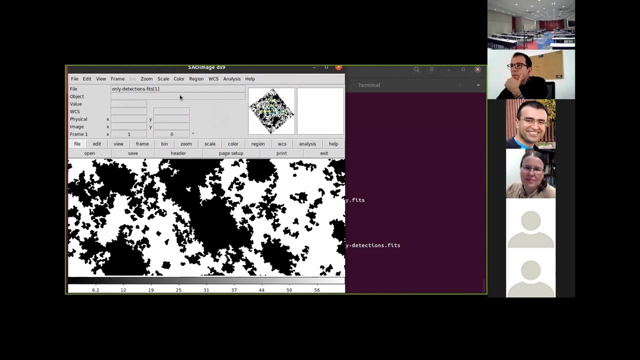 the mask of the sky background and only those pixels that were having signal will remain untapped. So, for example, only detections- and here you just have a look- only detections, And this is, let's say, the complementary operation to the first one. 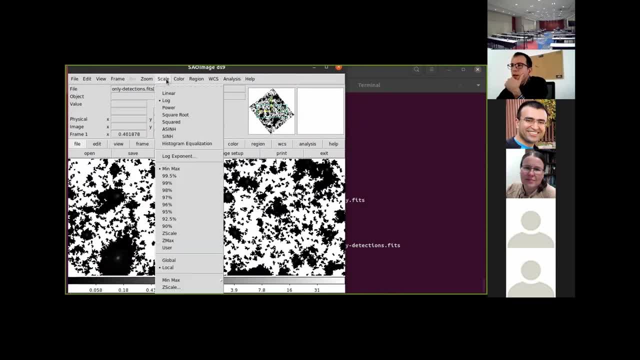 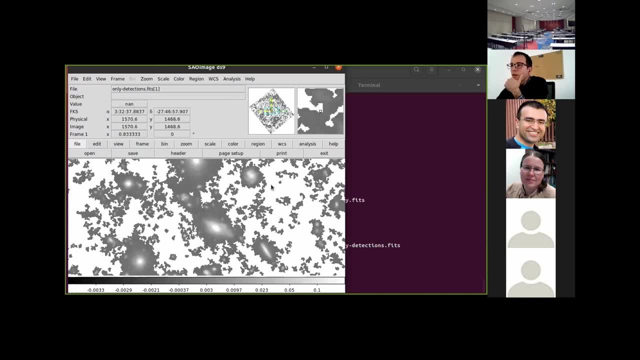 So here you can see that all of the pixels- let's change the scale again- that all of the pixels that correspond to the sky background that were computed by noise chisel. now they become not an under with the operation that we have just specified. 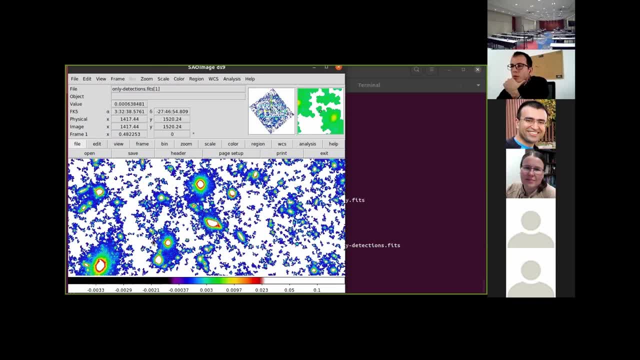 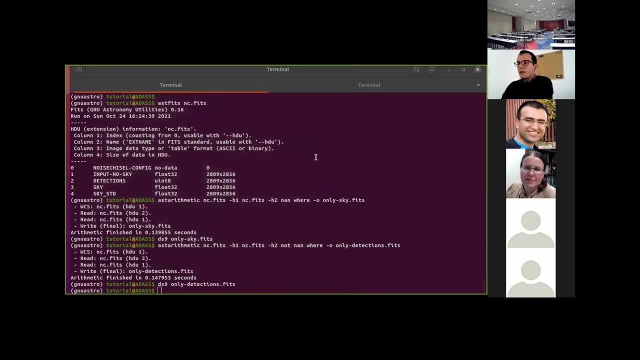 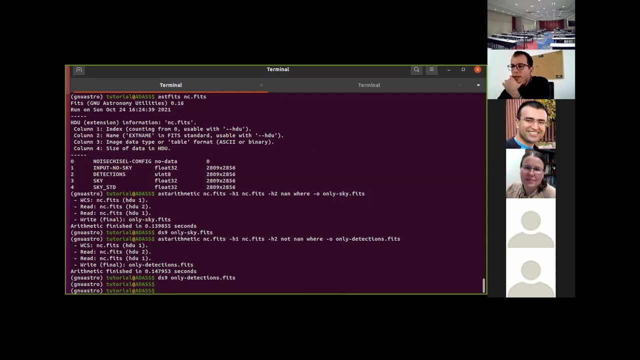 And now, here we have the remaining objects, without not a number of values. okay, So you can make even more complicated things, as you will see later. but now let's move to another program, the next one, which is segment. So once noise chisel has computed the detection of the signal, 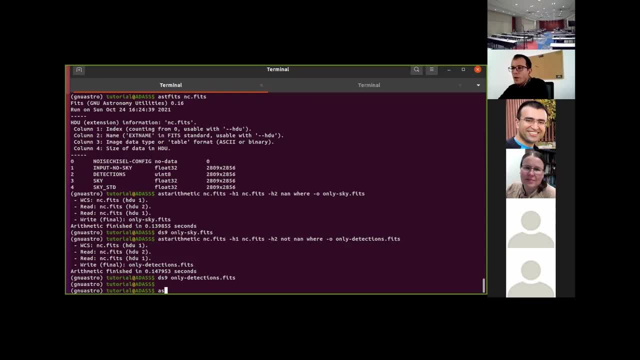 from our astronomical images. we can break that signal into different parts. So we are going to use here AST segment for making the segmentation of the signal. So let's use this, using as an input the output of my chisel. So noise chisel has detected the pixel that has a signal. 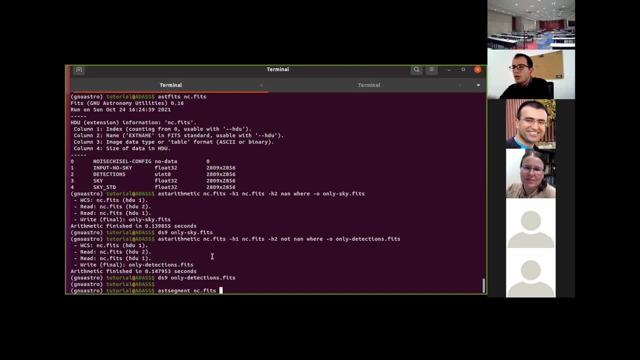 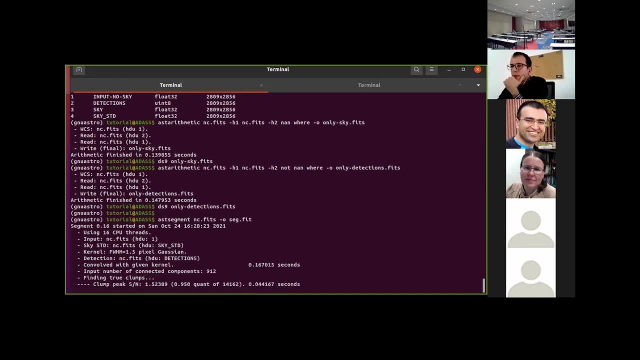 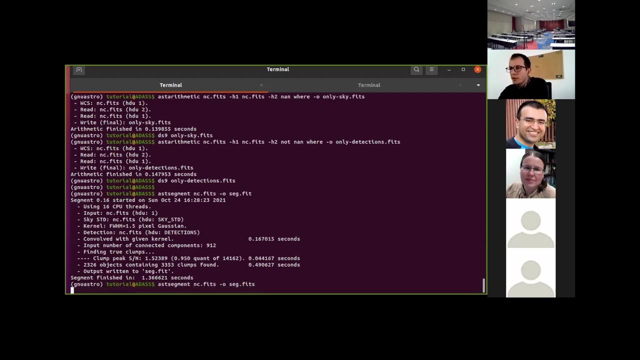 So now we have to specify AST segment noise chisel and that's it. Let's define as an output of the name segmentfits and let it run. So it is also really fast. And let me put fits, just in case something happen. 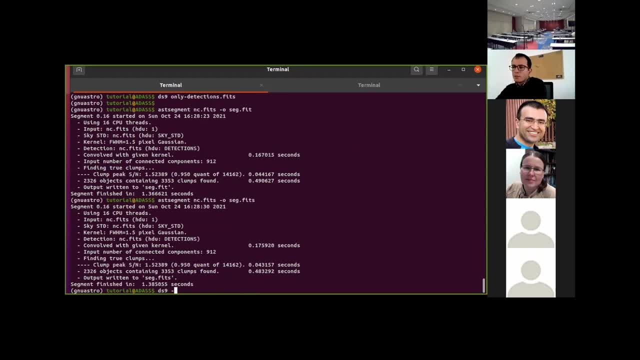 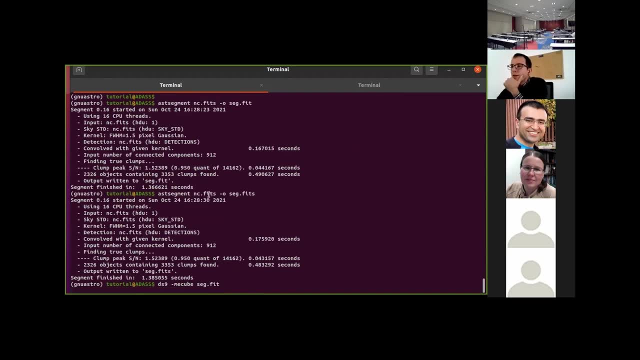 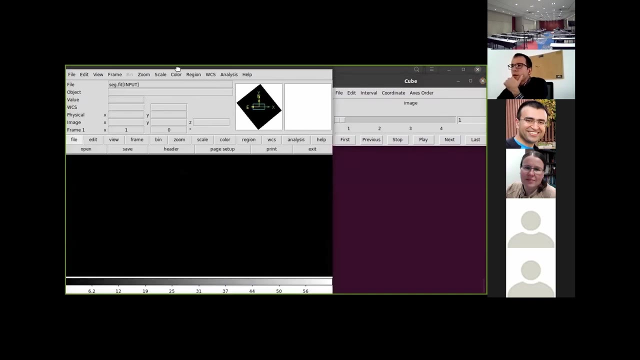 And now we can have a look again with the DS9 multi extension cube and then the segment image, And then you will see that now we have different extensions for the different clamps and objects that segment has computed. So let's change the scale. 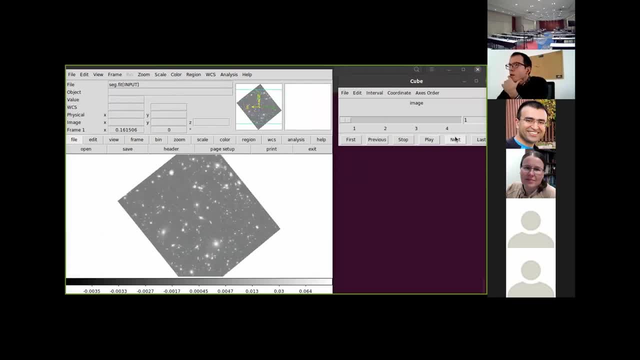 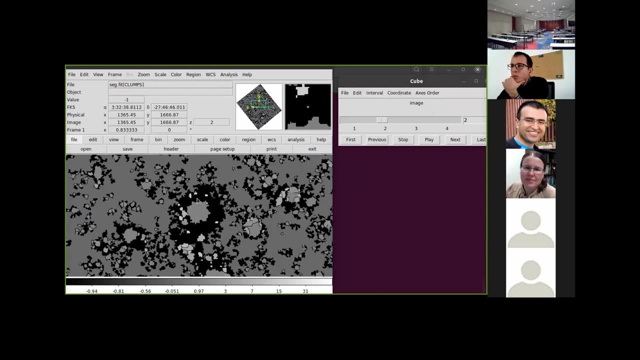 This is the original image, as you can see here. Yeah, and now, if I go to the next extension, you will see that now the signal has been segmented into different clamps. Okay, so this is one object, as you can see here. 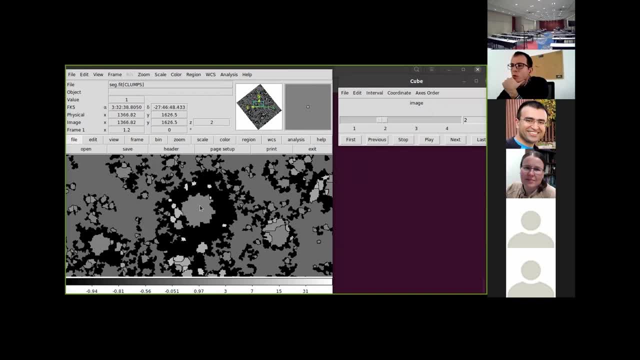 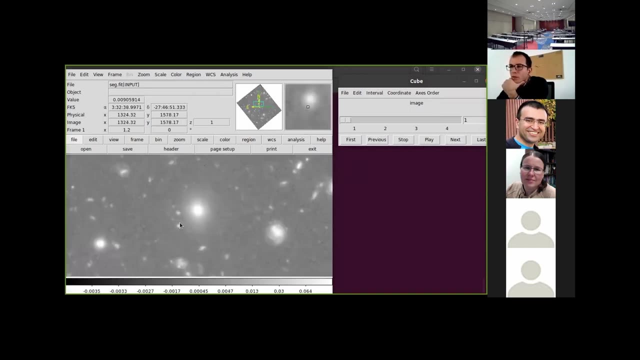 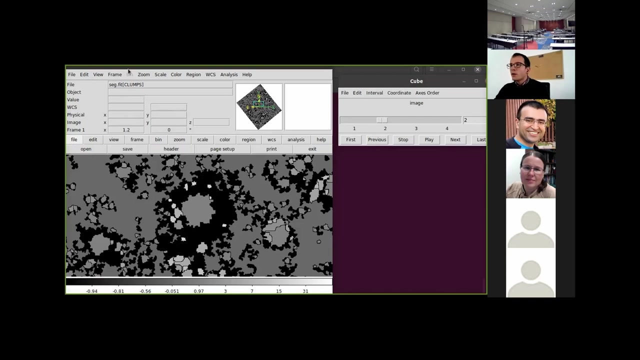 and then it has been broken into different clamps, different group of pixels that correspond to one structures. So if I change in between the original and clamps extension, you will see that all of the structures correspond to the clamps extension. And now we also have another extension. 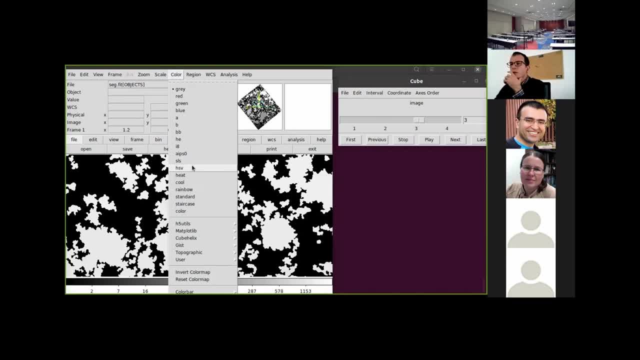 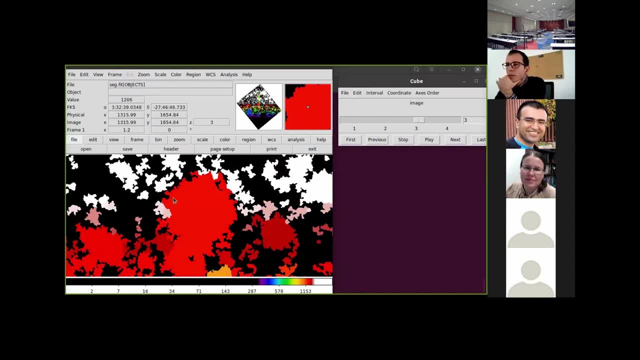 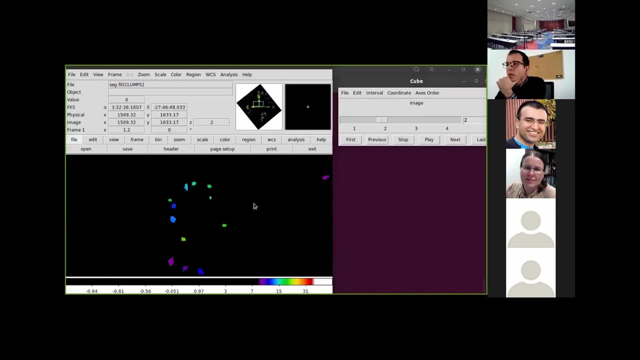 which correspond to the objects. So let me change the color bar. As you can see here, each different group of clams belong to one given object. So this is one particular object and within this object we have different clams, as you can see here. okay, 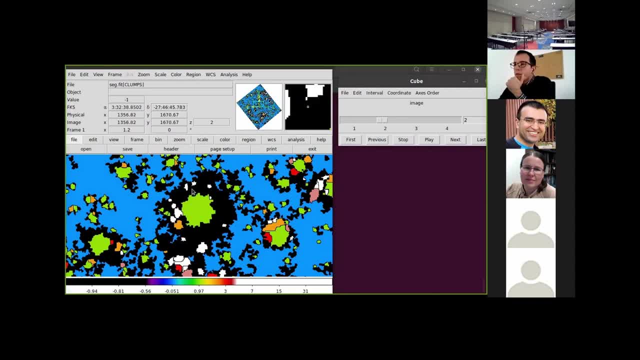 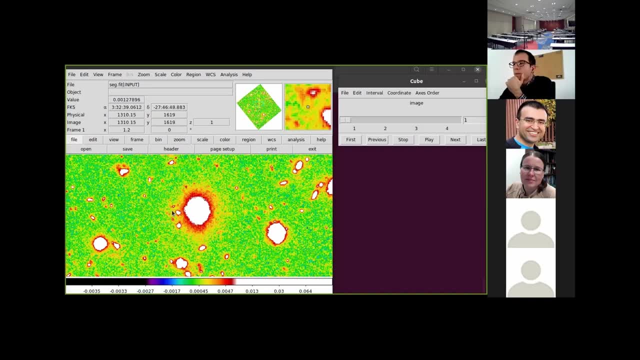 So now let's do the next experiment. Imagine, for example, that you would like to study the outer part of this galaxy- okay. So once you are able to detect the object far away, okay, using noise chisel. and now that you have break, 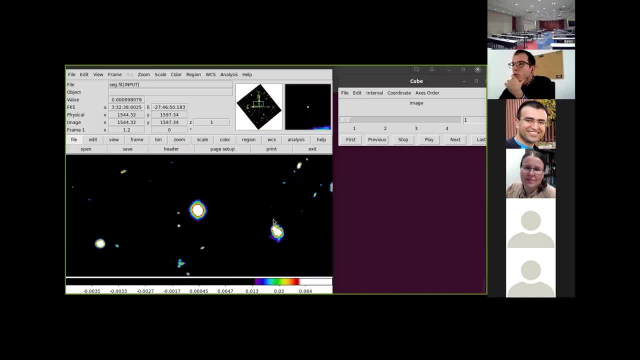 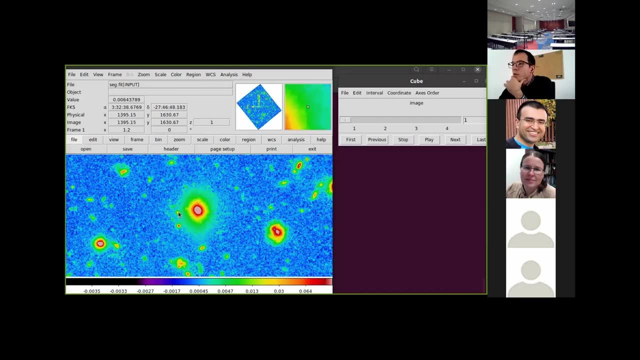 this into different objects, from this one to this one, and then also you are able to segment the different parts of the same object into different clams. okay, Imagine that you would like to study the outer part of the galaxy, the low surface brightness part of this galaxy. 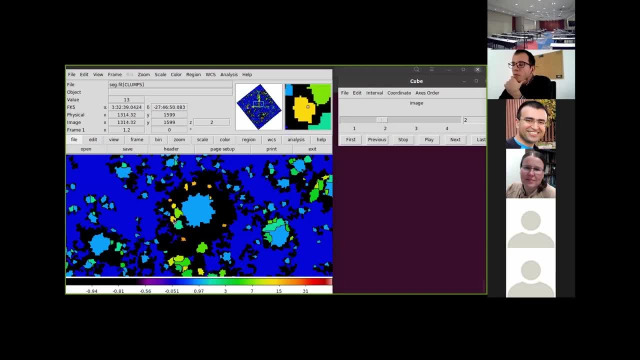 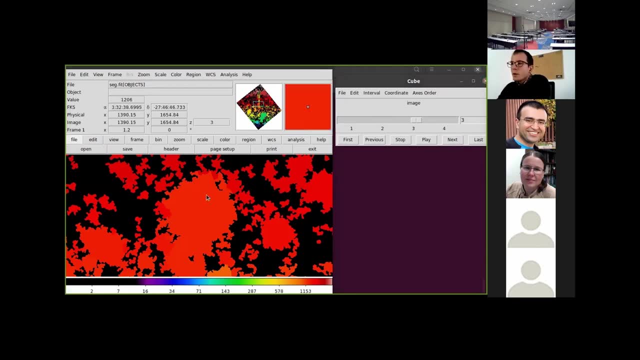 So you could make a combination of this mass and the object mass And for that particular experiment, remember this value. So the value that you can see here for this object, 1,206,. and now let's use arithmetic for make more complicated things. 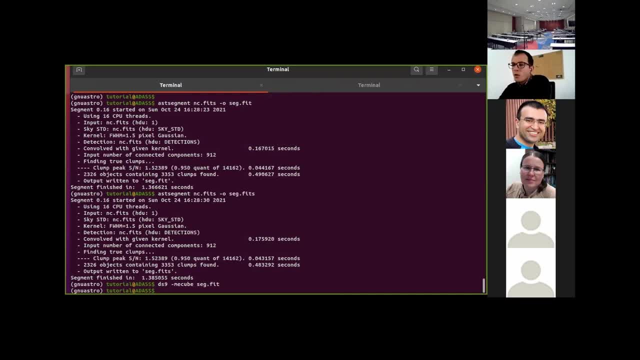 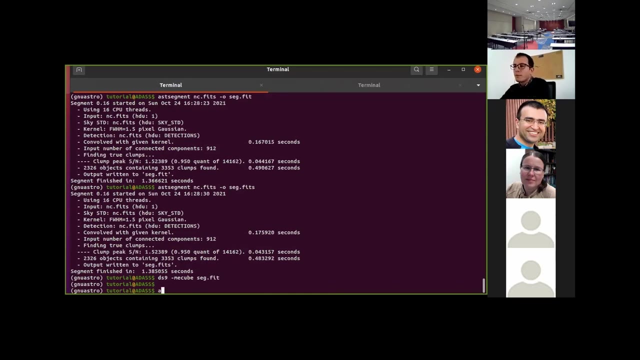 So we are going to mask all of the objects and all of the clams corresponding to this object while we study the outer part of this galaxy. So let's do it step-by-step Instead. remember that, just in case you have any problem or any doubt. 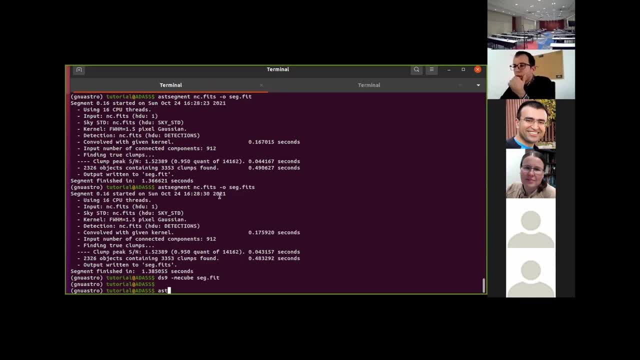 Mohamed Akhlaqi is in the Discord channel So he can solve any kind of problem you may have. So let's use again as the arithmetic. Okay, And now let's use a very nice feature of arithmetic. So let's specify: 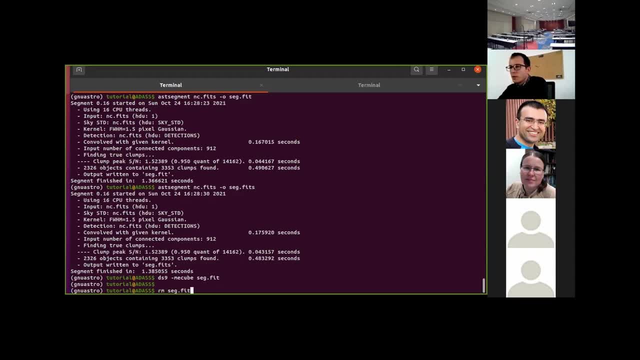 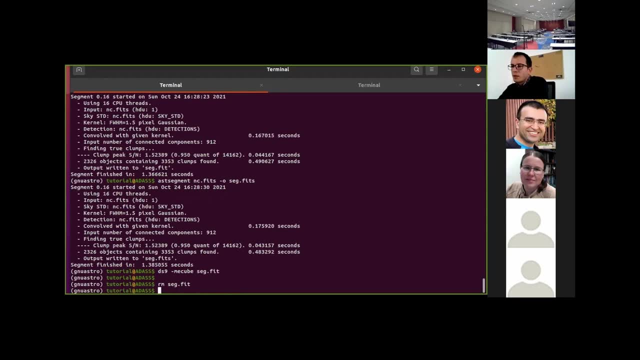 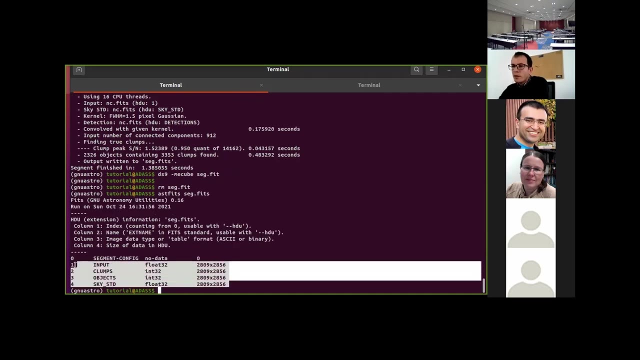 Let me remove this one. Okay, Arithmetic segment. Let me, before that, show the different extension, Just to have it in mind. So here we have the different extension that we have, And now let's go with arithmetic. So AST arithmetic, the segmentation extension number one. 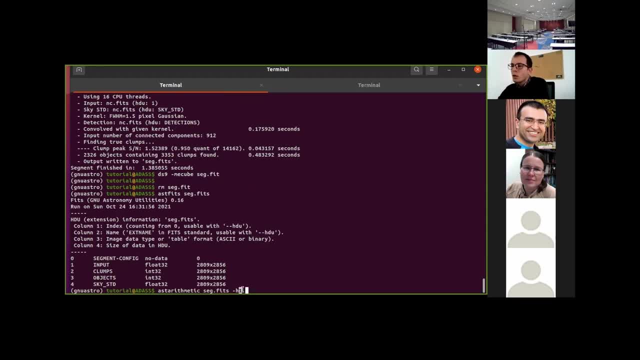 This is the input image And we are going to call this data set as data. So this is a feature here that we can use, which is set Dash data. Okay, So now inside arithmetic data is the extension number one data. Okay, 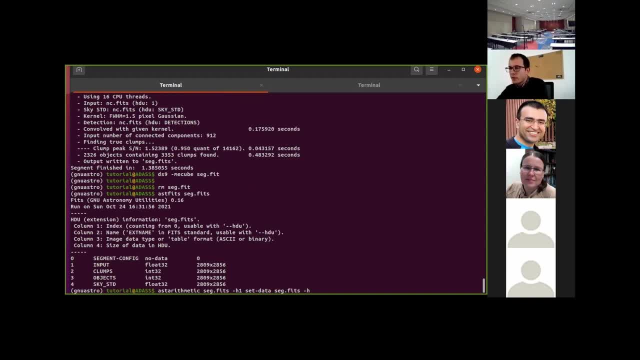 So let's do exactly the same, but for the extension number two, which are the clamps, let's call this clamps, Okay, And do exactly the same with extension number three, which is, uh, which correspond to the objects. 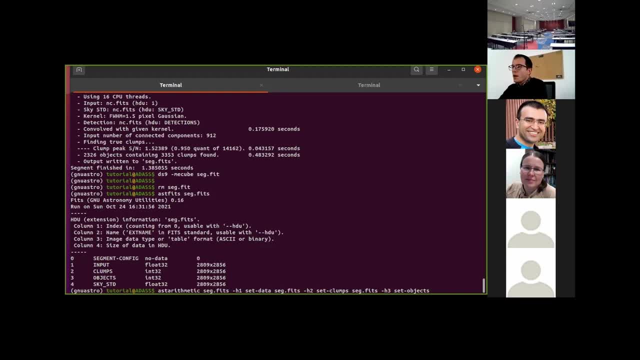 So set. And now let's do the operation. We want to multiply the extension number one, which is sorry, the extension number two, which are the clamps, by the extension number three, which are the objects. So you just have to type here: clamps, objects and then X. 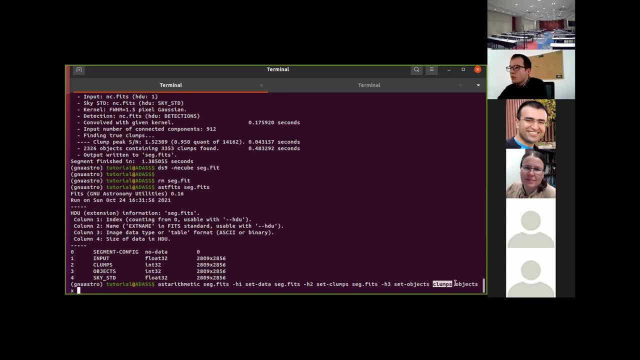 Remember the reverse policy notation: you have to put before the operands And then at the end the operators. Now we Want to call this for example: combine okay. So set dash, combine Okay, So this is the in combine. we are keeping the result of multiplying these two. 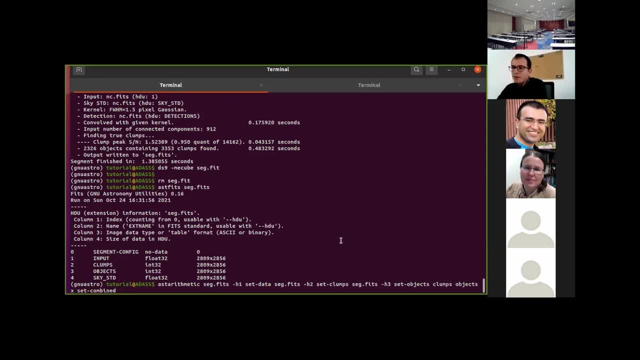 extensions. and now let's uh mask on the original image those pixels that are not equal to a given value, which correspond to the, to the value of the object that they say before So data, We are going To use the combined mask. 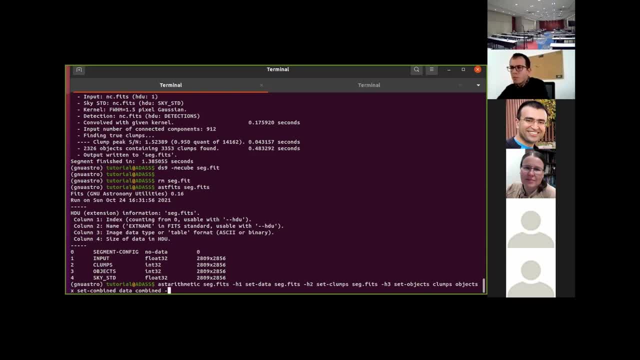 Okay, And now we say minus, minus, uh 1,206,, which is the value that we don't want to mask. So we say not equal, and then put nan values where this condition is: uh is true, Okay, And then we just have to give them a good output: uh names, for example. 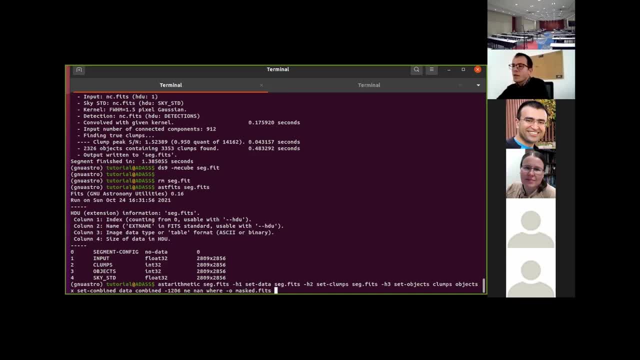 And then we just have to give them a good output- uh names, for example. And then we just have to give them a good output- uh names, for example. So we say mask That fits And then execute the data line. 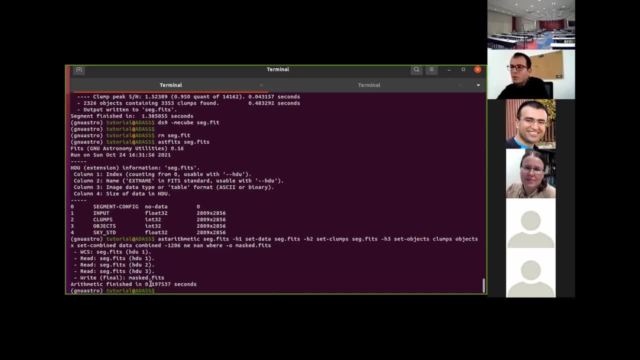 And you will see that really fast. So this is almost zero point. uh, 0.7, two seconds. It has compute all of these operation and it has given to you the output image. So let's have a look. um, using DS nine. 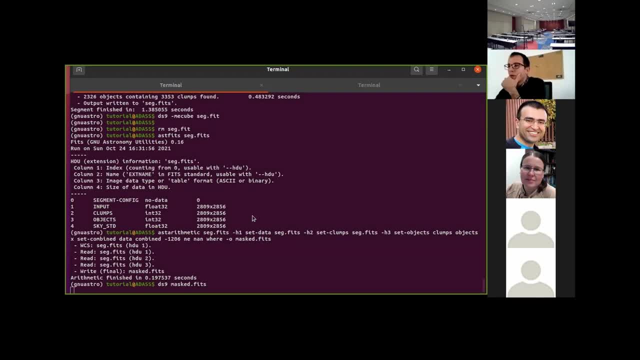 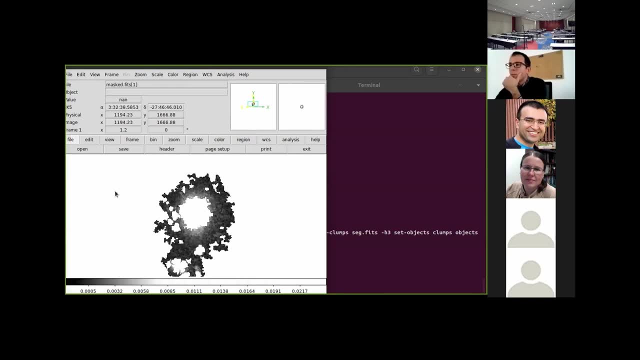 So mask and you will see what is the result of this operation. So, as you can see here, we have used, Uh, the different mask, the clamps on the object in order to only have the very low surface brightness features around this kind of clamps for this particular objects. 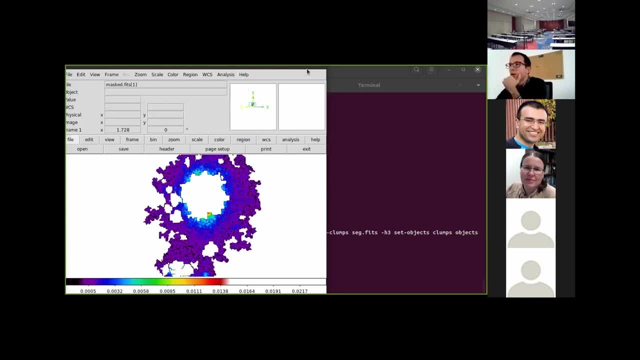 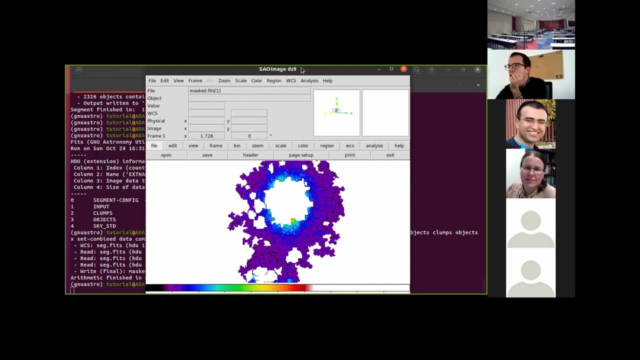 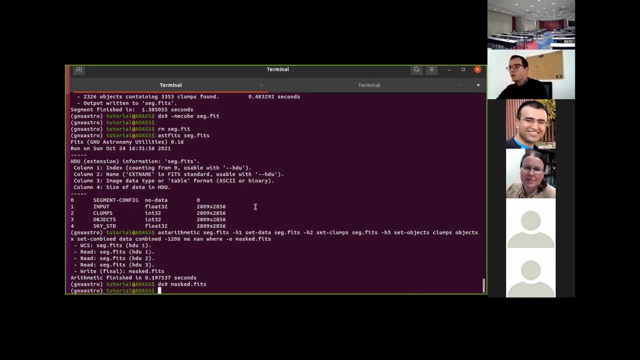 And all of these have been done in one single line, into the common line, So you can let your in ledger. This is just to let you know that you can make many, many, many powerful things. Yes, Using this, uh, this set of. 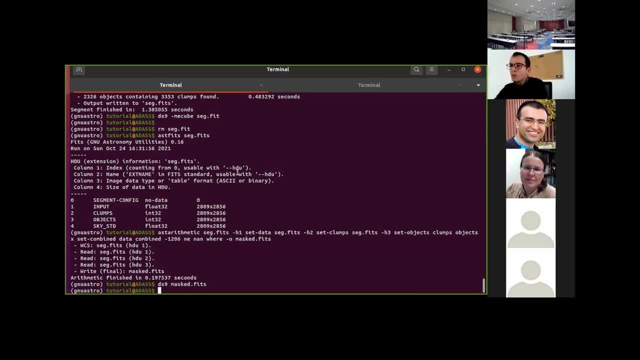 Programs from the new Astro. Now that we know how to use arithmetic and that we can do many things, let's move to the, to another program, which is AST- make a catalog. AST- make a catalog. This program was presented in others, 2016, in three step, by Muhammad. 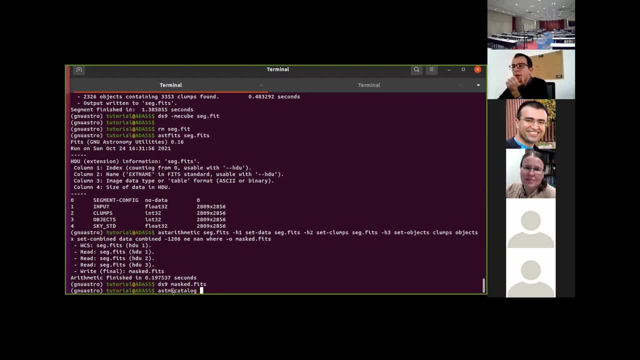 And now I am going to explain how to use that program, this program for obtaining Astronomical catalogs, astronomical tables, uh, from our images. So once we have constructed uh, once we have uh, detected the signal and we have, 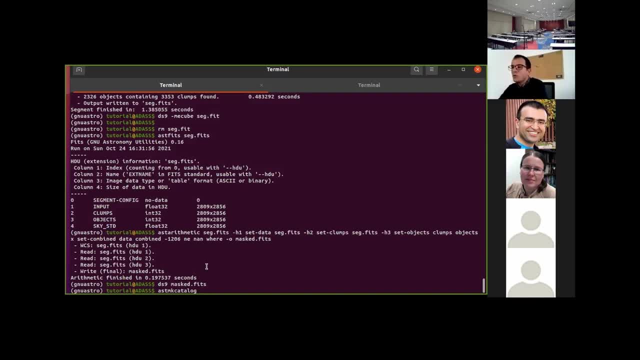 break the signal into different objects, we are able to make measurements over that, uh that images. So for AST make catalog, you just have to specify the segmentation image that gains from the program AST segment And now Just specify the different measurements that you want to obtain for your pattern. 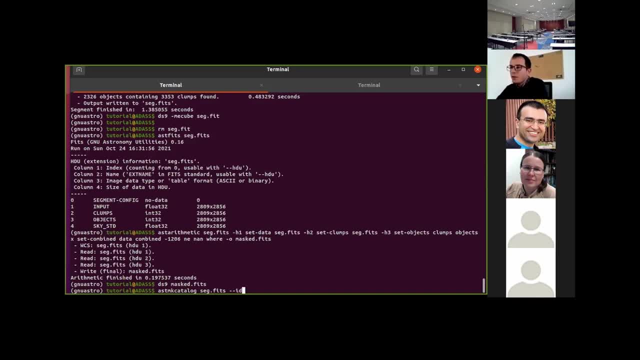 So for example, let's specify here the labels, the ideas of the objects, the right ascension, the declination, so the coordinates. let's put also the magnitude, the signal to noise, signal to noise, the axis ratio. 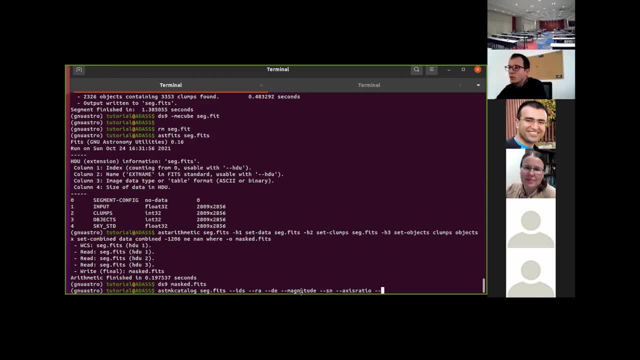 Okay, And then, in order to be able to have a Okay, And then in order to be able to have a Good magnitude values, we have to specify a zero point. So, for example, zero point equal to for this particular image, it is 25, 94.. 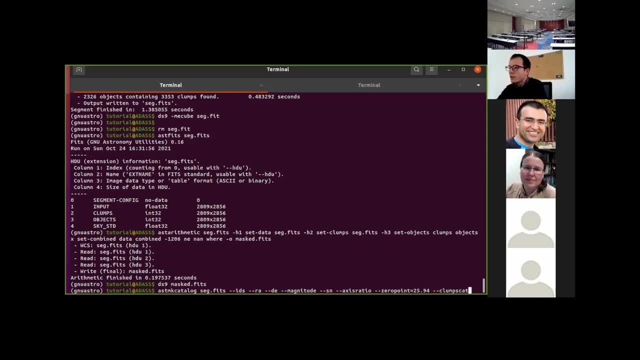 And then let's also ask for a plan that not only for an object cover, but also for a clamscape. Okay, And now let's give a good uh output names, for example catalog, and that's it really fast. 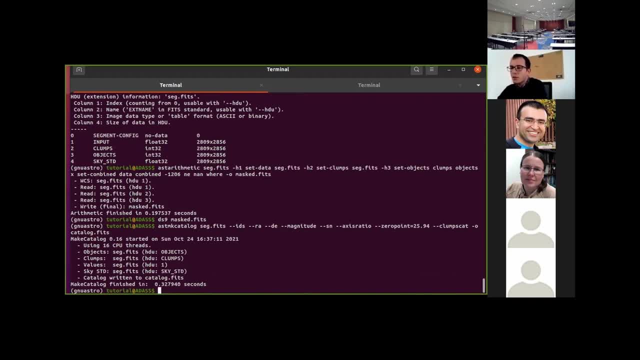 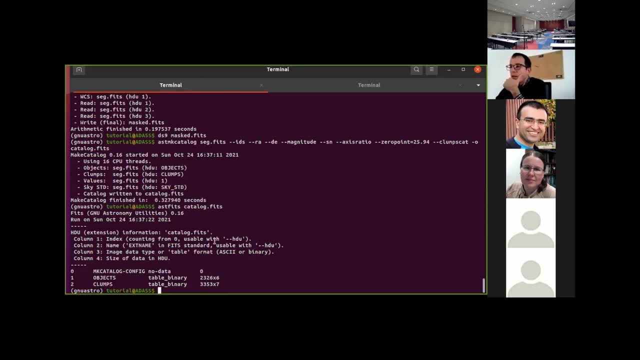 Again, It has compute the catalog and now we can have a look with AST feeds and the catalog that we are obtaining And, as you can see here inside of this file, the catalog that we have previously obtained. we have two different catalogs: one for the objects and the other one for clamps. 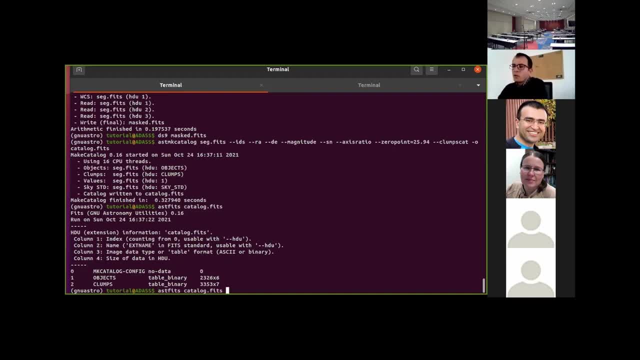 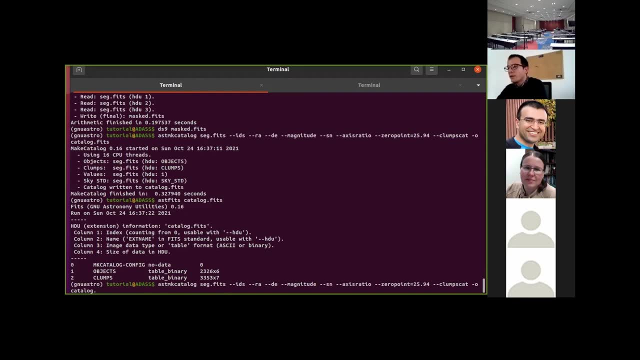 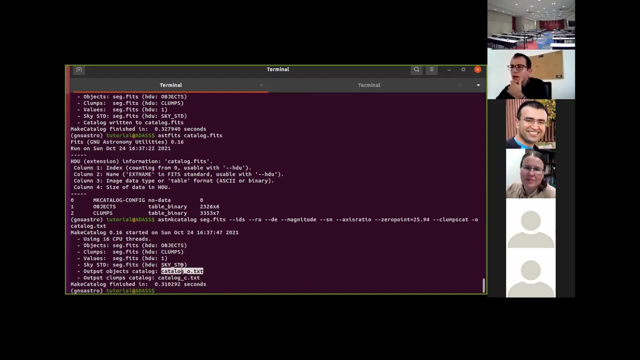 Okay, Now, for example, if you would like to obtain the catalog, the catalogs in plain text format, you just have to specify Here the extension TXT and in that case, uh, it will compute two different catalogs, so two different files, one for 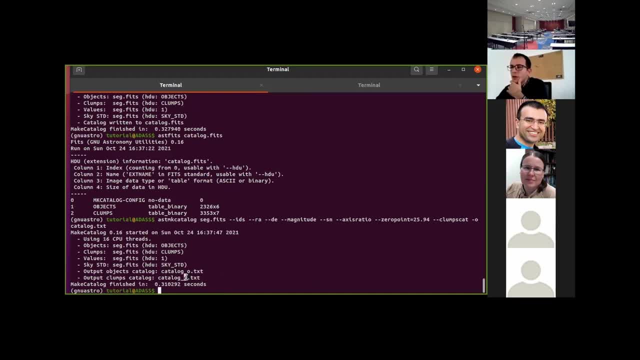 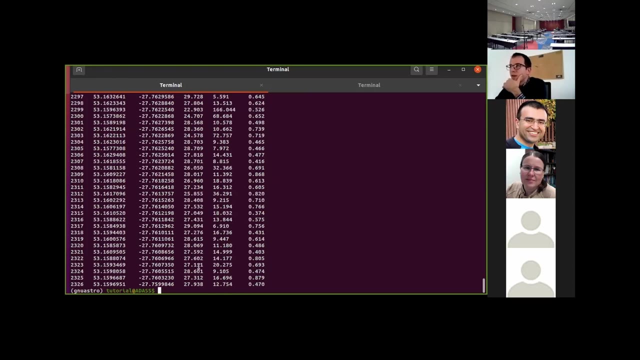 objects, as you can see here, and the other one for, uh, for plants. Now we can have a look at the, at the catalogs itself catalog, for example, for the objects, And you will see that here we have different columns that are the ones that we have requested. 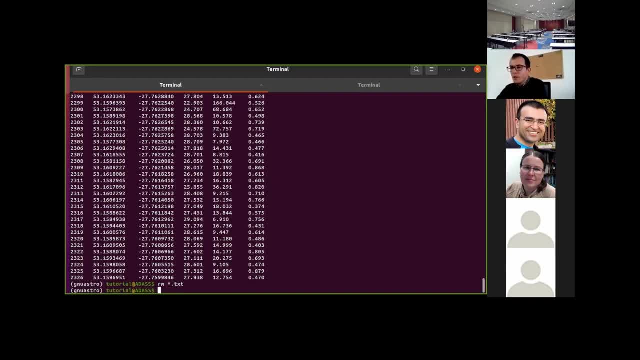 So let's remove uh, the The TXT files, because, uh, we are going to work with the, with the feeds, uh, with the feeds files. So, now that we have constructed uh one catalog, we are able to go to the next uh program, which is AST table. AST table. 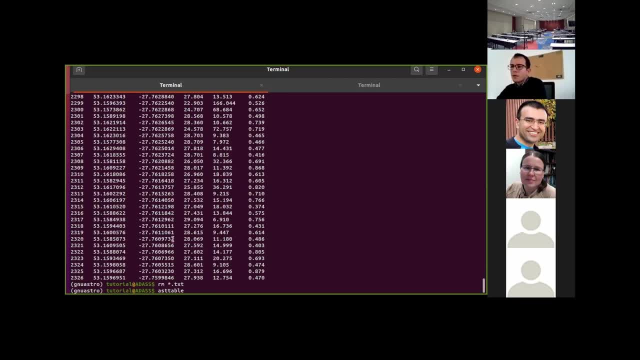 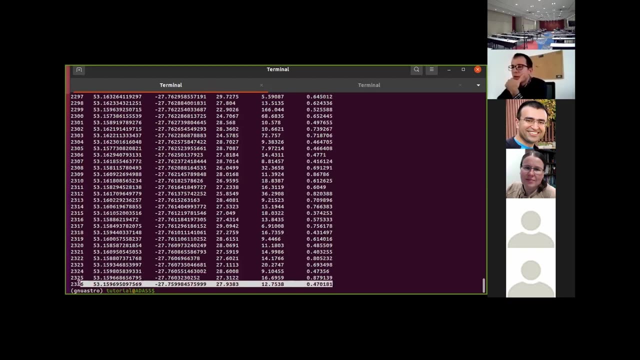 And this program is aiming to manipulate in astronomical data set, astronomical tables. So so here you just have to type AST table And then it will. it will print on the command line the catalog, the measurement, So the, actually the data of the catalog. 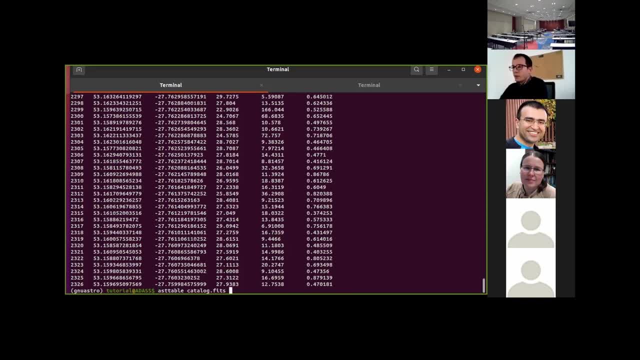 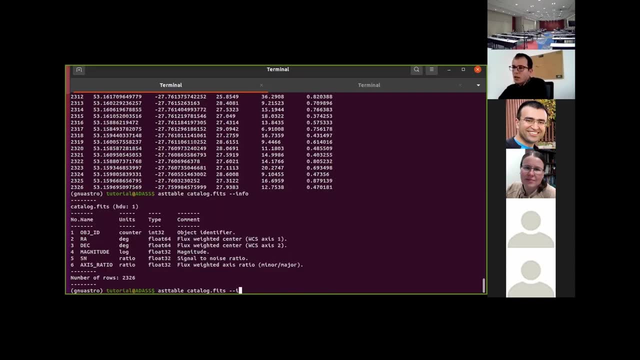 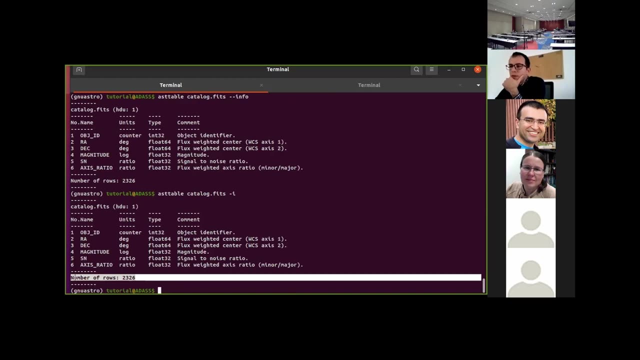 So if you want to obtain, for example, only some data of this catalog, the metadata, you just have to specify here dash dash, info or dash dash, sorry, dash- I in the short option And it is going to print on the command line: how many different objects do you have in your catalog? 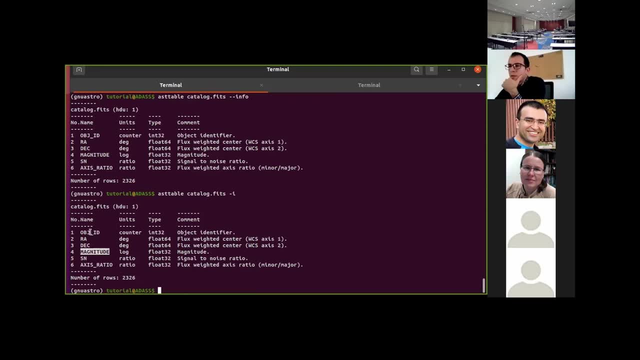 Okay, And the different columns measurements that you obtain with this particular catalog. Now imagine that you have a very huge, very large catalog and you only want to to use some of the columns, So you can do that with the option. column equal to, for example, write ascension. 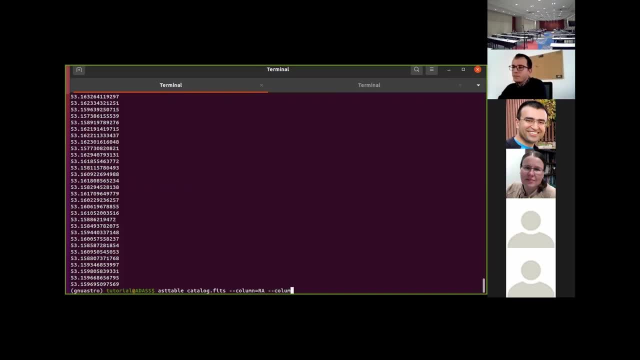 You can specify, of course, another one column in equal deck to obtain the Write ascension and declination. And actually you can do this much shorter, just putting a comma in between the different names of the columns that you want to obtain, and even shorter with the option that dash C and the name of the columns. 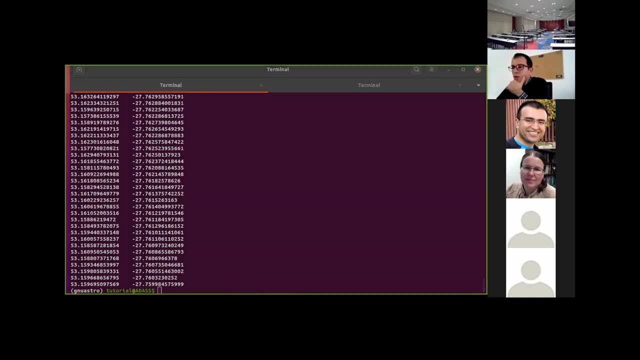 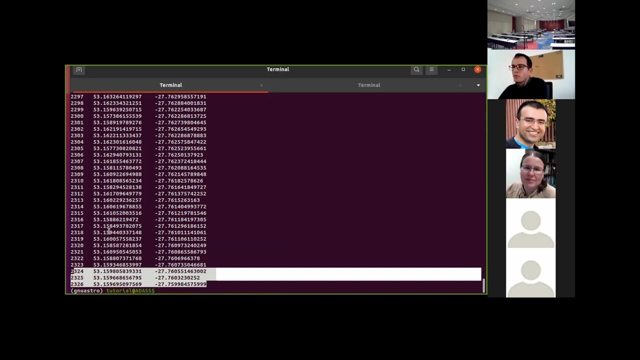 Okay, Of course you can also use the number of the columns, So the position of the column system instead of the name. So column number one, number Two and number three, and it is going to print on the comma line the columns that you have specified. 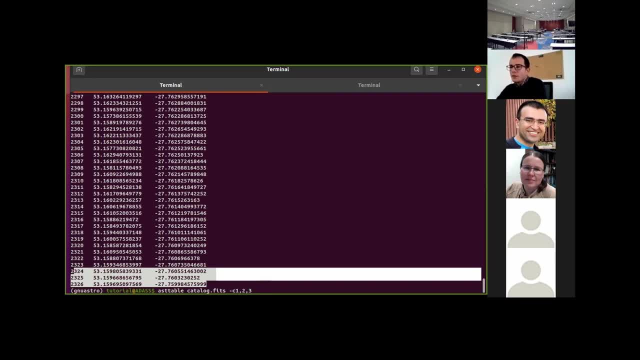 Okay. And now imagine, for example, that you want to keep these columns as another table, just because the original one was very large. So you just have to specify here the output name and say, for example, super catalog. that fits Okay. 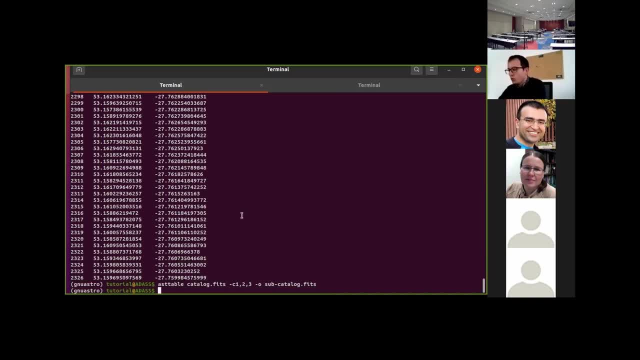 And it is going to save all of these into you, Into a new data. So I used the table super catalog just to have a look and you will see that now this is the result of the of the previous operation. If you want to, for example, have a look at the some objects that are within a given range of magnitude, 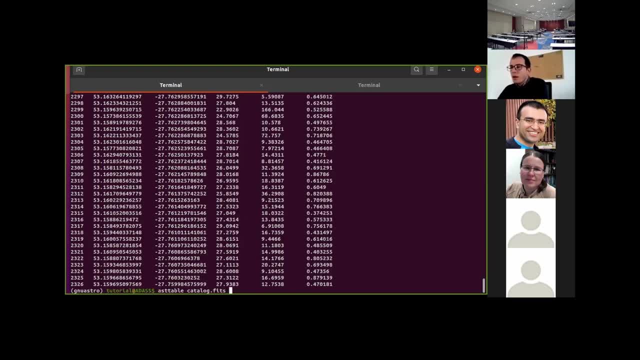 So, for example, let's print everything here And now imagine, for example, that you only want To have in your sample only the objects that are within a given range of magnitude. So you can. you can do that by specifying here with the option range. So range equal to the column name, So magnitude and then comma. the first values, for example 26.99,, and then the other value, the, the, the other extreme of the range, So 27.0.. And it is going to print on the common line: 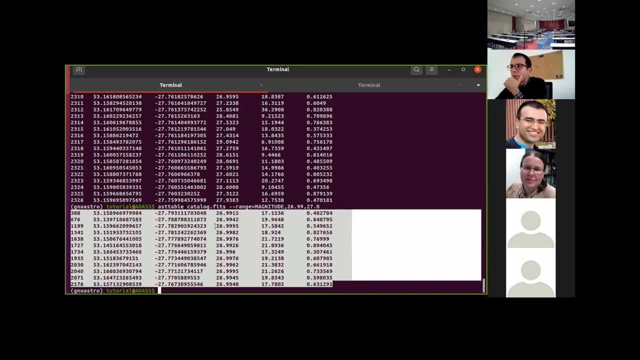 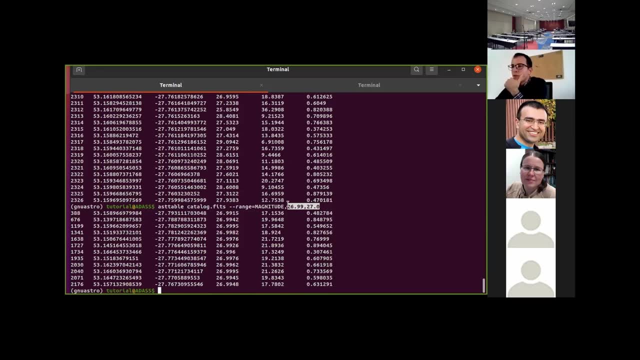 Only do those object that uh, that uh, that uh for, for the condition that the this is true in that, uh, in this range of magnitude. again, you can do exactly the same, but adding another condition. 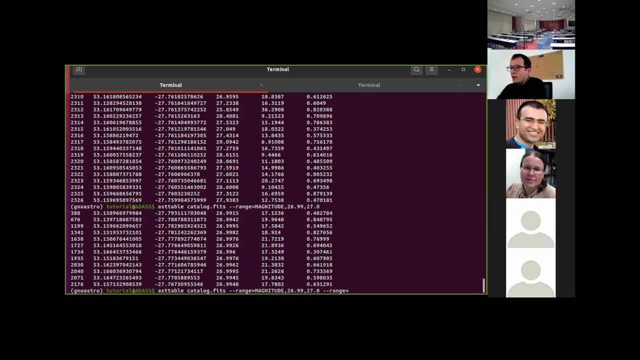 So, for example, I want all of the objects that are in the range of axis ratio in between, for example 0.0. Point Six and one, and then it is going to print on the comma line: only does object that uh, that uh. that are true for these two different conditions. 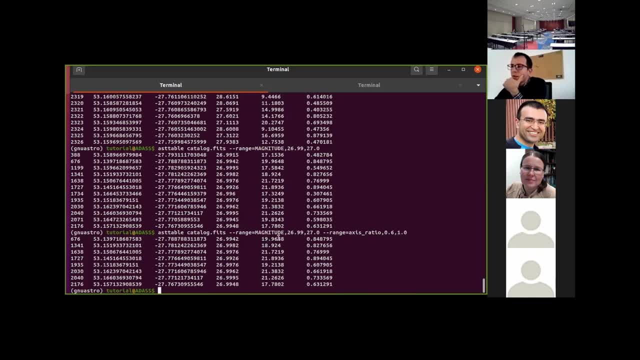 And now imagine, for example, that you would like to to sort this sample by the signal to noise ratio column. So you you just have to use the option dash, dash, sort, and then the column name, so signal to noise, and it is going to print in all. 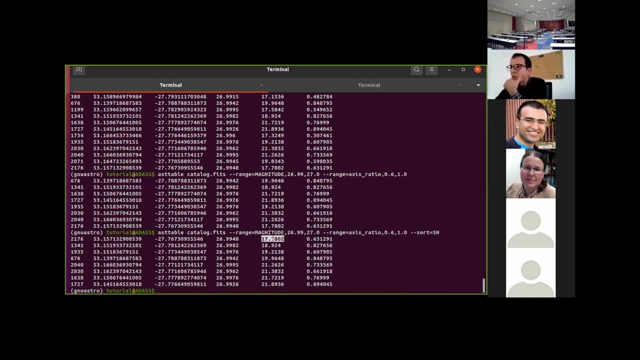 There. So this is the very first one. So the smaller signal to noise ratio value and this is the largest one, that of course uh falls within these two different range of magnitude and axis ratio. If, uh, for example, you will like to count the number of objects that you have in this uh, in this sample, you just have to die this to the program WC and count the number of lines. 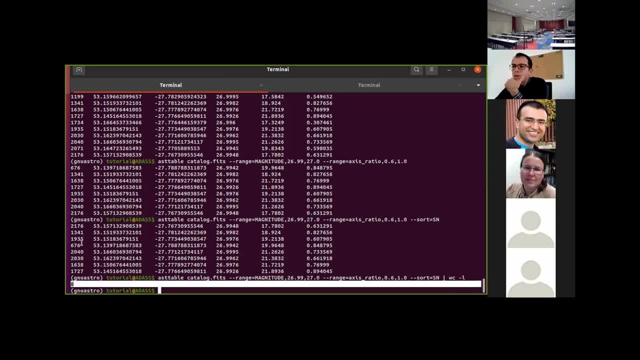 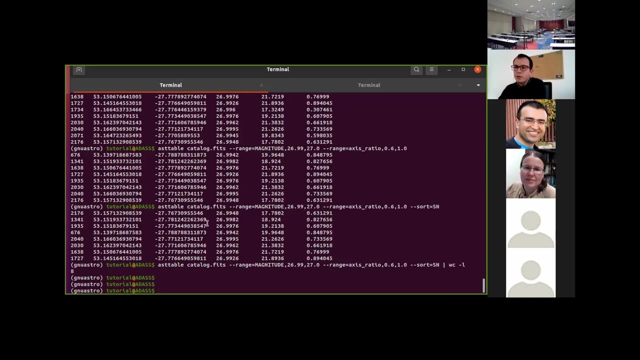 So, in total, we have eight uh different objects. Uh, in total we have eight different objects. Uh, in total, we have eight different objects Within our catalog. that uh, with this range of uh, with this criteria, and now moving to into another feature, which is the arithmetic column with uh- AST table. 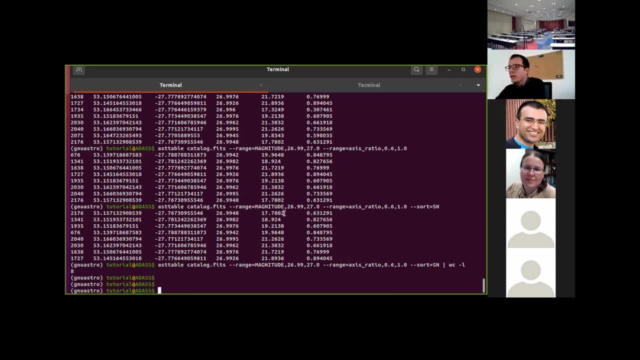 So, once we are able to sort, to manipulate, to filter our, our data, imagine, for example, that we would like to obtain the magnitude column, but in milli magnitude. So we we want to to transfer the magnitude column to milli magnitude. 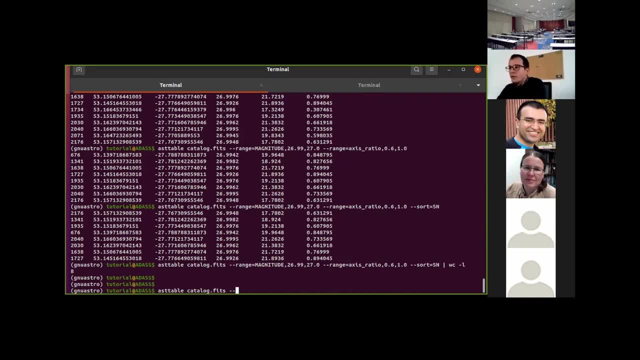 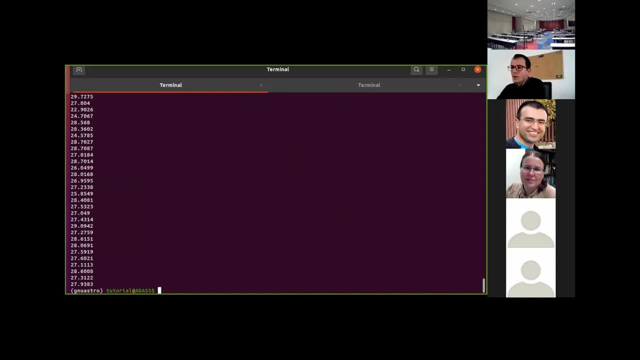 So we we want to to transfer the magnitude column to milli magnitude. Okay, So we can do this directly with uh AST table. So let's put, for example, the column here, magnitude. Okay, This is going to print the original magnitude column and now we want to operate this column. 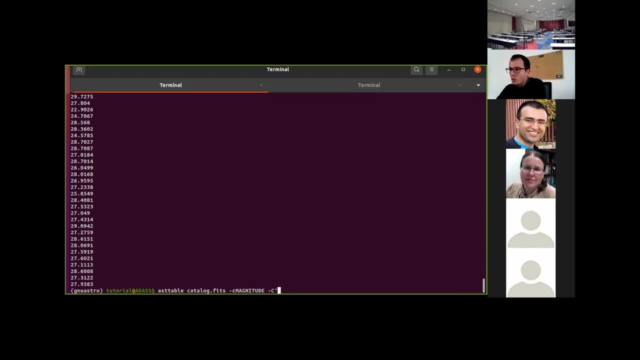 So we just have to type here C and then quotes, sorry, in small, single quotes. And now we are going to specify here, Arif, because we want to make some operations, and then, And then we want to multiply this magnitude column by 0.001, and then the operator, and it is going to give to you, it is going to give to you the, the, the results. 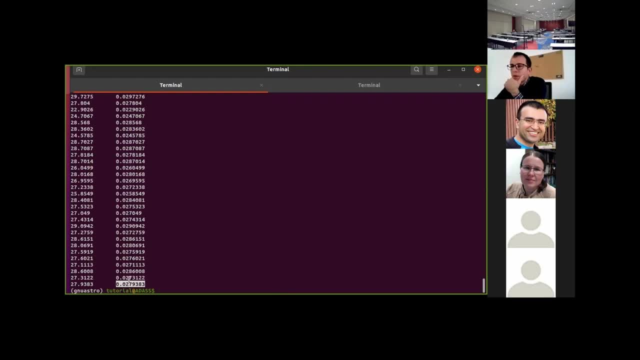 So once we have uh, multiply the original column by 0.001, of course this is very simple. We have again many different operators, So let's make another one. Okay, One more complicated. So imagine, for example, that here we want to transform the right ascension and the declination of this catalog into pixels. position of one particular inch. 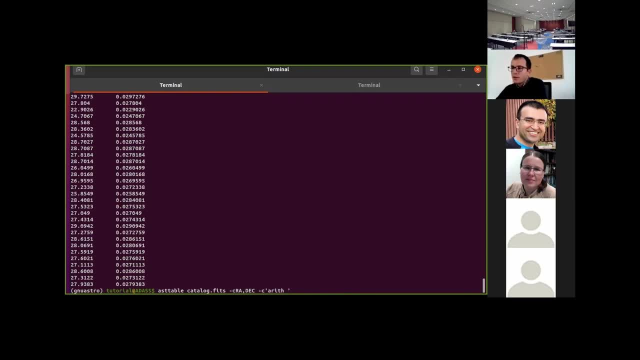 Okay, So we can just specify here this operation. We want to make the following operation right: Ascension declination. And now we want we are going to transform the WCS to image coordinate. Okay, If you just press enter here it is going to. sorry, I'm missing here EMG, and it is going to complain about not having astrometric information. 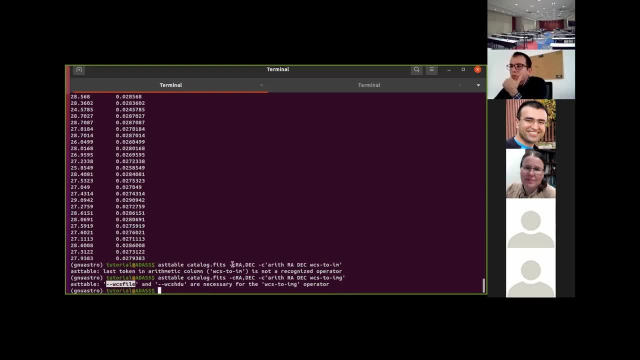 And this is because you are trying to transform the right ascension and declination. but, of course, a EST table with this operator needs some WCS information, for which we are going to give, with this option, WCS information. Okay, So now we are going to use the WCS file, the original image. 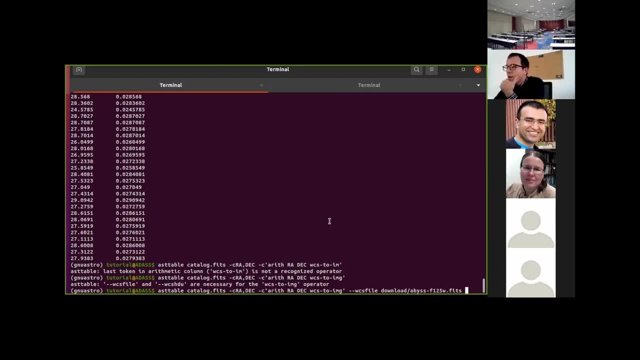 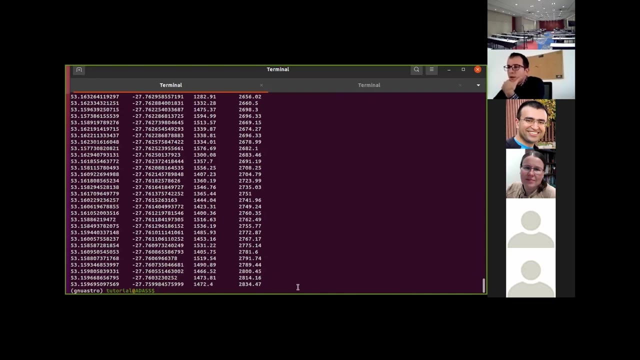 So, for example, download and this filter. Okay, So now it is going to use the astrometric information within this image to transform the position on the sky to pixels position. So press enter And you can see. So, for this particular image, the position on the sky that corresponds to these coordinates are the pixel in these two different terms. 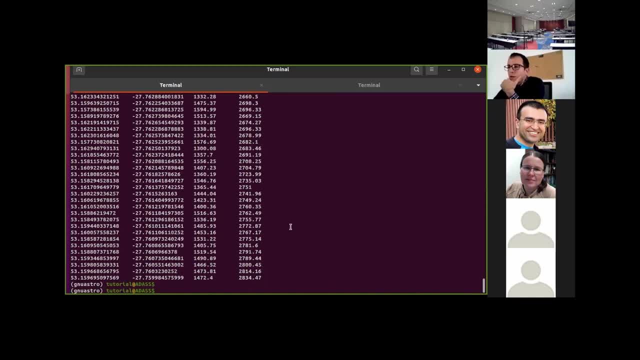 Okay, We have many different operators that you can have a look at the GNU Astrobook, But this is just one single example in which you can see the different things that we are able to do. So let's move now to another interesting program, which is AST query. 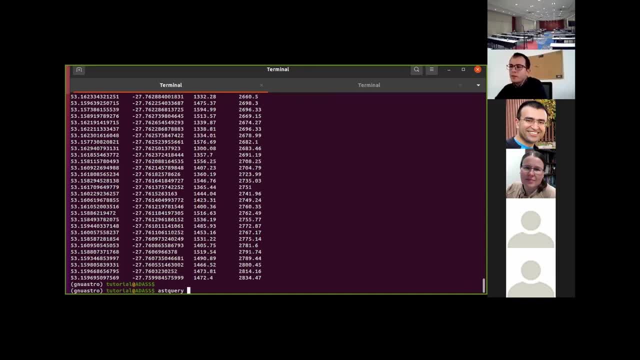 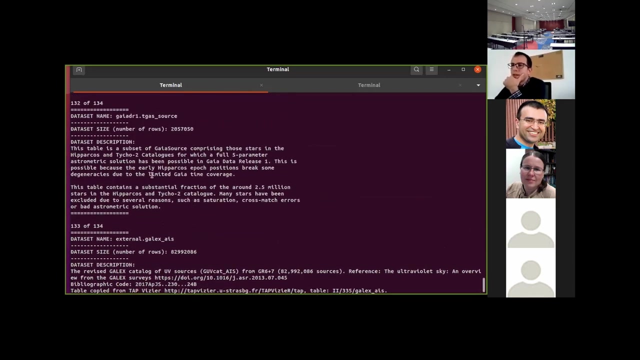 And, as you can imagine, this is for making queries to astronomical databases, for example, Gaia, Gaia or VCR. So if you type here, AST query, Gaia, dash, dash info, you will see that here we are retrieving all of the data, all of the metadata that belongs to the Gaia database. 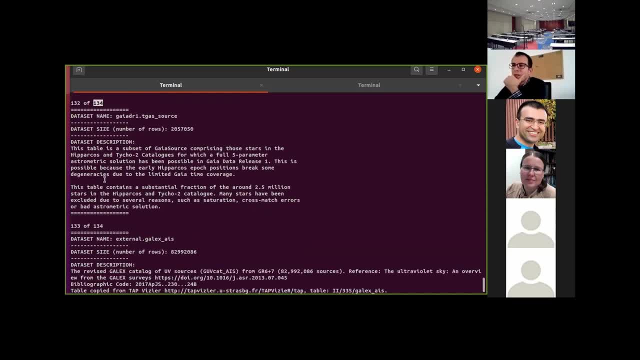 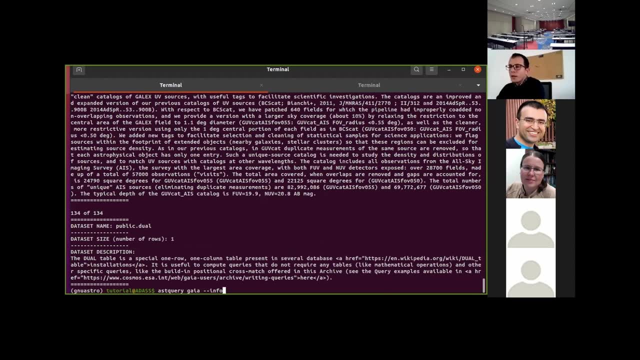 So we have here 134 different tables that we can use directly from into the command line. So, for example, just to specify a given data sets, Data set- Here we can say we want to obtain the data data release number three of Gaia. 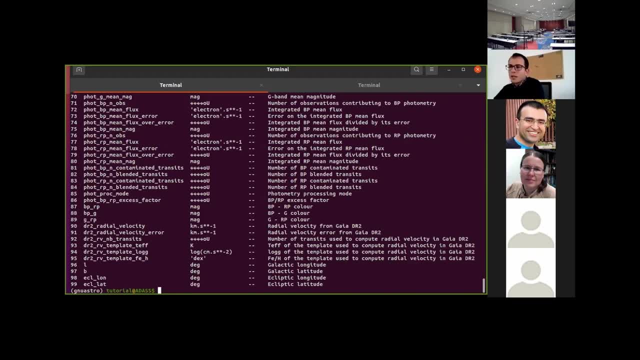 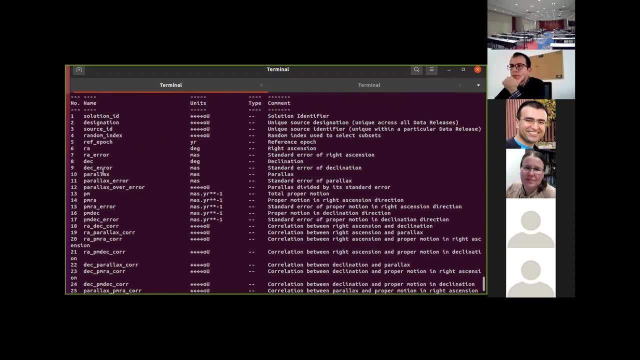 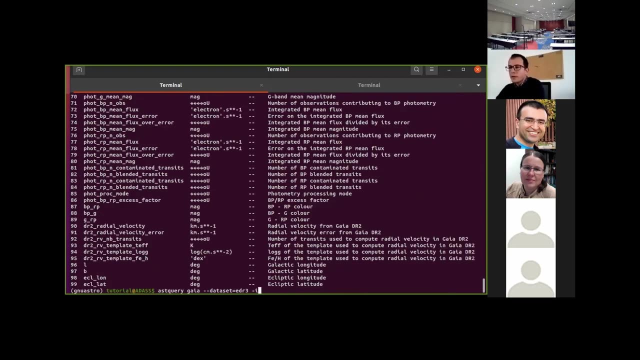 So let's print the information and you will see that for that particular data set we have the columns names. So you can, you can obtain that information from here. Okay, Another interesting feature is, for example, to have a look at the at another data sets. 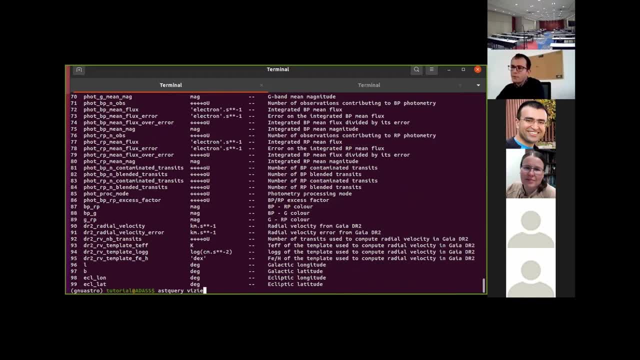 So the databases, for example This year, and now imagine, for example, that you want to look for some particular keywords. So just to specify here limit limit info, and I'm going to type here my two surnames: 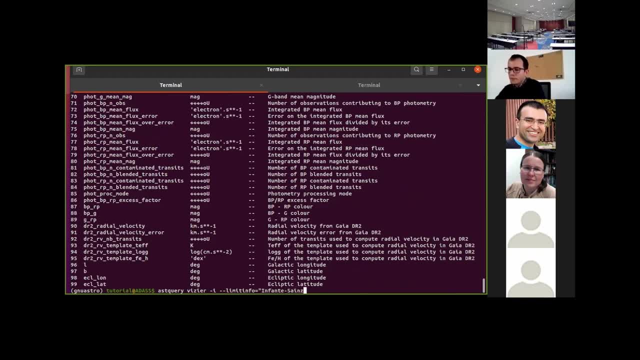 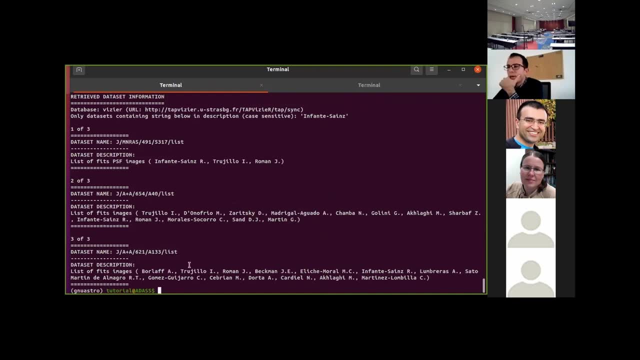 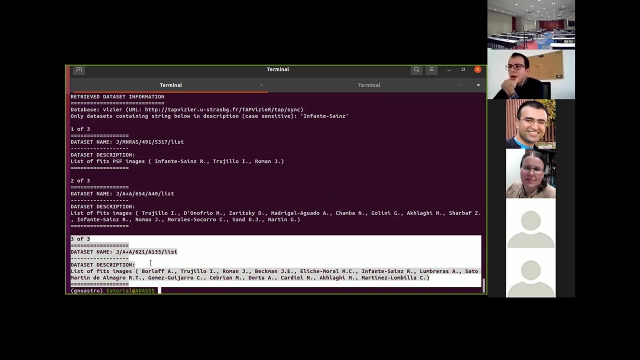 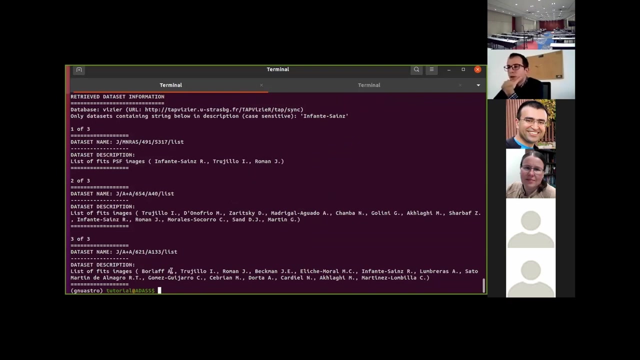 So infante signs. Okay, And just let's go and look for this, for this keyword into the VCR databases. as you can see Here, I have a couple of data set that I sent to VCR. Actually, this is the one that correspond to the images that we are using for the tutorial that were reduced, published by Alejandro Borlaff a couple of years ago. 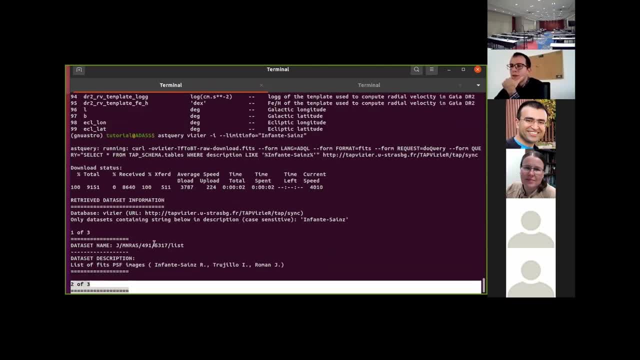 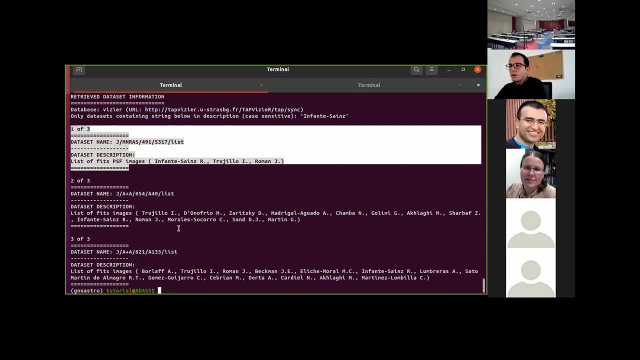 The next one is about the low surface brightness of some galaxies, And this one correspond to to the Sloan Digital Sky Survey paper, PSF paper. So So, but this one is Okay. So this is just to let you know that you can use this powerful feature for looking into the VCR databases just from the command line. 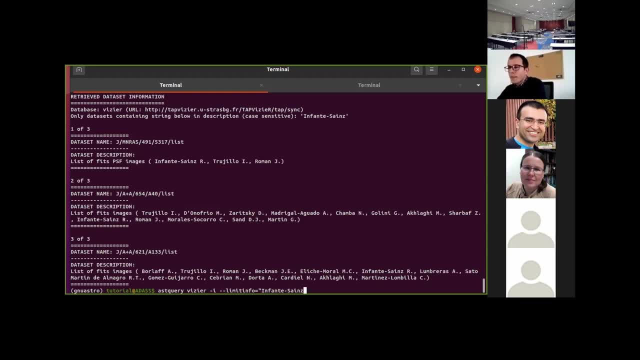 And this is really easy and really fast to use. So now let's go to use some data from Gaia. So we are we are going to download a catalog, So let's put like here, Gaia, the data set number three, so the R3.. 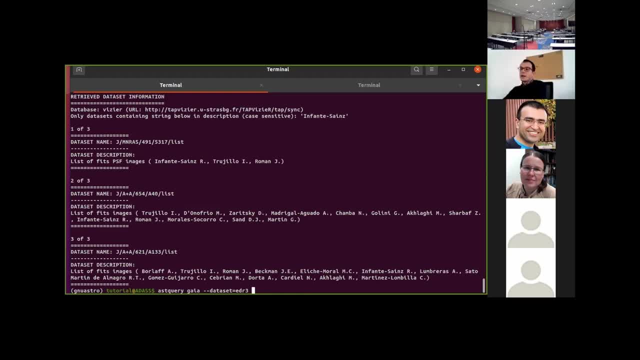 And now, Of course we don't want to download the entire Gaia catalog, but only those, that part, that correspond to our image. So we can say here, dash, dash, overlap, overlap with, and then our image Again. download the image and the filter. 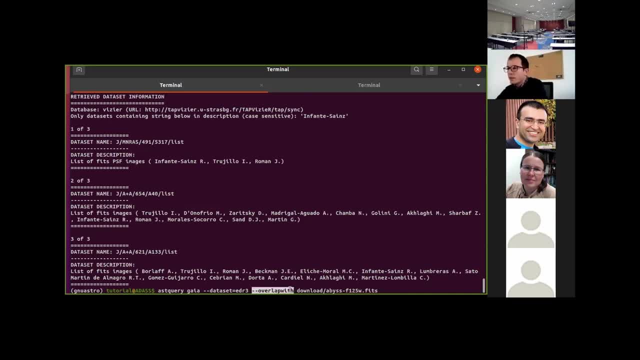 And now, instead of only downloading all the catalog, just that part that overlap with our particular image. Now let's specify the columns That we want to download, So for example, the source ID, the right ascension, the inclination and then the photometrical magnitude. 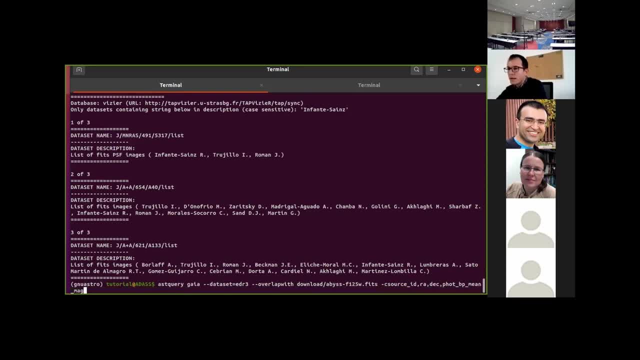 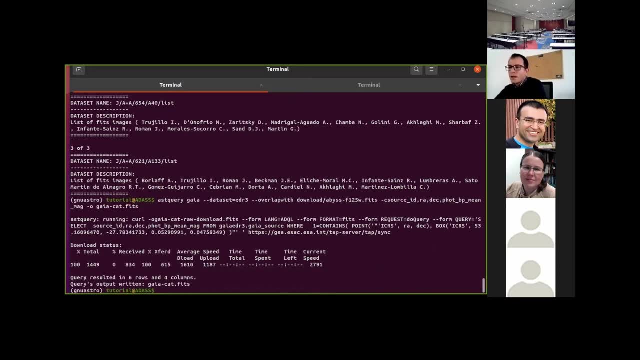 So the photometrical VP mean magnitude, And then let's put a good name, So Gaia dash cap dot fix, And that's it. So we have retrieved the data that correspond To our, to our image from Gaia, And you can see here that it consists in a table with four columns, which are the ones that we have requested here. 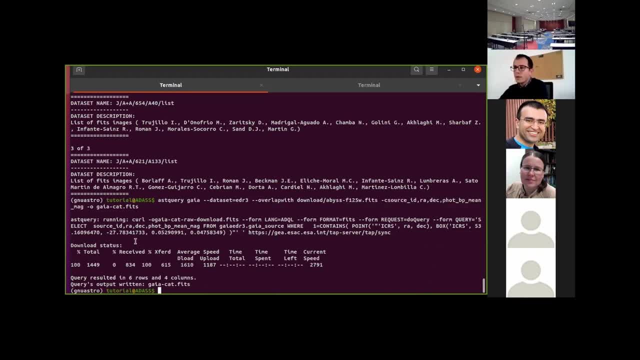 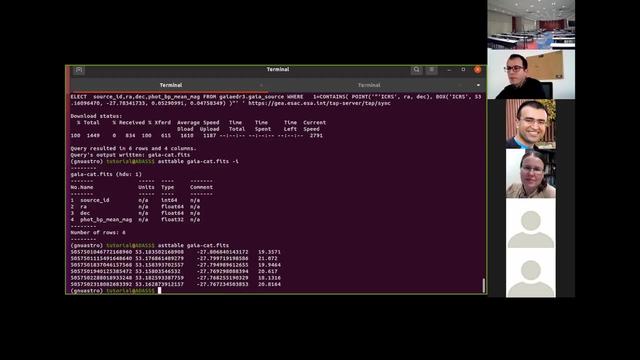 And three, sorry, and six different objects. Okay, If we have a look again with AST table Gaia catalog and the information, you will see that this is actually the case. This is and this is the raw data. Okay. 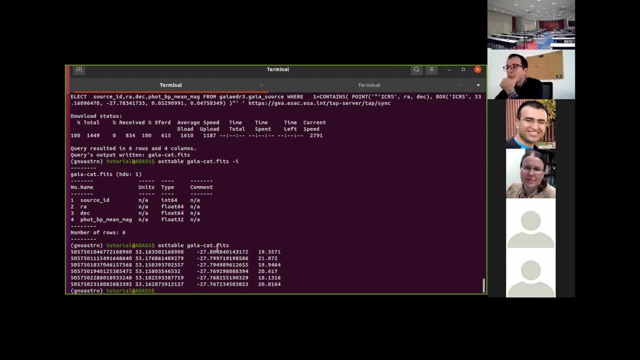 So now let's move to the next program, Which is AST match. Now that we have computed our own catalog with AST make catalog and we have another external, external catalog from Gaia, We could make the match in between that- two different catalogs. 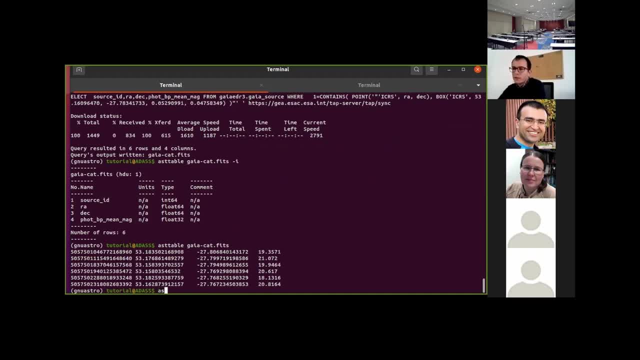 And for doing that, we are going to use the next program, which is AST match. Okay, This is a program for making the match. Okay, This is a program for making the match. This is a program for making the match of astronomical tables, and just let's do it. 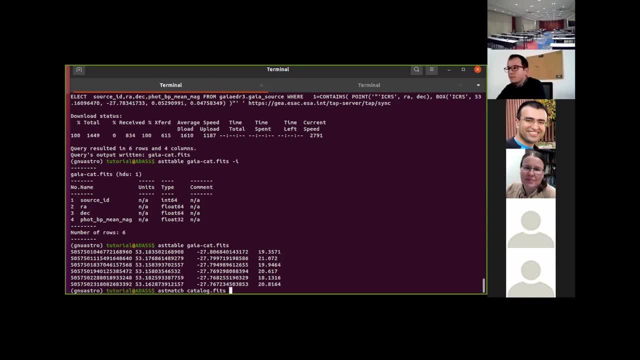 So give, for example, the first catalog and the extension that we want to use, So extension number one, for example, just to put here the name explicitly, then we are going to use the right ascension and declination for the matching roles. 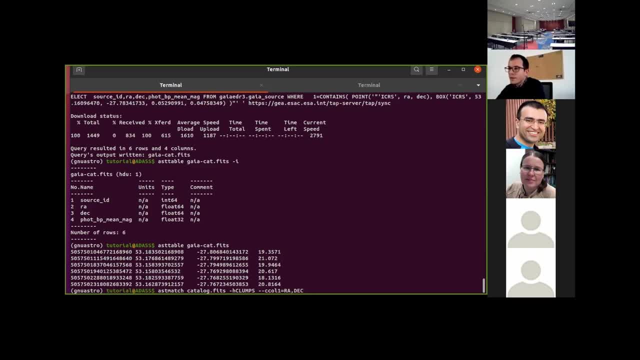 So right, ascension declination. This is what we are going to use for the first catalog, for our catalog, And then do exactly the same for the Gaia catalog. We are going to use this, the first extension, So HDU2, because this is from the second catalog, number one. 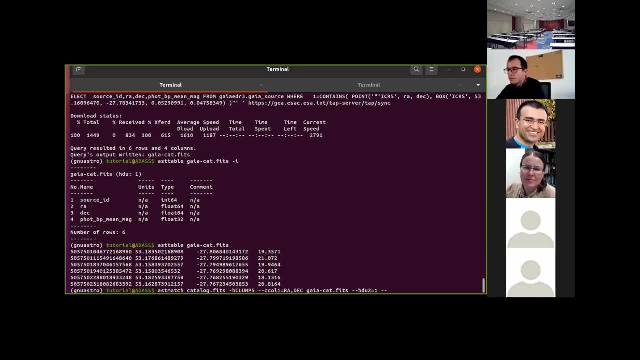 And then we are going to use the right ascension, So C4, number two, Again right ascension and declination. And now we have to specify the aperture in which we want to make the, the, the match. Okay. 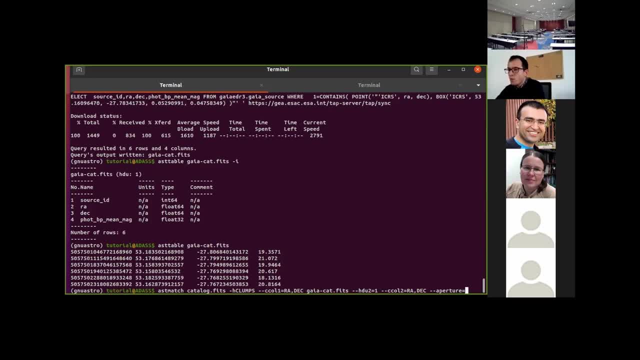 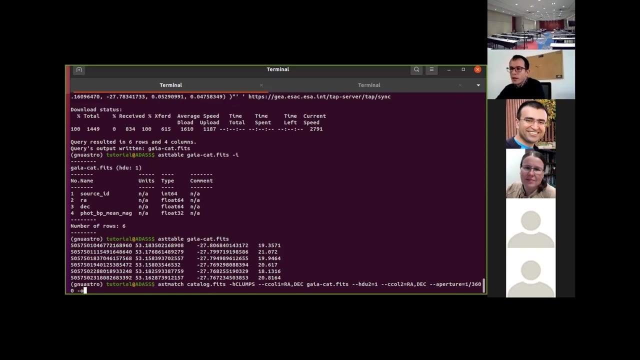 So aperture equal to one arc seconds. since we have specifying here the columns in degrees, we have to specify also the aperture in degrees. So divide here by 3,600.. And then, for example, the output will be Gaia match. 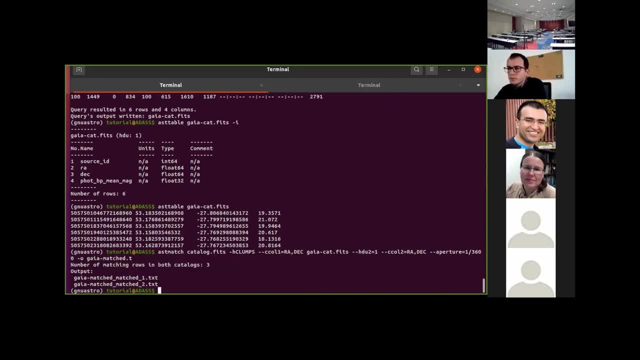 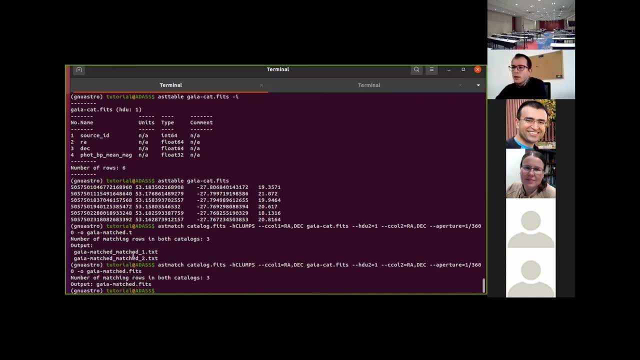 And that's it. Sorry, And that's it. We have obtained the output, which is actually the the match catalog. So AST fits, Gaia match fits, And you will see that inside of this file, which is the result that we have obtained, we have two different extensions. 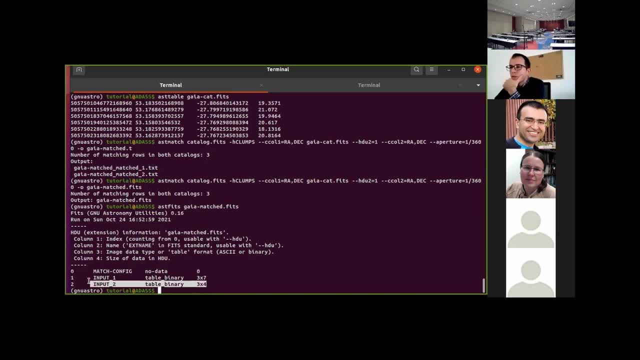 One corresponds to the object that we are going to use for the match. Yes, were present in the, so once correspond to the columns from the first, from the first catalog for the object that are match, and the other one for the second catalog, if you would like, for. 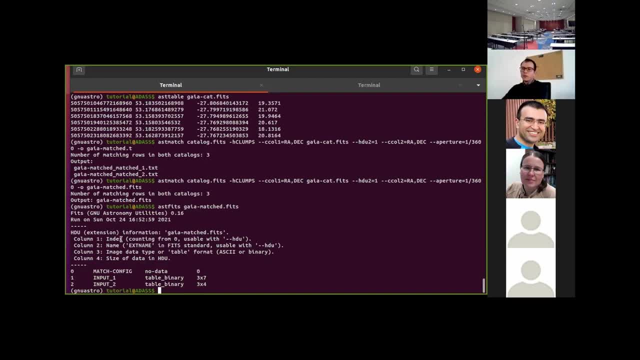 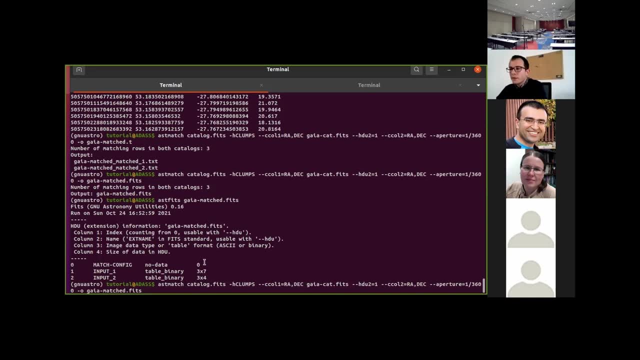 example, to obtain one single extension, one single file for the match result, we can specify this with the next, uh, with the next option. you could say here: dash, dash, out columns, so out calls, and then specify which calls, which column from each catalog. do you want so, for example for 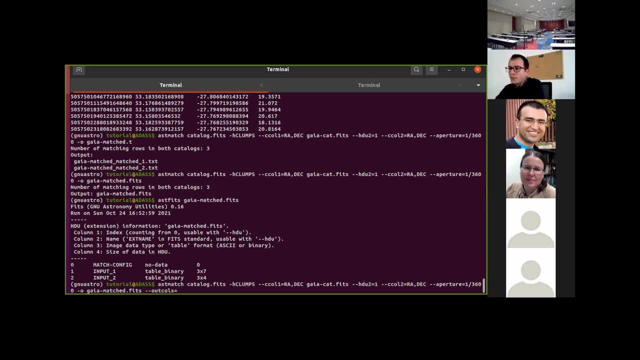 from the, from the first one you decide, you just has to type here: a: for the first one, we i want the right ascension. and also for from the first one, i want the declination and the magnitude, okay, magnitude. and then for the second, which correspond to the gaia one, okay, so i put here b, i want the photometrical. 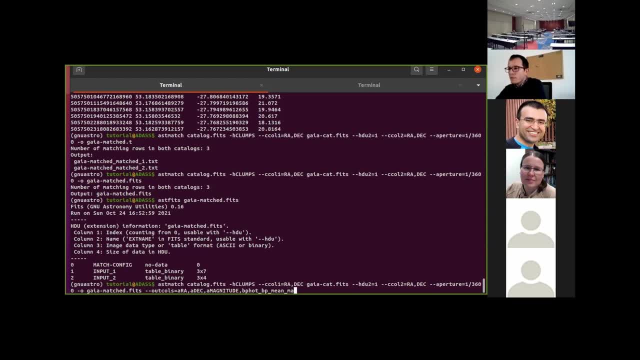 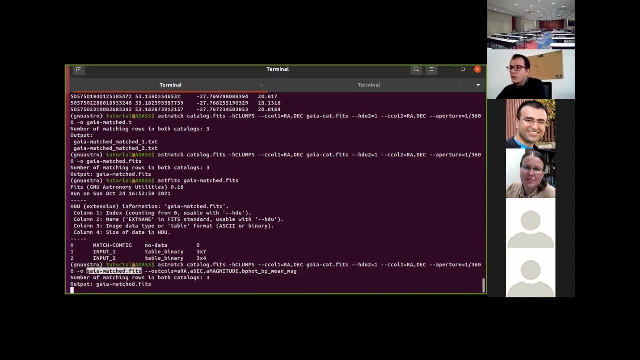 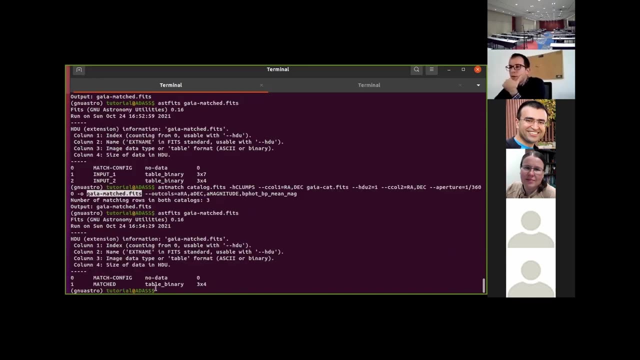 magnitude. okay, so bp mean magnitude. and now let's put here: and that's it, because we have already specified the name here. so just press enter. and now, if you have a look again at the output, you will see that the output now is only one single extension. 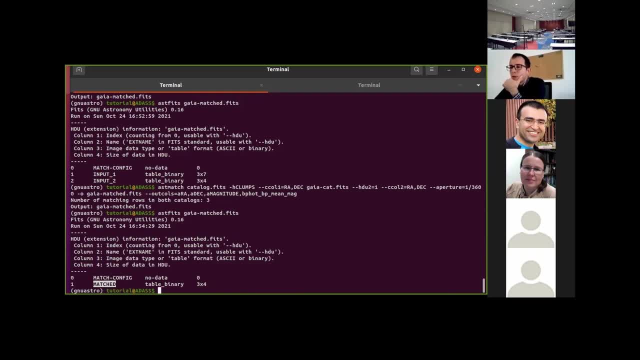 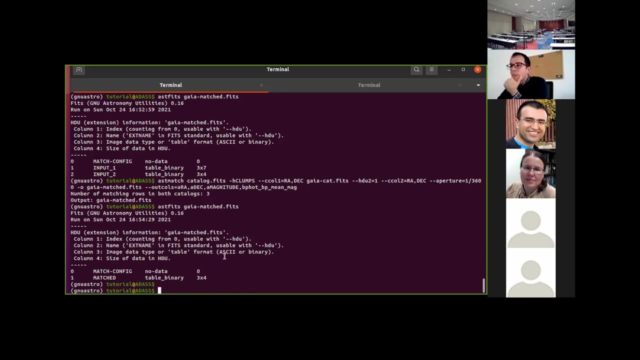 in which you have the match object from the two different catalogs. okay, so this is really powerful when, when matching really large astronomical catalogs, and it is done in parallel and very efficiently and really fast. okay, let's now go to the next project, which is for obtaining the statistics of of images and astronomical tables. 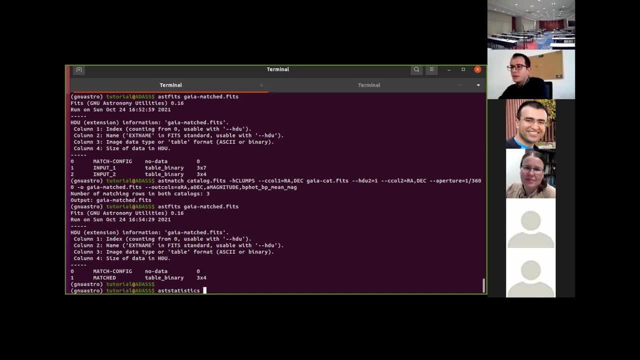 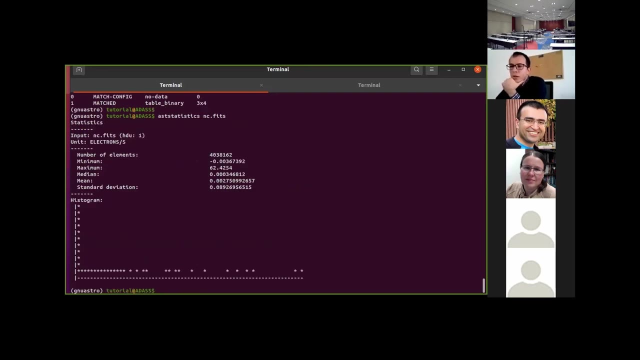 and the name is ast statistics. as you can see, here now we are going to obtain, for example, the statistics of the noise digital output. remember, this image is noise chisel and just presented in, it is going to compute the basic statistical input information of this image. so here you can see that the number of elements, so the number of 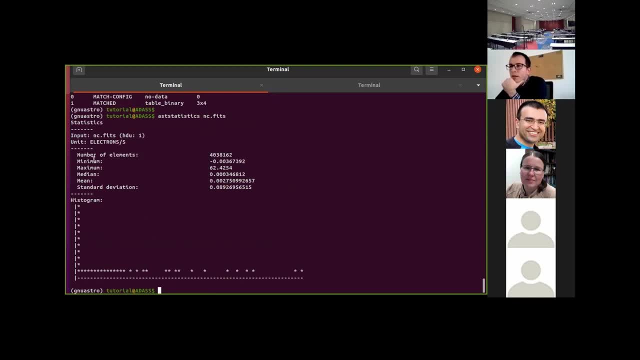 pixels is this one. it is going to obtain the minimum, the maximum, the median, the mean and the standard deviation values, and also it is going to print on the command line a very nice histogram. that is really useful when, for example, you are working on a super computing facility. 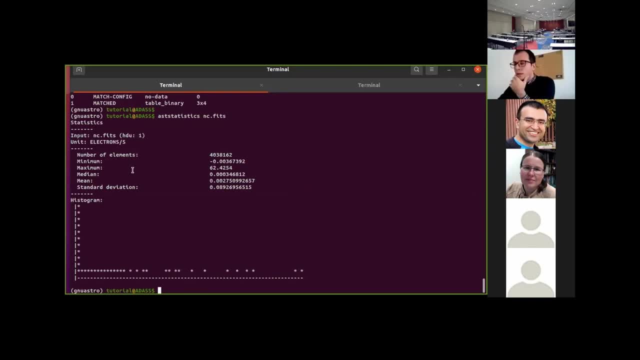 and you don't have access to a graphical interface for having, for example, having a look at the histogram or any kind of plot. so you don't have to go to to download your the data to your local machine and so on. so here we can see that we have some. 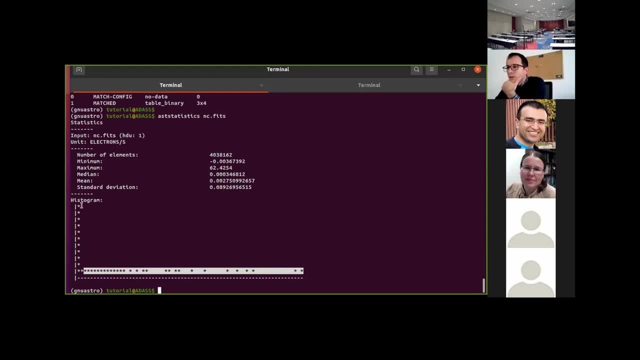 pixels which are very bright. so this is the pixel distribution value, and so now we have different options that we can play with. so, for example, let's have a look at only those pixels that are below given value. so let's down, for example, 0.005, and then statistics is going to compute, only the statistics. 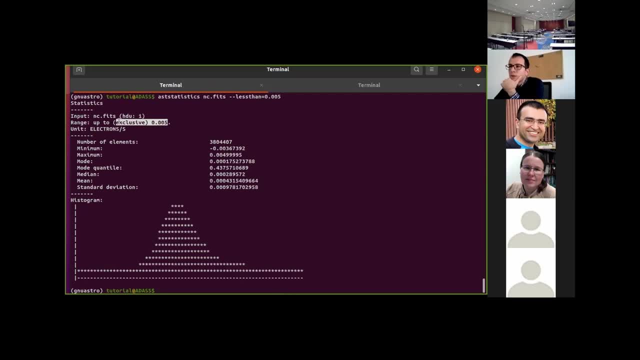 for those pixels that are in the range of pixel value that we are specifying. so again, the pixel, the number of pixel is different. the mean maximum, the mode quantile and so on, they are different and, as you can see here, the distribution is also different. so this corresponds to the pixels that are pointer, so essentially to the 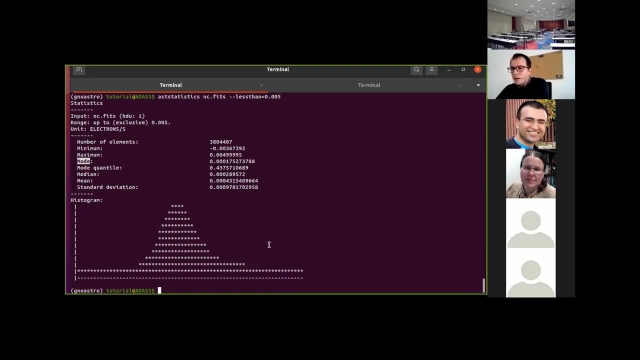 sky background pixels. Okay, so now, instead of having a look at all of these measurements, imagine that, for example, you would like to obtain only the mean. so you just have to type here mean, and it is gonna print on the command line really fast, the mean. and of course you can. 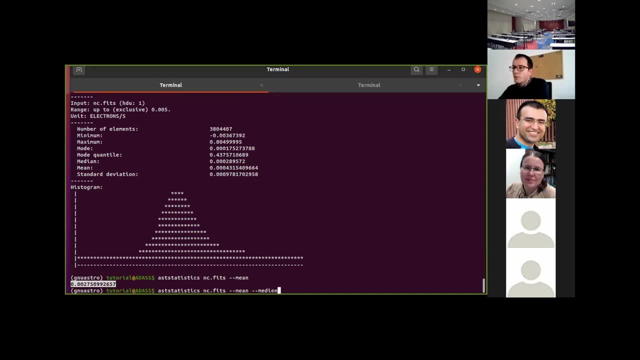 do exactly the same, for example, with the median and the standard deviation, And, for example, imagine that you would like to compute the skewness of this, of this image. so then you will, by talk Just to make this computation Okay. so I mean that's, by doing this We can print. 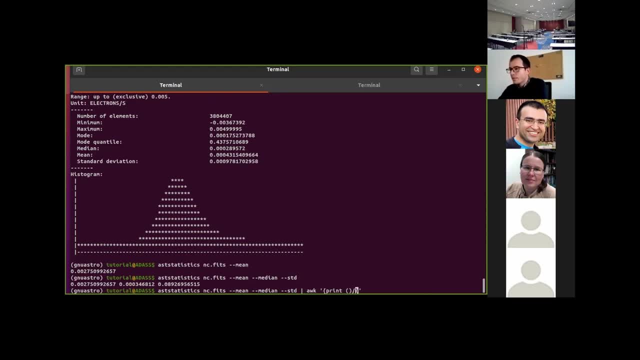 the result of computing the skewness. here the skewness is defined as the, as the mean. so the first concept column, the mean minus the second column, divided by the standard deviation. So this is a measurement of the skewness of this image, as you can see here and now. 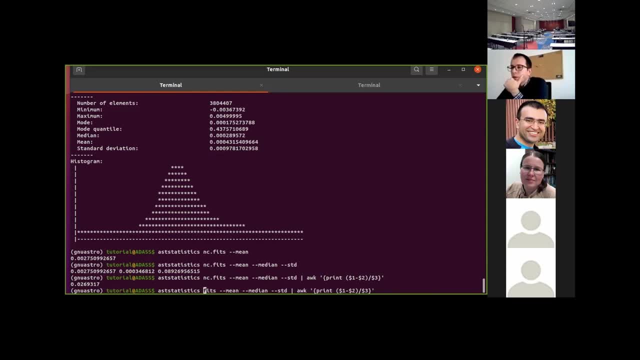 for example, imagine that you would like to compare this with the image in which we only have the sky background, because the signal were masked as I showed before. So now you can compare the different skewness of these two different images and see that. 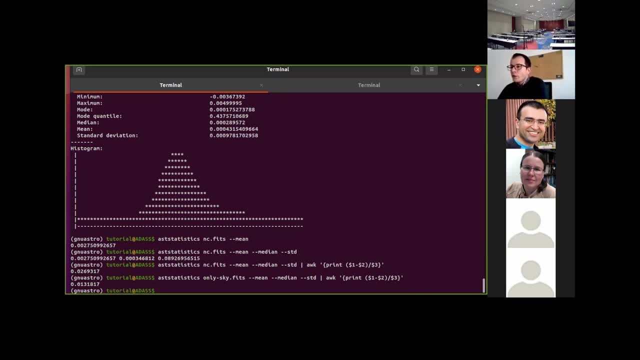 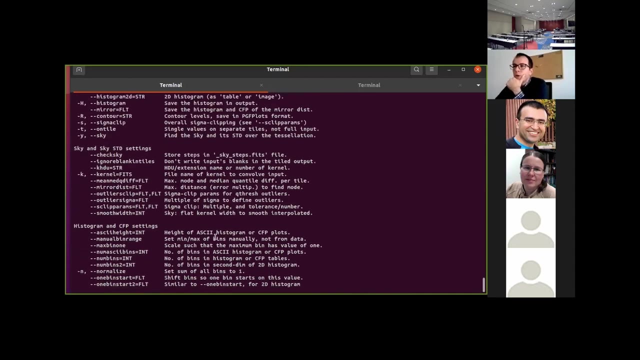 actually they are different. Of course. again, we have many different operators that you can use here. We have also SigmaClip. just to have a look at all of them, you can use the option help or go to the book into the website to check what are the different options and all of the information. 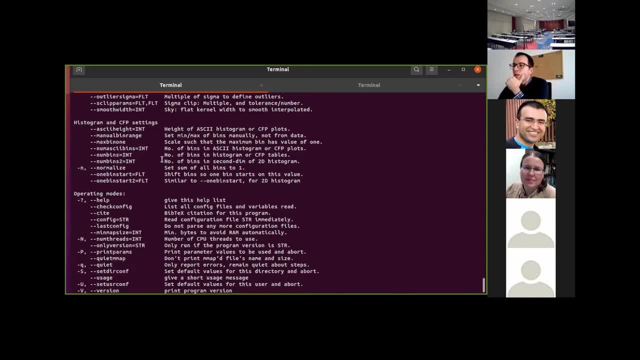 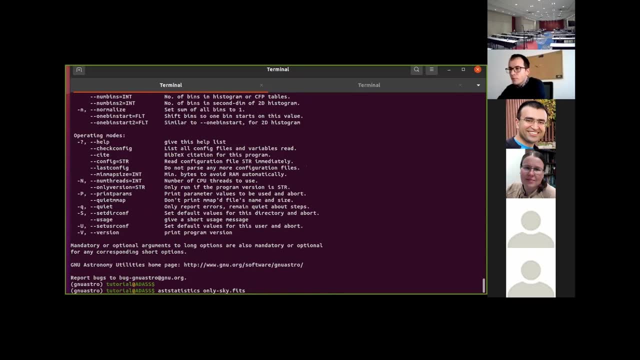 related to all of them. So another interesting measurement are the ones that correspond to the Sigma Clipping values. So, for example, to obtain the statistics using the Sigma Clipping values, Sigma Clipping operator. sorry, so dash dash, Sigma Clip is going to compute the Sigma Clipping. 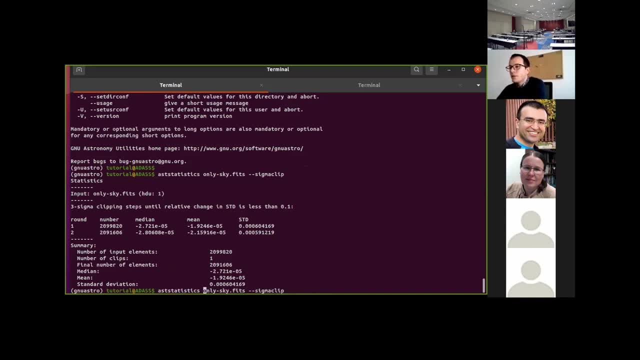 values. so let's use, for example, the original image just to see more iterations, which is the fit, and it is going to compute the Sigma Clipping values for the number, the median, the mean, So the main parameters, right, So you can see that it. 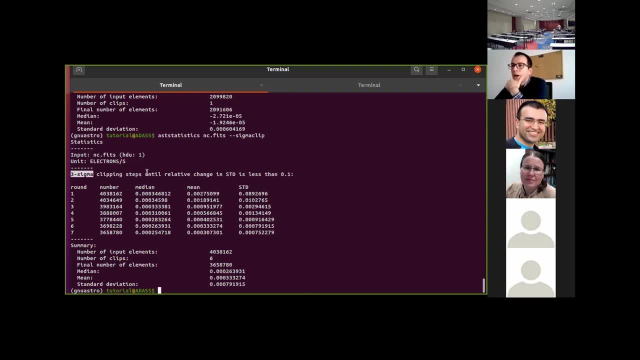 is computing by default 3 Sigma, Clipping until it reaches a given tolerance. Of course you can. you can change the 3 Sigma to be another 1, like, for example, 2 Sigma or 5 Sigma, whatever you want. 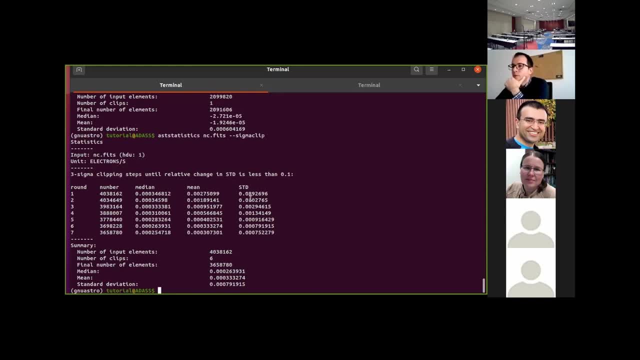 want and also the tolerance. So it computes different iterations until it reaches the tolerance level And the final results you can have a look at here. So this is done really fast, as you can see, and it is really powerful, And then again you can use the AST statistics. 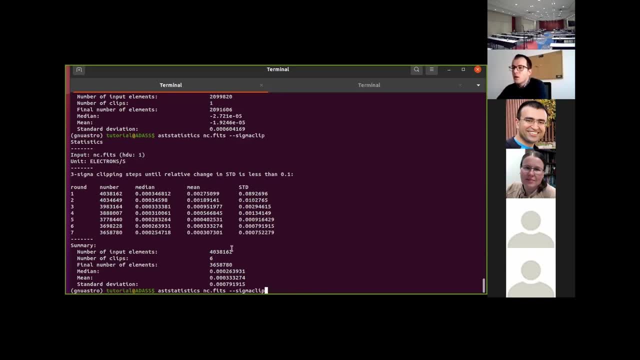 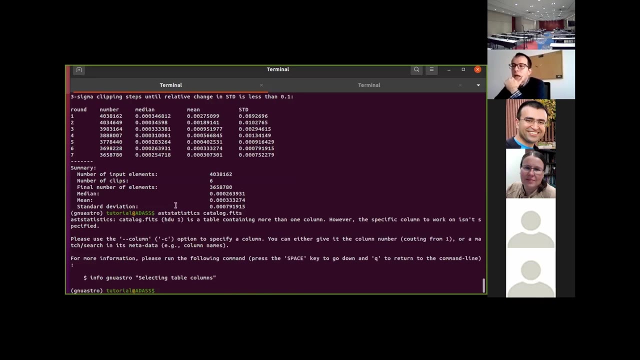 for example, with the catalog, not only on images. So if you provide here the catalog that we were measuring before, you can say S AST, statistics catalog and just presenter, And of course it is going to complain because we have different columns that you cannot mix together. So you have. 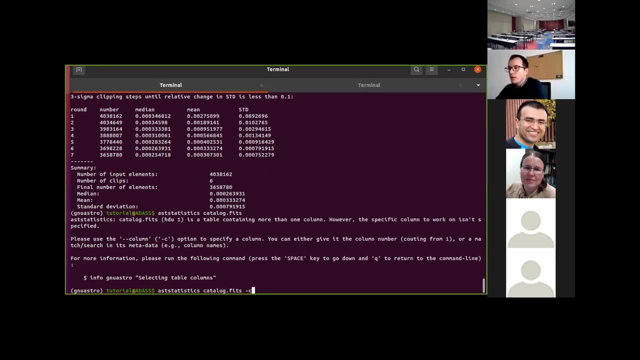 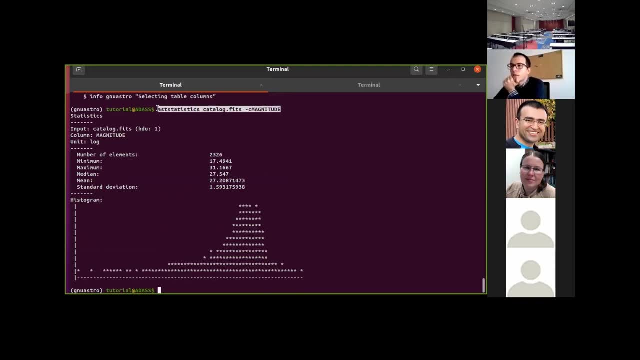 to specify a given column, So for example, C magnitude, and it is going to compute. So this is the line that I have just executed And it is going to compute the statistical parameters for that particular column. As you can see here, this is the minimum value, the maximum and the distribution of values. 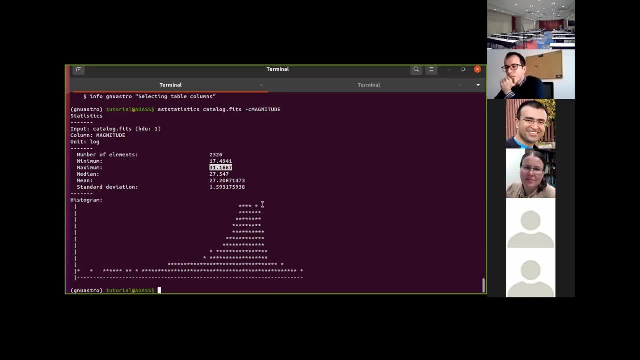 as you can see here. Okay, So now let's move to high level features. So now I am going to review, for example, another program which is AST Convert type, And this is designed with the goal of converting different data sets, So different for converting data sets into different format files. So 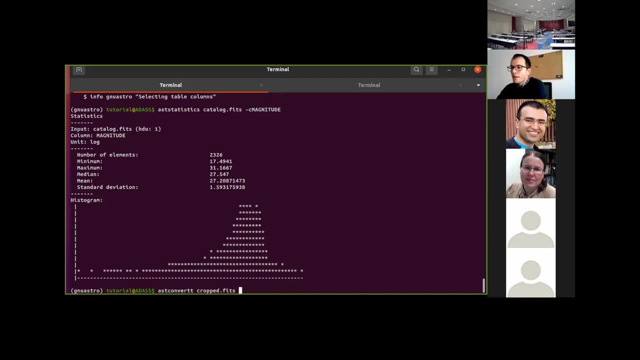 for example, let's have a look at the crop image: crop feeds. So instead of having a look at the original feeds file, with this program we are going to convert this feeds file into a JPG image. So just to specify the output, crop JPG- and it has done the conversion. 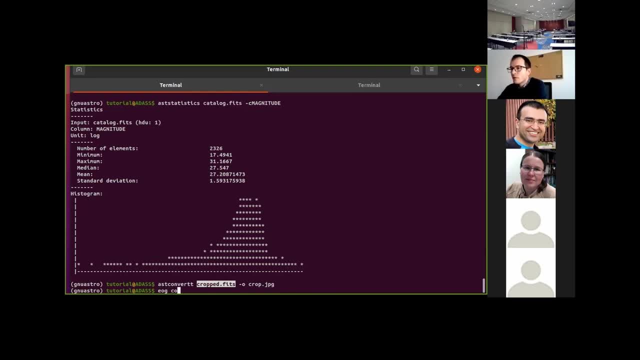 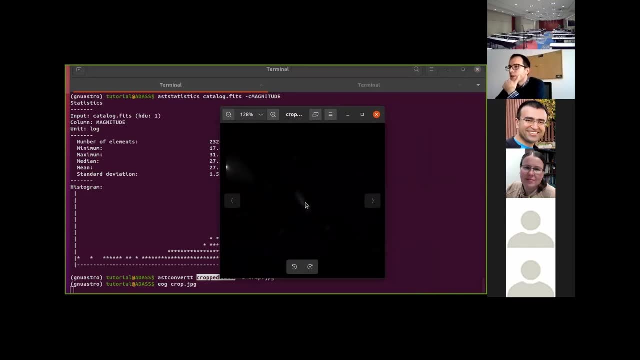 So right now we can use, for example, the OG to have a look at the crop image, And here you can see that we have this small image in which in the center, we have the galaxy, But of course, the appearance of this image is not. it's not so nice. 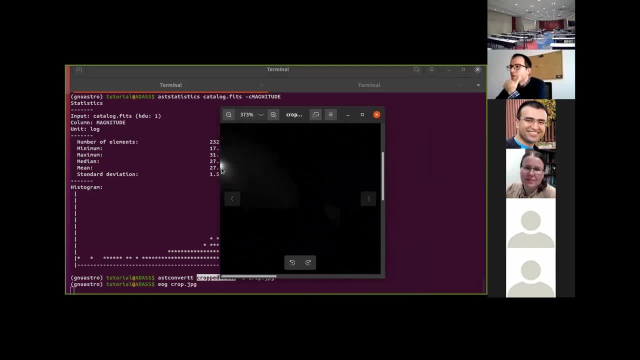 The ability of this image to have very strong tons of pixels, And this is because we have very bright pixels, for example this one that is in the border of the image. So AST convert by default is trying to represent all, so the entire range of pixel values. 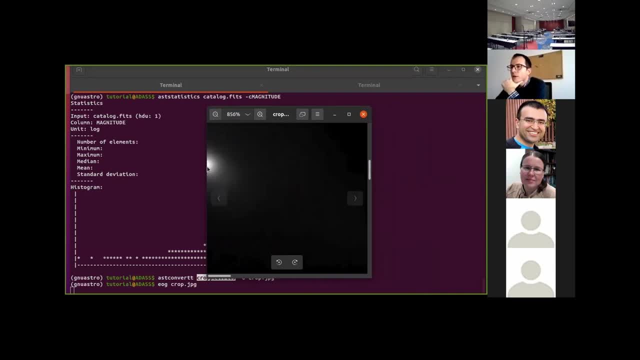 in a linear scale And because of the very central part. so the central part of the very bright object is a pixel value very high and the sky background are very pixel value very high And then you can just put little universo, So the object may some little. 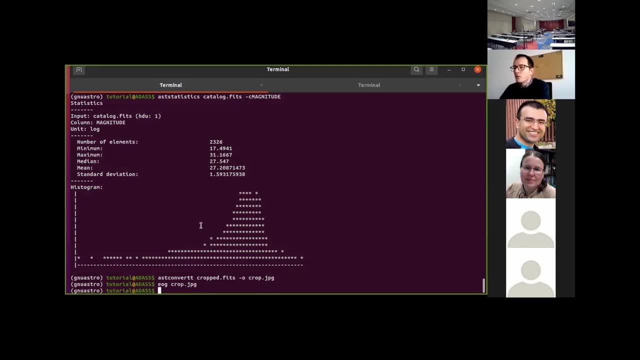 bit of that picture, but still some pixels that we don't really look. you should suppose, but they still don't have the vertical and full and this doesn't have the vertical low. it is almost impossible to have a good image with such a huge amount of pixel value. 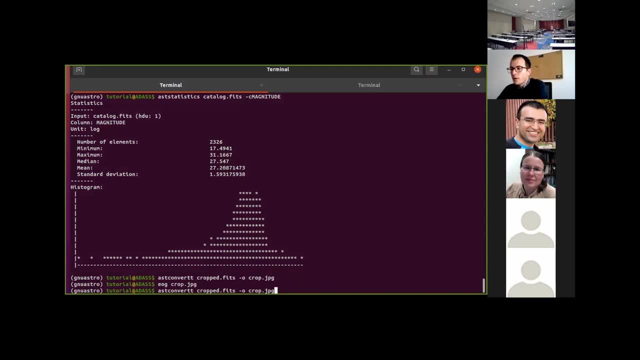 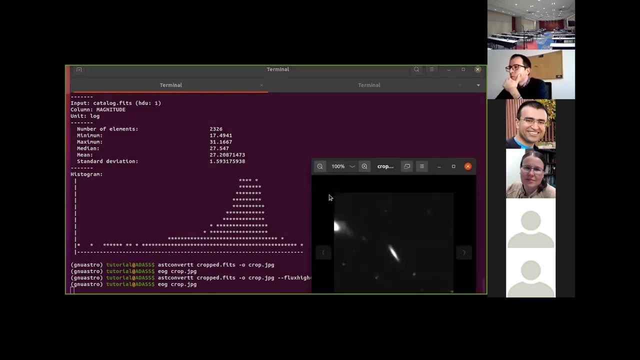 So to solve this, we have the possibility of specifying here the maximum value for the pixel that you want to represent, So flux high, for example 0.1, and I do this. Of course, we are going to improve a bit the image, as you can see here, but the center is going to be completely. 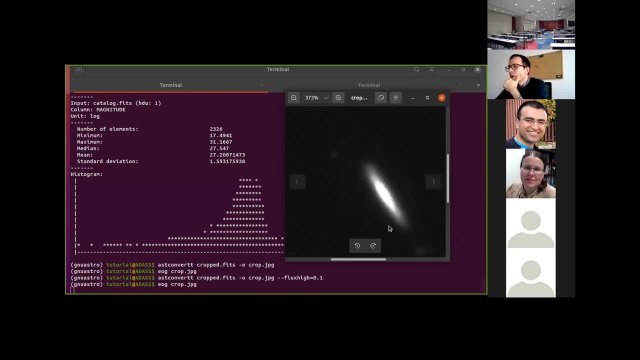 saturated, So we have some more information. You can have a look at the other part of the images, but of course, the result can be improved a lot. So here we have also many other different options. For example, instead of keeping this image as JPG, you can just save as APS, which is 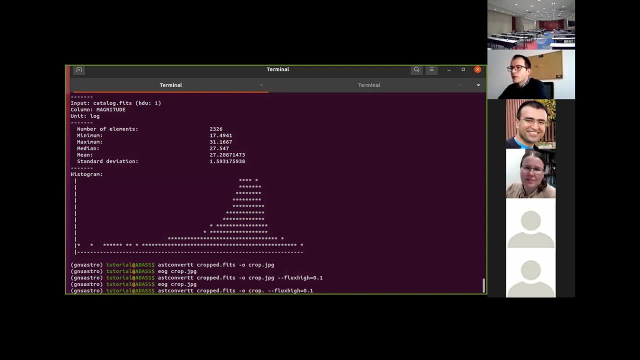 more convenient, for example, when obtaining images for papers and publications. so APS, and it is going to automatically make the necessary conversion for obtaining in the APS form. So let's have a look at the image that we have just created: APS. 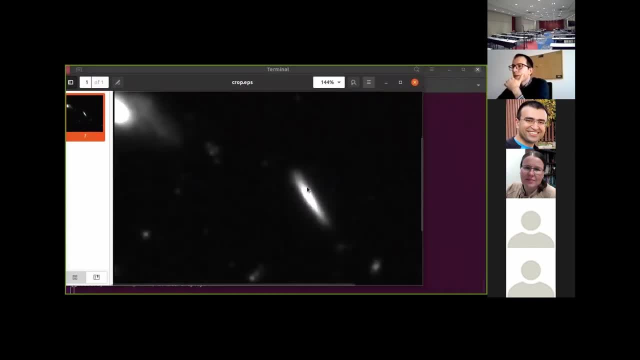 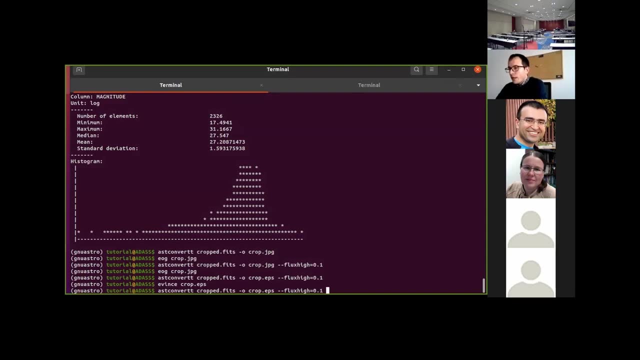 oh, really big. okay, and here you can see that directly. it has been converted to APS. We have different options. for example, we can change the color map, color map and, for example, select the briefings, which is the typical one. that 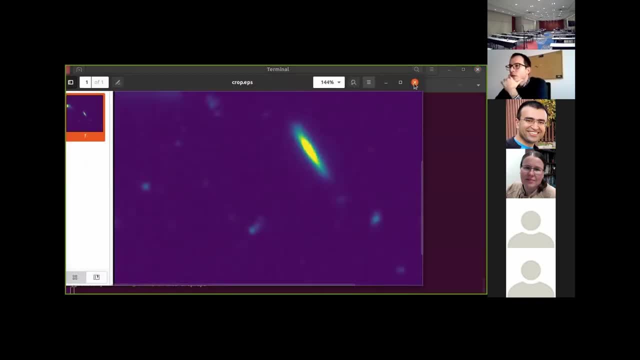 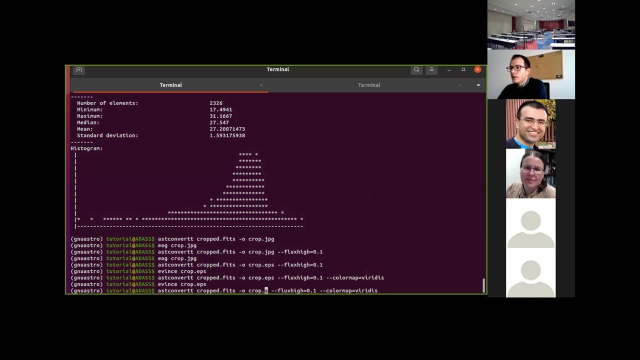 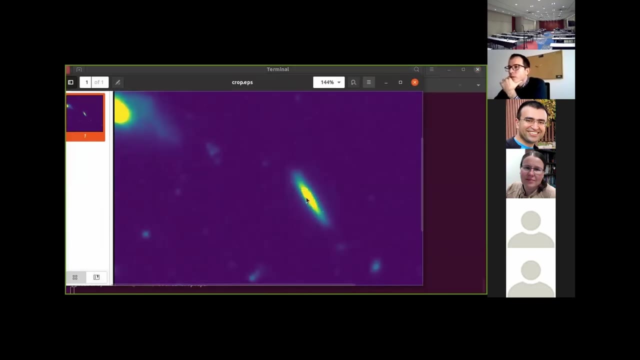 is not probably usable by default, as you can see here. Okay, and we also can compute the PDF, the image, in PDF format. Okay, again, if I change two of these, this image, you will see that this is in. so it didn't change. 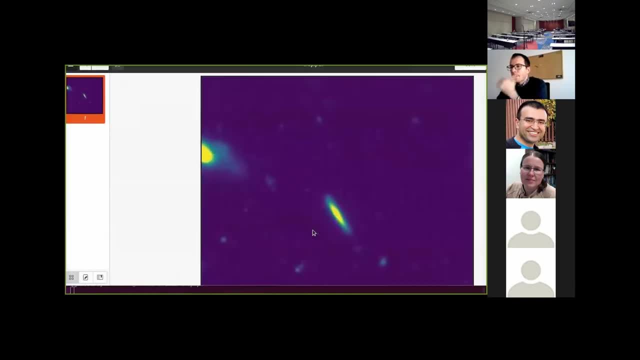 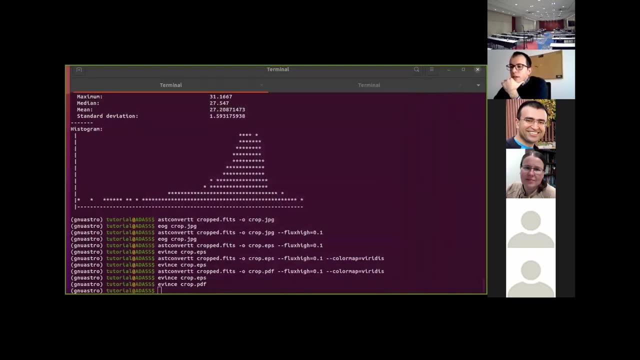 crop PDF Here. So this is the PDF that the AST crop is generating. So now, instead of making this kind of fake color image, let's say, since we have three different images for the same region of the sky, as you can see here- download. 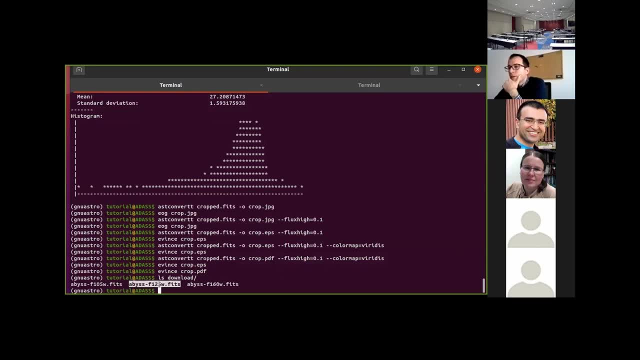 but we have been always treating this image but we have other two, So this is the redder and this is the bluer and this is in the middle. okay, So we can assign each one of these image to one color channel and give all of them to AST convert. 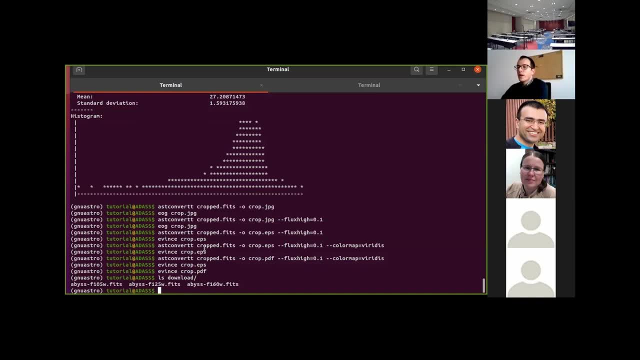 to generate a color image. okay, And this is actually what we are going to do. So AST convert: we have to give the images from redder to bluer, so download this filter, the download the other image in the next filter and the last one, which is the bluer. okay. 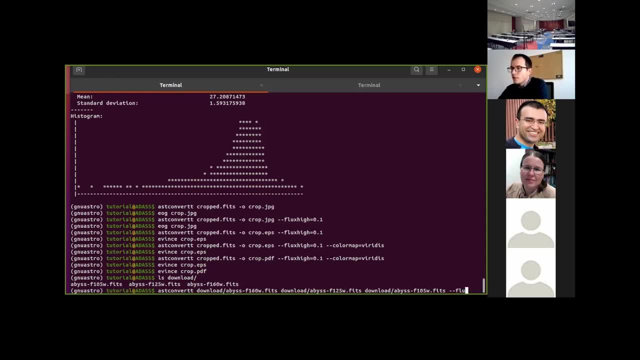 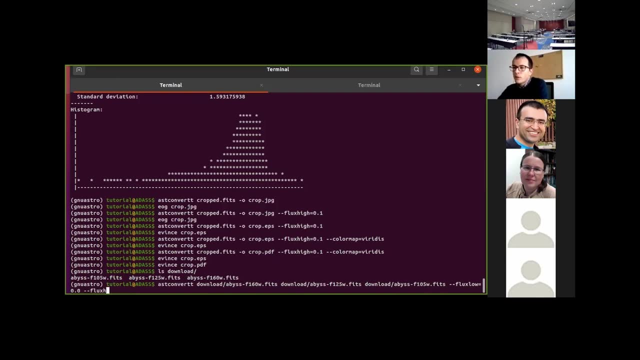 Now let's specify the flux range. So dash dash: flux low, equal to 0.0, to not have negative values, and flux high just to keep the the brighter regions- 0.001, for example. and then output color dot JPG. 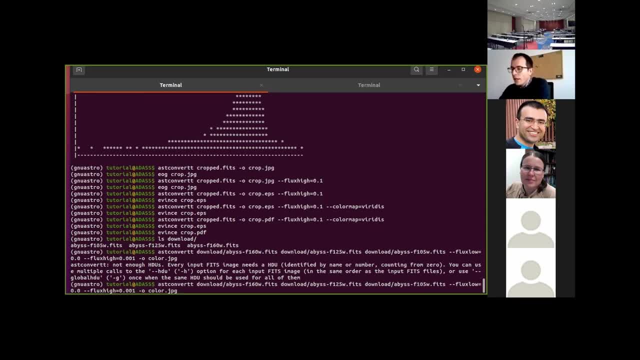 Okay, and it is saying that I have to specify an HDU for all of the images. So in this case, since I am going to use the extensive number one for all of them, I can specify a global HDU. so dash G1,. 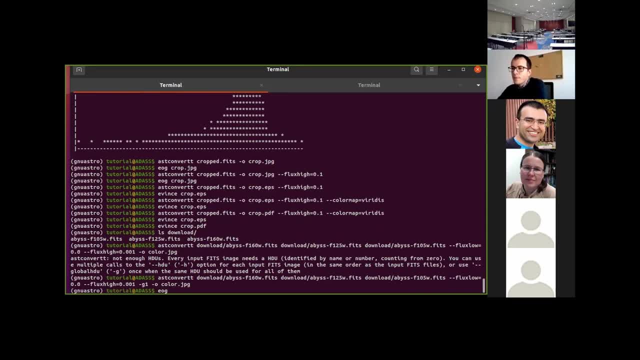 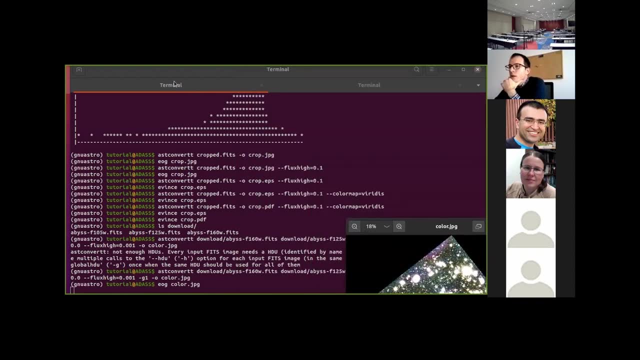 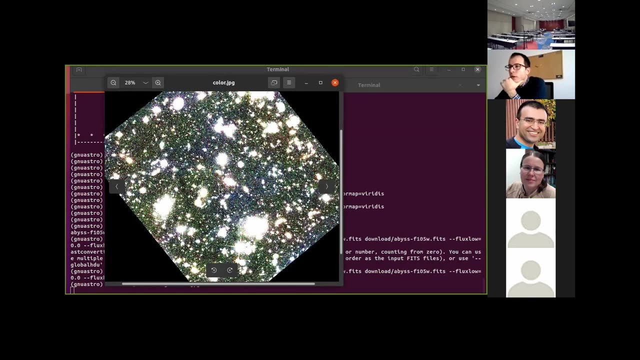 and it is gonna make the color image. So I have to specify the color image and then output color dot JPG. So this is the kind of image that we are computing. with this image, Of course, it has many different options that you can play with in order to improve the results. 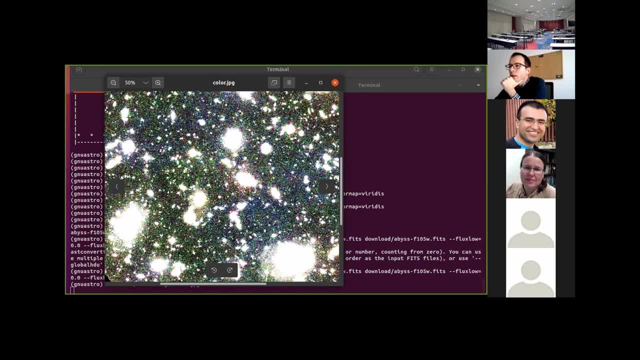 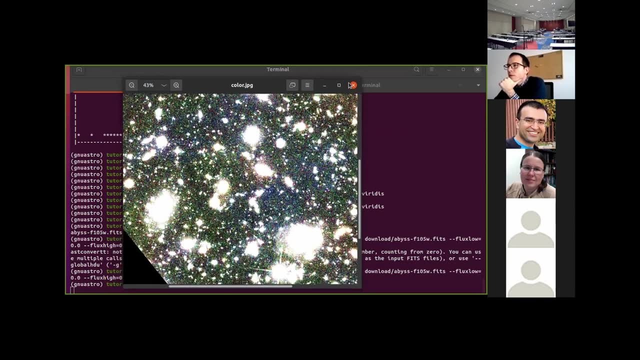 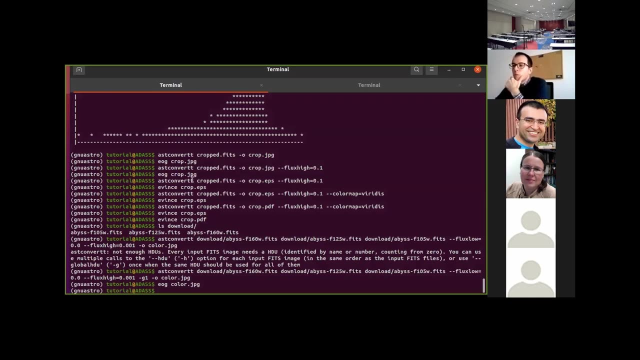 But in general we have the problem that we are showing here, the pixel value distribution in a linear range. So to solve this I am developing a script of, let's say, calls to different GNU Astro programs in order to obtain automatically a 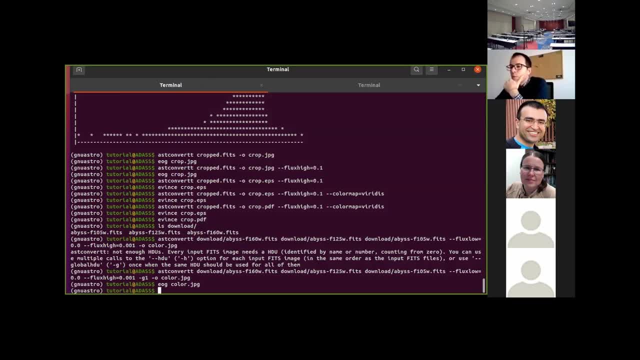 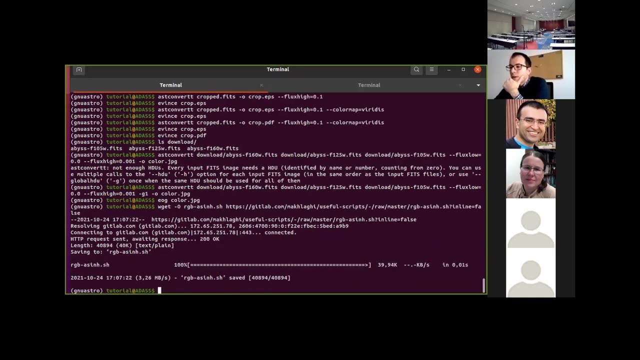 good set of parameters to represent color images, to create color images. So this script is actually in this direction. I can download this script. It is not in GNU Astro yet, but we are working to include this script as part of some other GNU Astro program as soon. 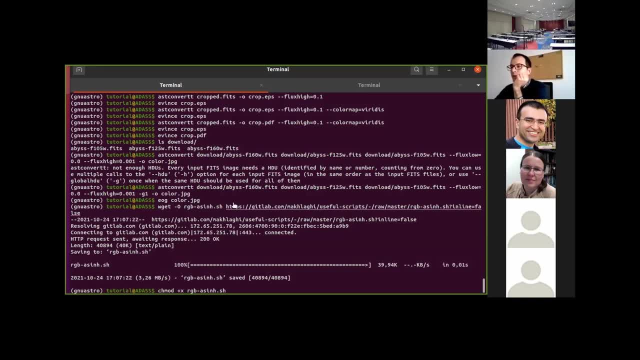 as possible, And this is a perfect example in which you can see that you can use different GNU Astro programs for making the analysis of your astronomical data in the proper way, using the well-defined blocks of programs that I have just reviewed before. So let's give permission to this script that I have just downloaded. 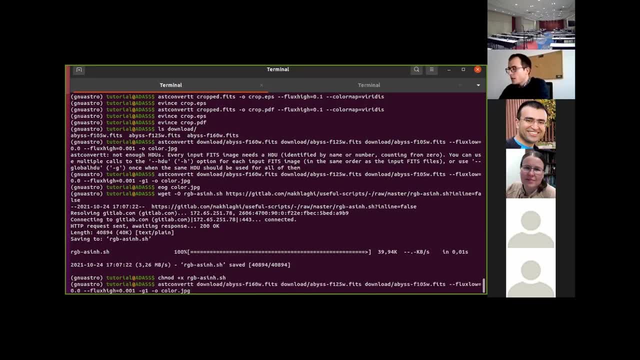 And now let's go to the next slide. So let's give permission to this script that I have just downloaded. And now let's go to the next slide. So let's use this instead of the original AST: convert So RGB. And then we are going to use this script on the original images that we were using. 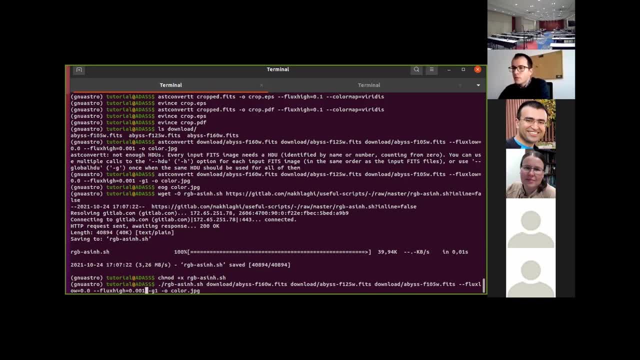 So let's modify a bit the parameters. Okay, let's remove this because they are not longer necessary. So again, hdu equal to one. So basically, we are doing exactly the same. We are giving the three different images from redder to bluer. Okay, and now we want to specify here that the 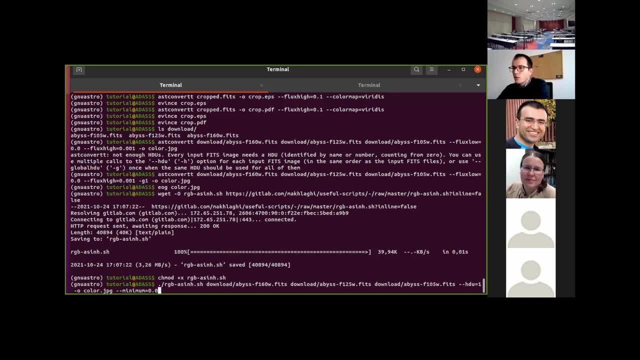 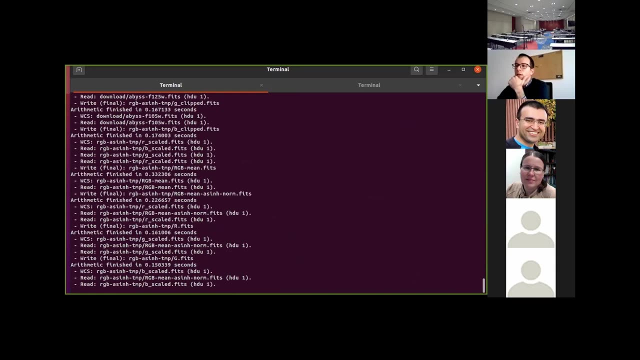 minimum value is equal to zero, because we don't want negative pixel values, And then specify an output name, So, for example, colorjpg, And it is going to make different operations. So, arithmetic- as you can see here, arithmetic is being used a lot. 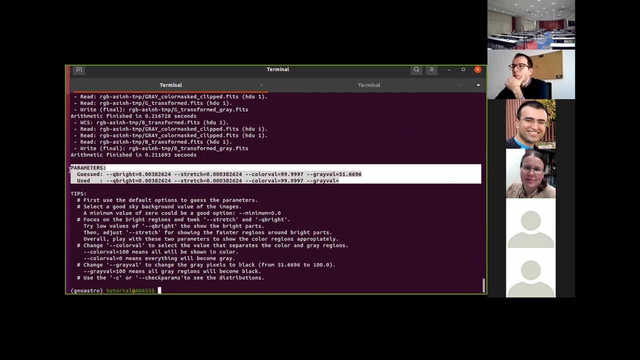 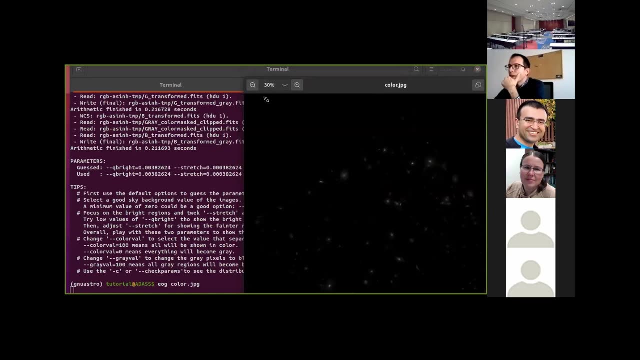 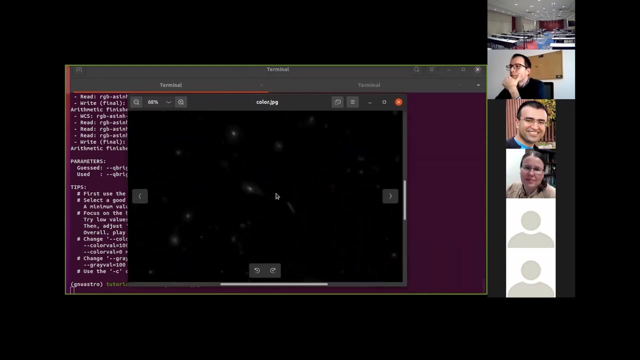 And it is able to compute automatically some parameters that you can play with for obtaining a good color image. So let's have a look at the image JPG And here you can see that it has computed the necessary transformations for obtaining a better color image. So, essentially, this can be improved a lot, as you will see. But basically, 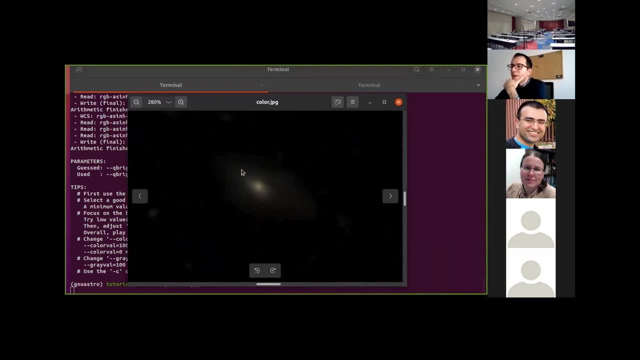 what it is trying to do is to make the transformation of the pixel distribution using an arc cosine hyperbolic function. So all of the details about this transformation was published some time ago by Robert Lupton 2004.. So you can have a look at that paper to study the details. 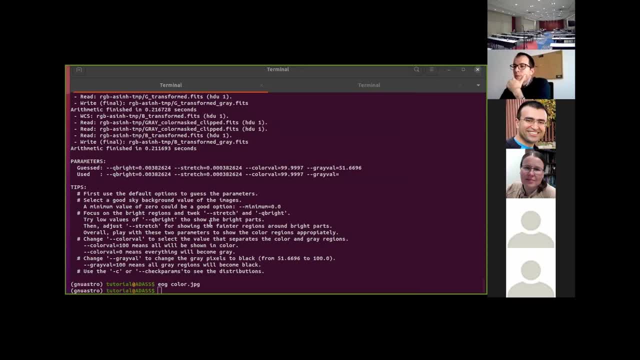 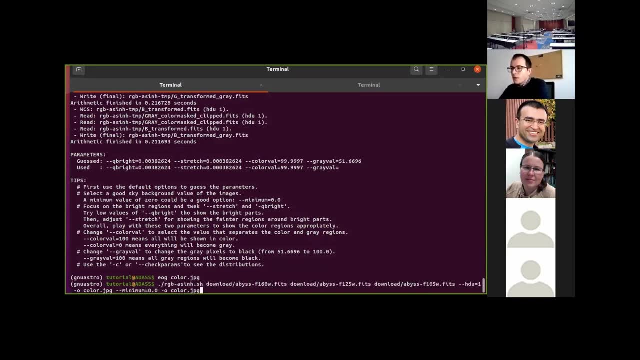 of this algorithm here. I am just trying to implement this to have a good tool for obtaining, for obtaining color images. So let's play a bit with the parameter. As you can see here, this is some of the guess that the program has done, And now I can use another one. So for 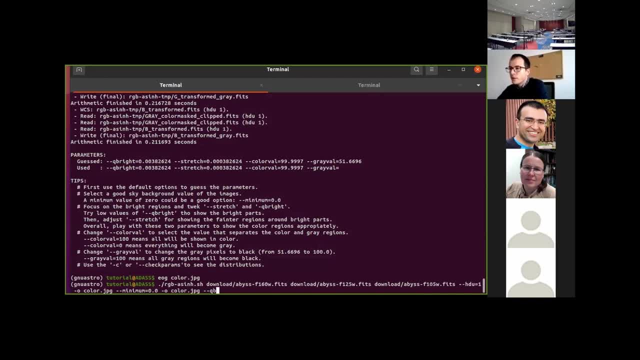 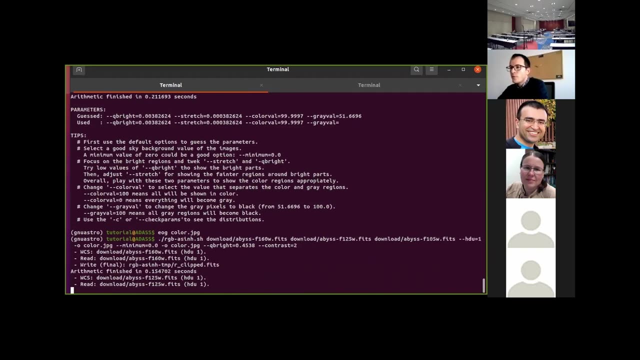 example, dash, dash, Q, Q, bright, bright, bright, Sorry, And let's put, for example, 0.4538, for example, and then implement it. Let's prove the contrast by a factor of two And then let's run this, the same line of code. 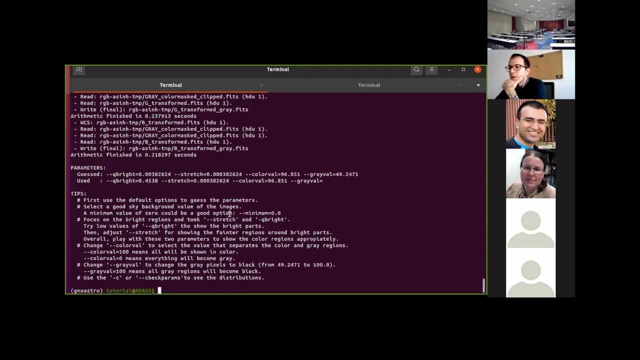 but just modifying this couple of parameters, And then you will see that now, well, you can see here that the parameters for the original ones were this one, Okay, And now we have changed these ones, Okay. So, basically, if we have a look here, G color image. 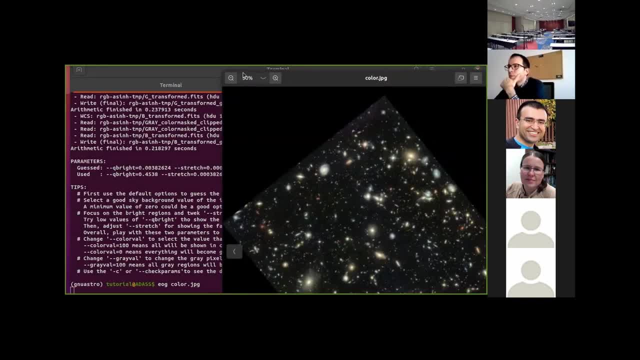 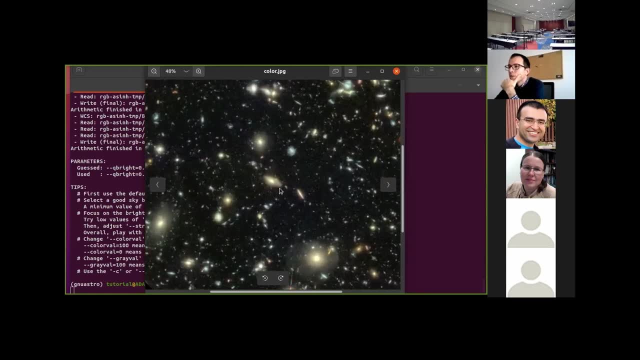 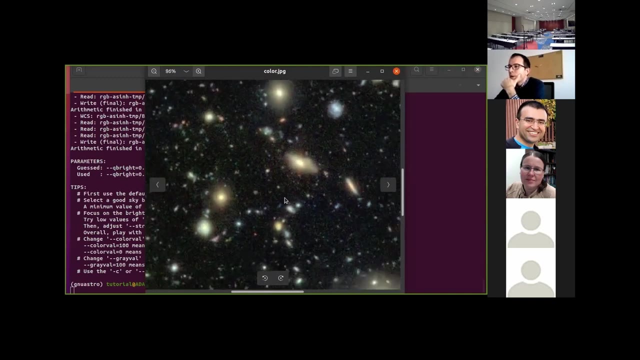 you will see that now the image has improved by a lot. Okay, So now we are able to see the inner part of the galaxies and the stars together with the outer part and the sky background in a much better way. So this is just playing a bit with the parameters, but in principle you will be able to. 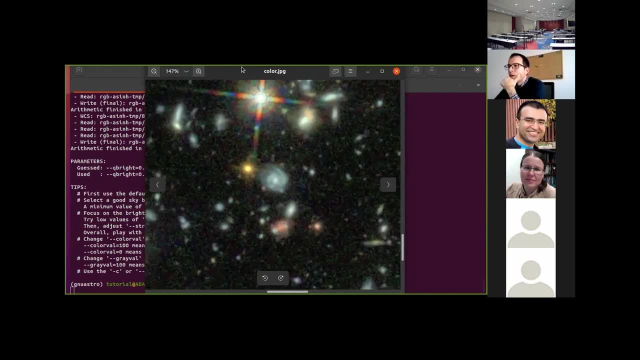 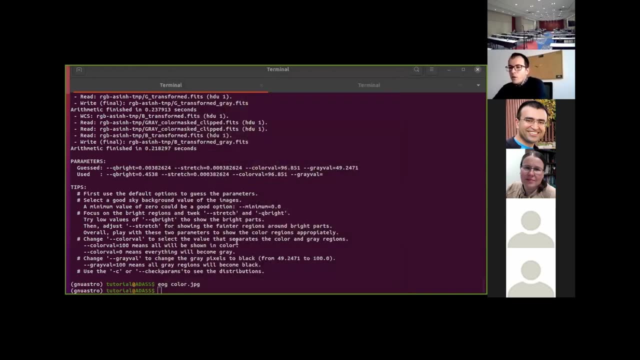 play and improve a lot of the parameters that it is possible to use With this, with this kind of scripts. So now I have some minutes in which I can keep going to show a couple of things about how to generate some profiles and making the convolution of astronomical. 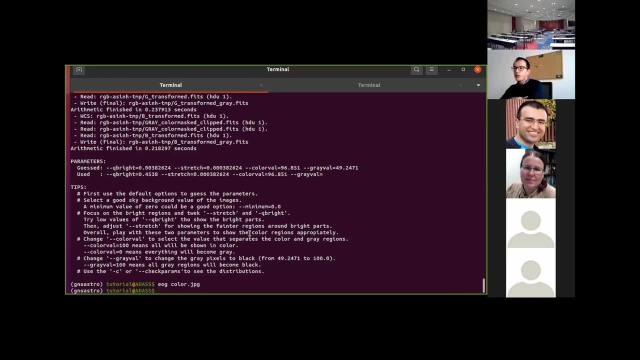 images. So let's, let's do this once we have- we have reviewed this script. For example, we are going to use the ASTM key, prof, And we will bring down ASTM key to a certain point here. ASTM key to this world. 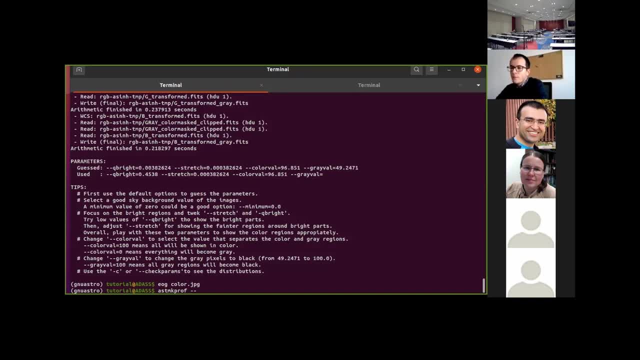 and create an alpha symbol and patients And Hey, this is ASTM key prof. This is ASTM key prof, Just say ASTM key. So So, this is ASTM key prof. specify that you want to have an oversample of one. So just one pixel. 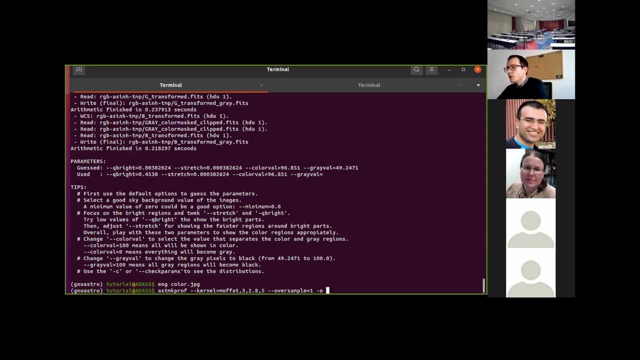 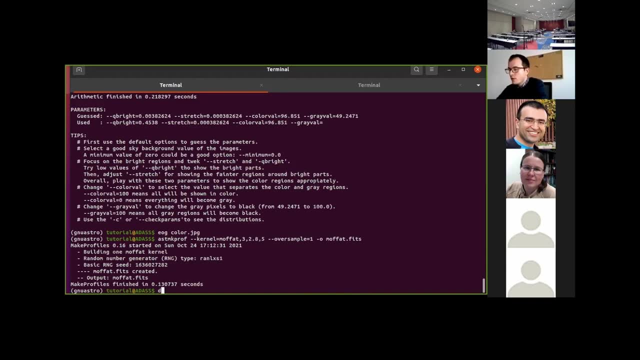 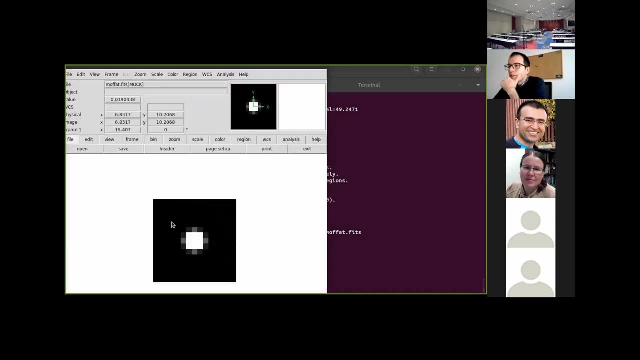 Oversample equal to one, and then the output that we are going to call MoFap. Okay, and really fast, it has computed this image. So let's have a look at the image MoFap, and you can see here that it is actually the shape of a MoFap. Okay, 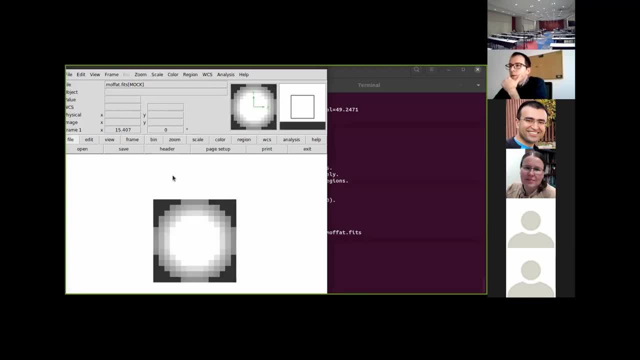 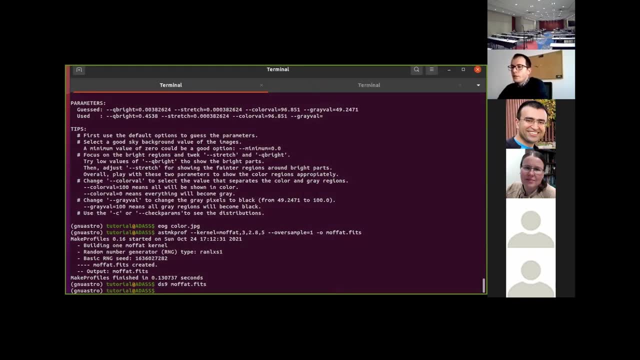 In the same way, we can specify that we want to obtain, for example, a Gaussian function. So for doing this, the MoFap- sorry, the Gaussian- only have two parameters. so remove the beta and then let's call this. well, you have to specify here Gaussian. 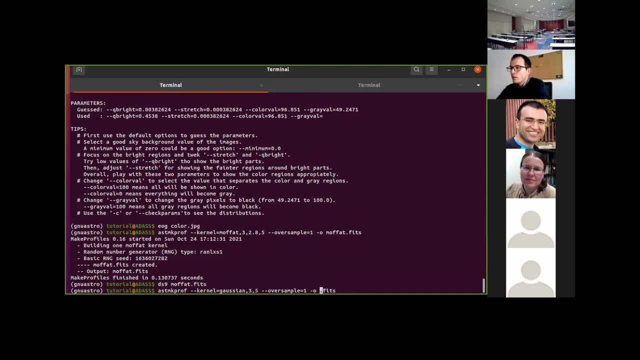 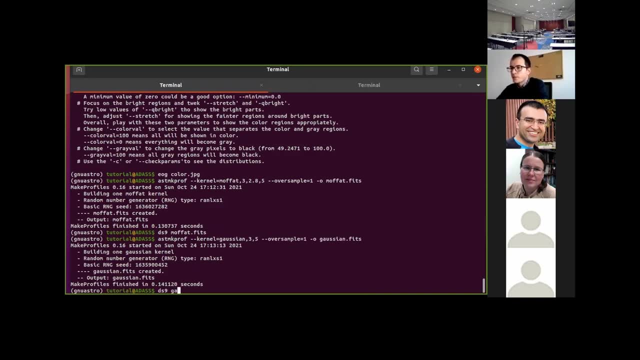 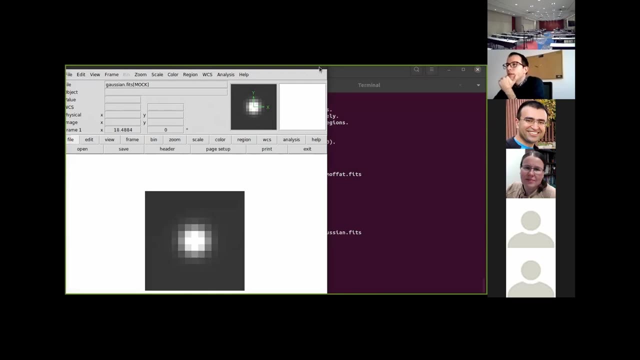 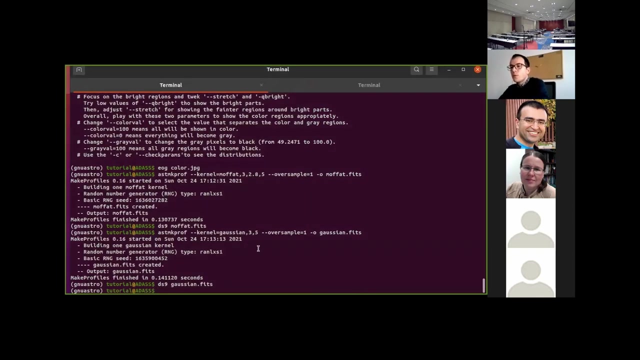 Gaussian, and then let's call it a different way, so Gaussian, and now it's gonna create a Gaussian function in the same way than before. Okay, Now we can use this Gaussian or this MoFap function to make the convolution of the original image with this kernel. So, and to do that, I am going to explain another program, which is AST. 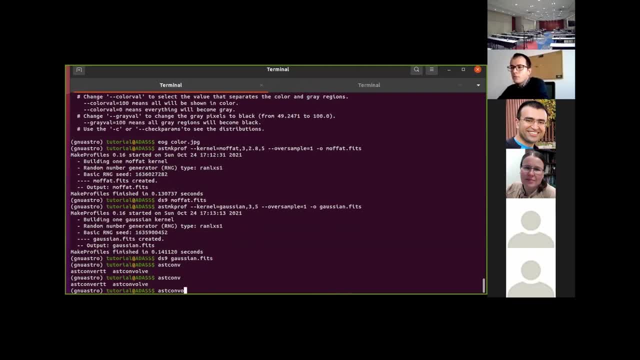 convolve. Okay, so now we have to specify the original image. So download this filter and then the kernel that we are using. So kernel, for example, the Gaussian, and the, the space in which, the domain in which we want to make the convolution. So in this case we are going to make the convolution. 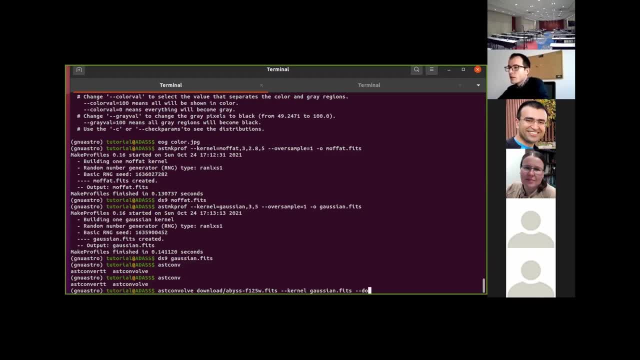 in the spatial domain. So dash, dash domain, And then spatial, and then the output name, So convolve, convolve dot fits. So again, we are using the input image and the kernel Gaussian that we have just created with the previous call to AST: make profile. 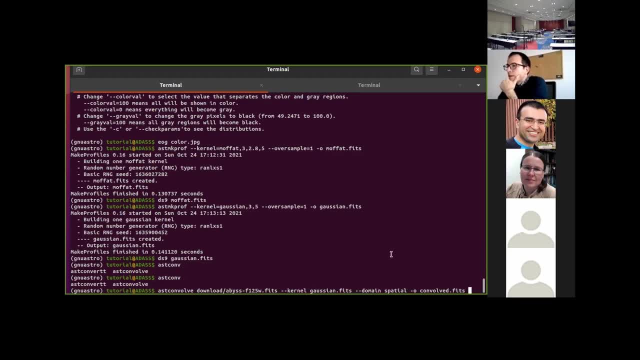 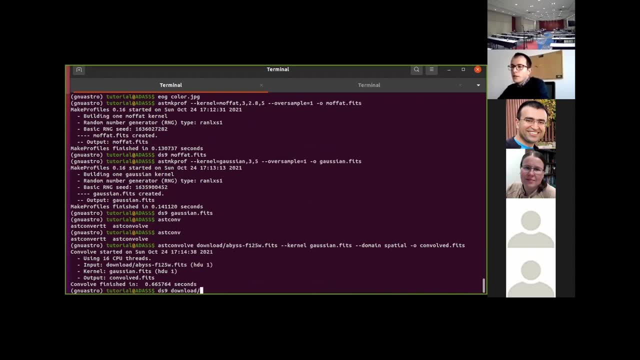 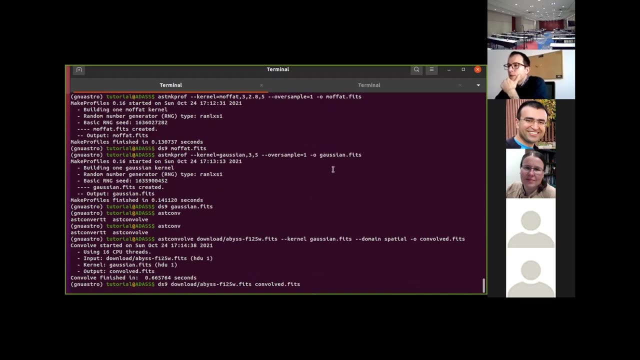 Make the convolution in the spatial domain. and then let's, let's do the convolution, Let's have a look so we can open the original, the original image, just to compare, and the convolve with DS9 at the same time, Just to see how we can make. 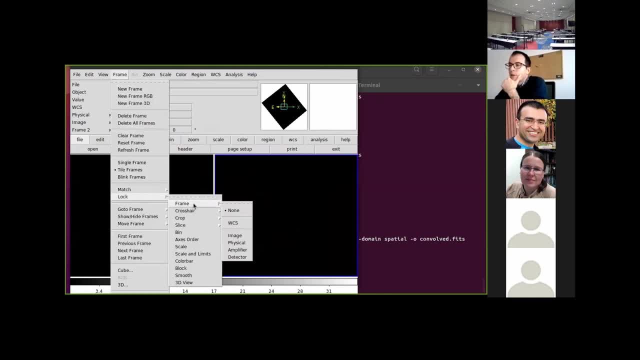 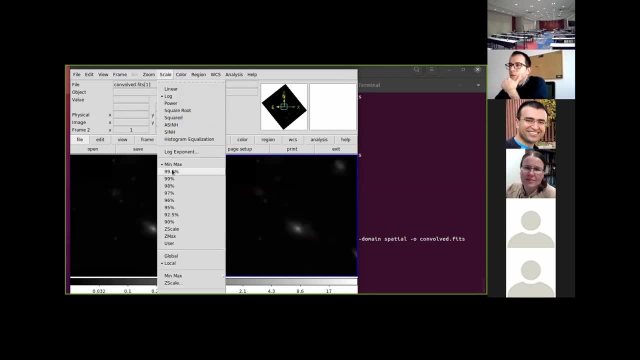 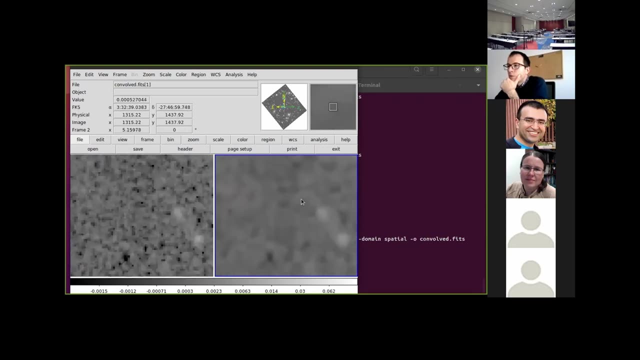 we have made the, the filter, the smoothing of the image. Okay, just to have a look here. let's match everything, just to compare the two different images. So, as you can see here, the convolve one has increased the signal to noise, But of course the 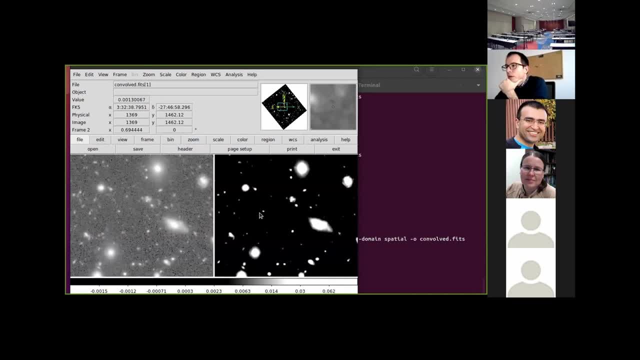 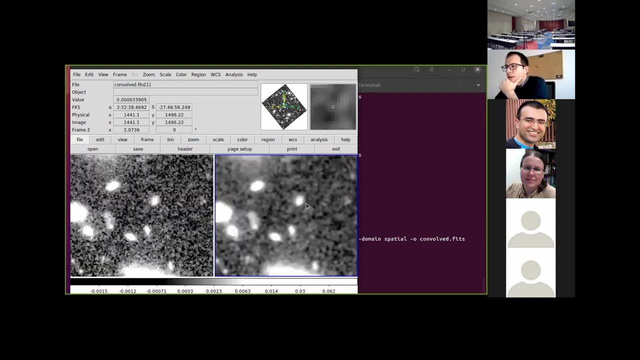 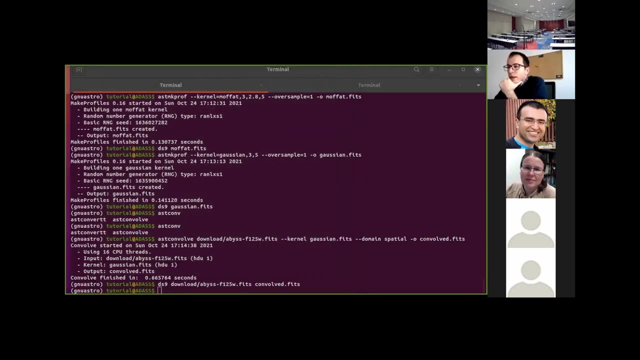 resolution has been decreasing. Well, not the resolution of the pixel, because the pixel size is essentially the same, but actually we have a smooth image. right, We'll make the conversion with the Gaussian kernel, So this is something that you can do directly. 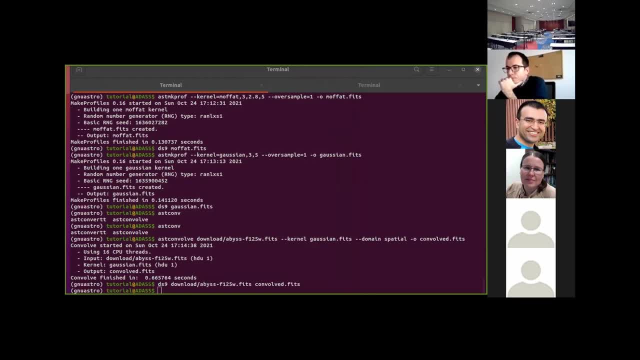 from the command line. And then, just to finish, I would like to show a very nice example on how we can use different other tools of Benoistro for making a catalog, a synthetic catalog, and then make a kind of a simulation of a galaxy with a stream. So here we are going. 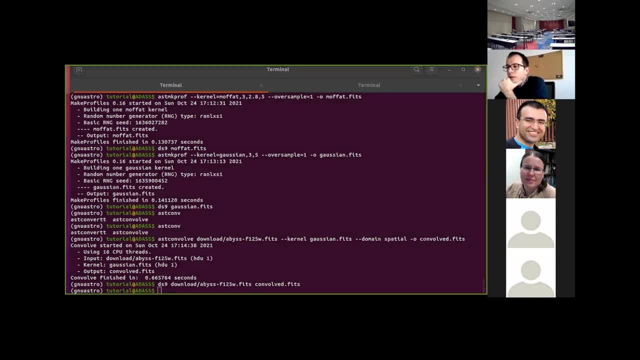 to make a catalog. Just let me copy directly this line. Okay, So this is a bit strange at the very beginning. You can ask to Mohammed at the Discord channel. but basically I'm going to put some parameters that will be used for AST: Make Profile for building some. 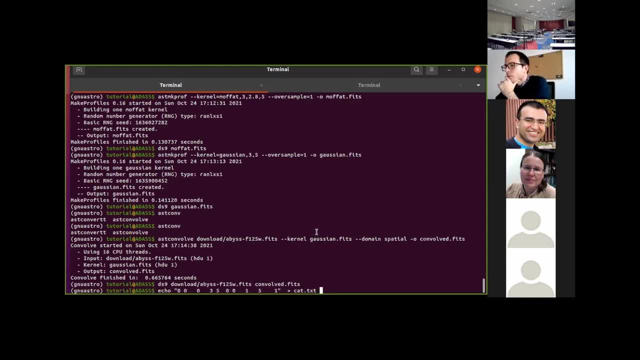 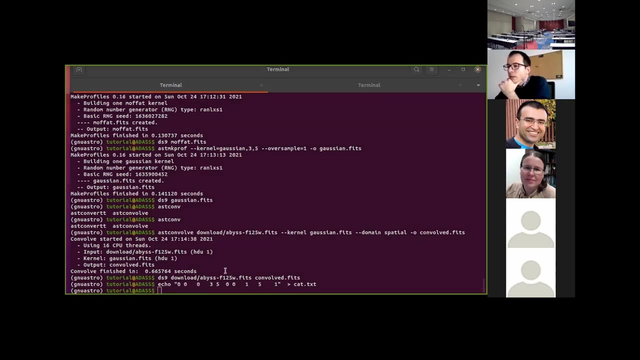 objects. okay, So in this case, for this one, we are encoding here the necessary parameters for creating the PSF. Okay, So, this is the PSF, And now we are going to put a galaxy which is a CERCIC profile. 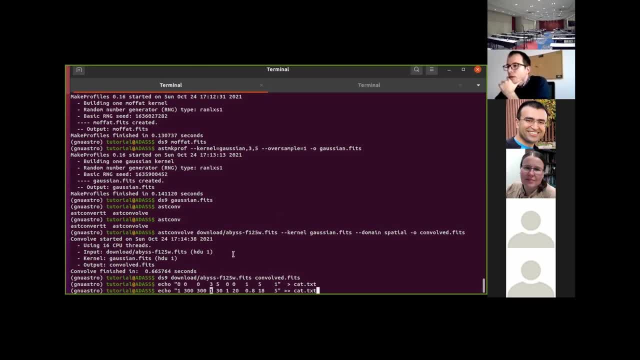 We say that we want to create a CERCIC profile with the CERCIC profile, And then we just make a CERCIC profile, okay, And now we are going to put a CERCIC profile with the CERCIC, an index equal to one, as you can see here- Okay, at this position, and many other parameters. So 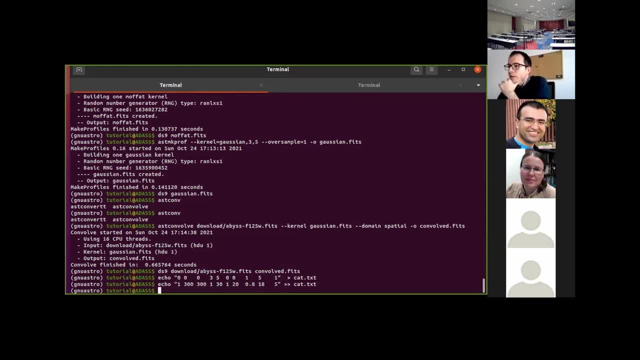 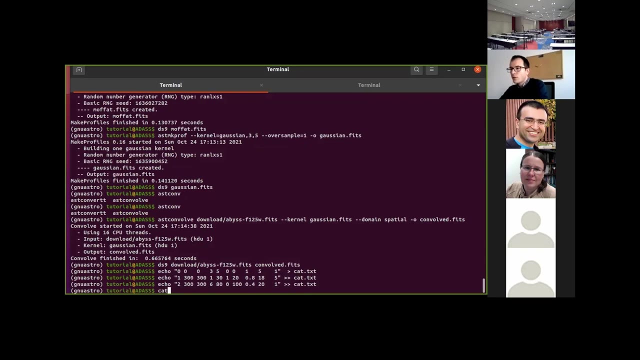 the position angle and so on. So let's keep this in the same file And then let's put a string, which is also a ring of pixels that we are simulating. So, now that we have created this file, let's have a look. So I've got the txt. This is basically the parameters that we are. 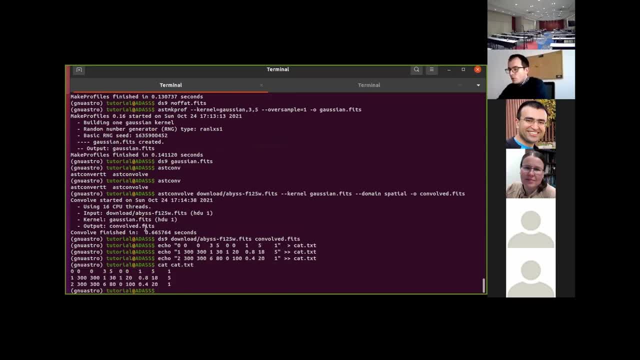 using for making the simulation. Now let's use ast make profile to make the synthetic image, So we can specify here that we have a particular size. So let's give the catalog catalogtxt merge size, for example, equal to 600 and 600.. The mode is in image. 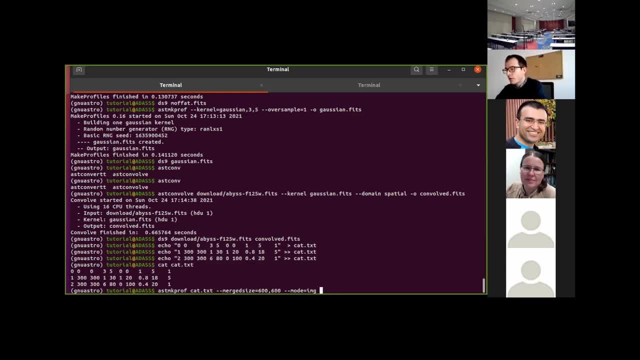 image, because we are not giving world coordinate, coordinate on the sky. we want to over sample this five times: zero point, zero point of equal to 30, for example, and then which is for the for the stream, equal to 20.. And then output, for example: 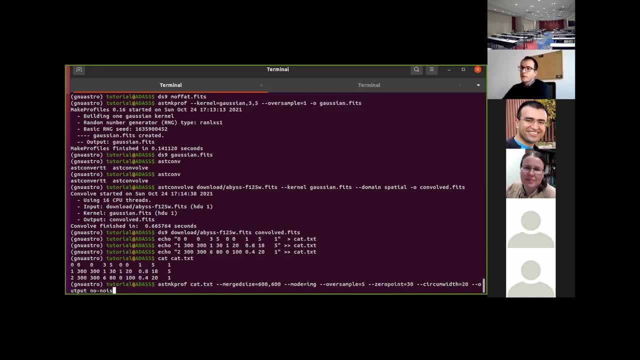 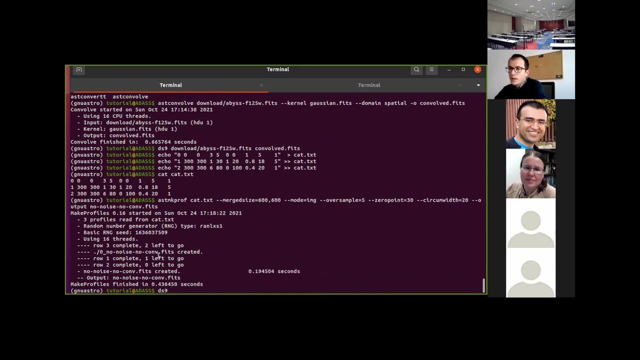 no noise, because this is not having noise yet. And no convolution, No convolve dot fits And it is going to create this synthetic image. Okay. so let's have a look at this image Really fast and you will see the kind of 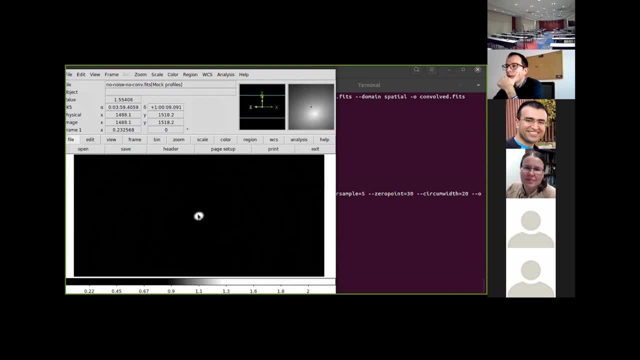 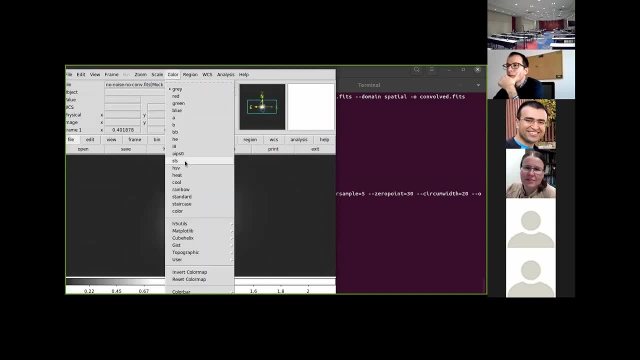 image that we have created. Okay, so the center, we have created the galaxy, And we have a ring here that corresponds to the to the stream. This has been computed only using the GNU Astro AST make profile with the parameters that we have specified in this file. 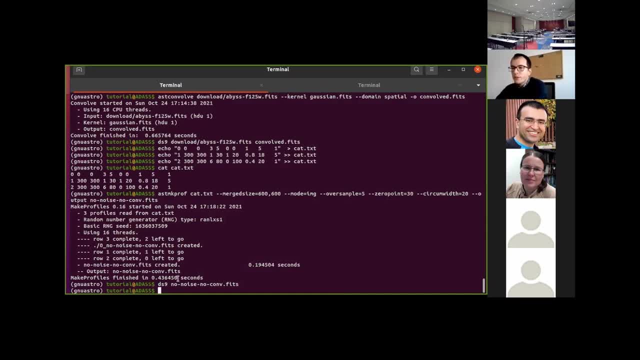 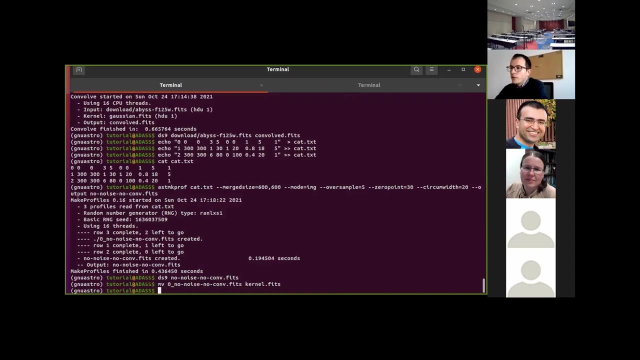 And now the thing that we are going to do is, well, let's move, let's move the this file, that that it is the PSF, the kernel. Okay, let's move on and call it like kernel. So this is this. could be a bit strange at the very beginning, but you have the instruction. 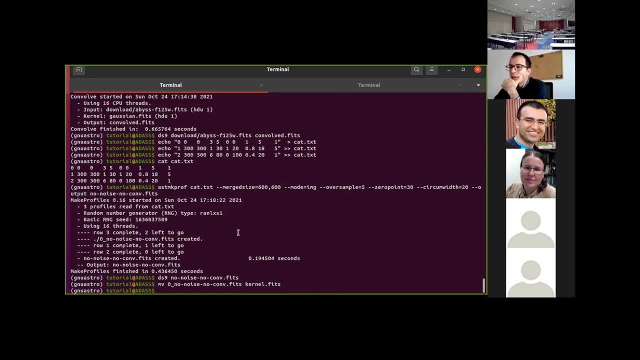 that I am following into the website And, in any case, you can ask to ask in the discord channel, So there is no problem. So now we are going to convolve the image that we have just created with the with the kernel. So let me just 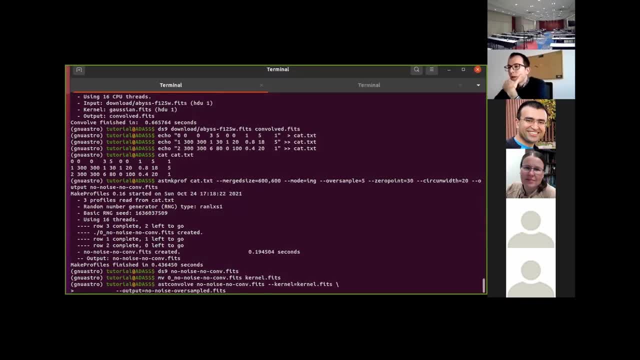 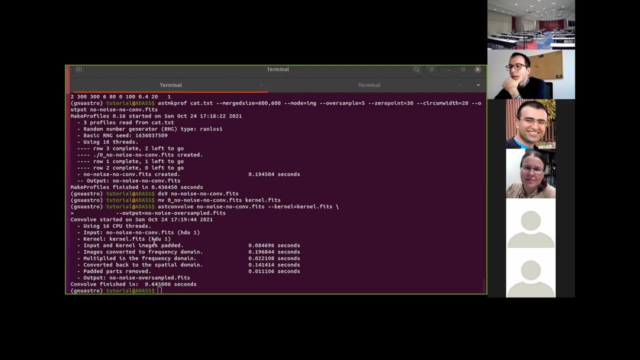 copy and paste the line that I am putting here. So again, AST convolve the original image and the kernel that you, that we have just created. just execute this And then we are going to warp, which is another program that I don't have time to explain right here, but you have the information. 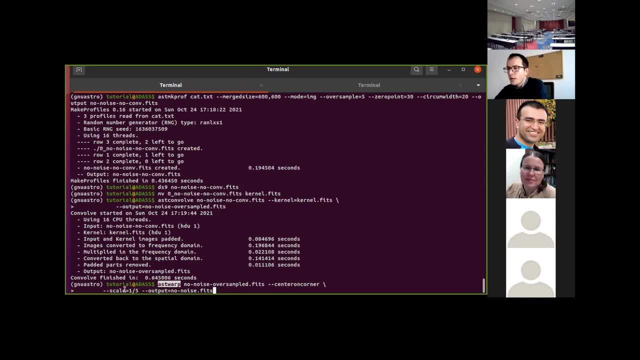 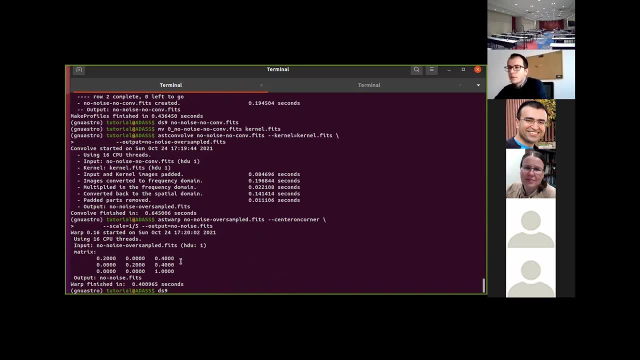 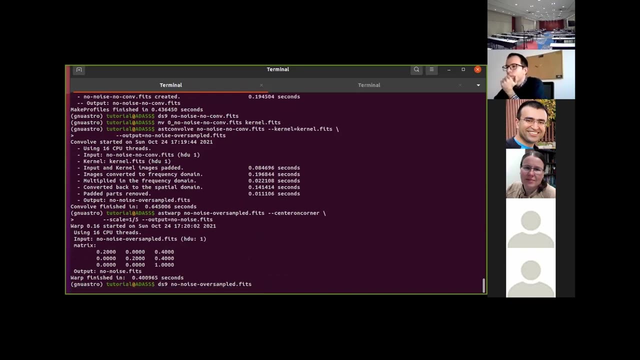 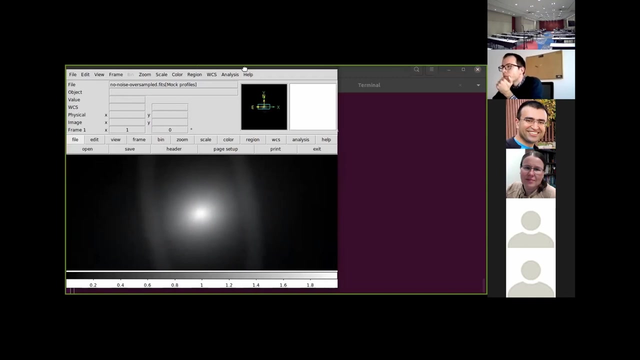 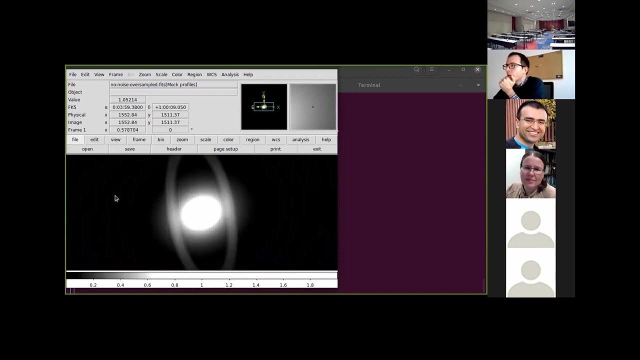 So we are working this, okay, we are transforming the pixel scale. So let's do this step. Let's have a look at this image And no noise, For example. okay, Note, you have 10 minutes left over. 10 minutes. Okay, perfect, Perfect, Thank you. So just to have a feeling of what I am doing. 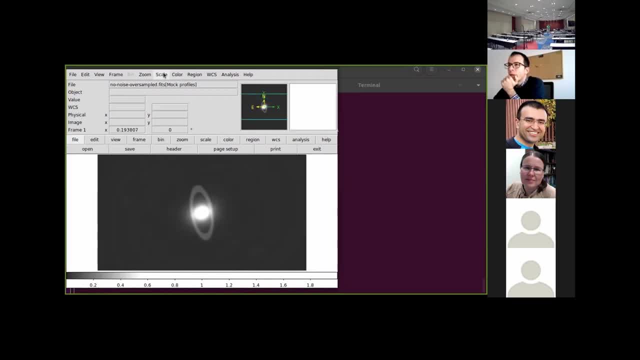 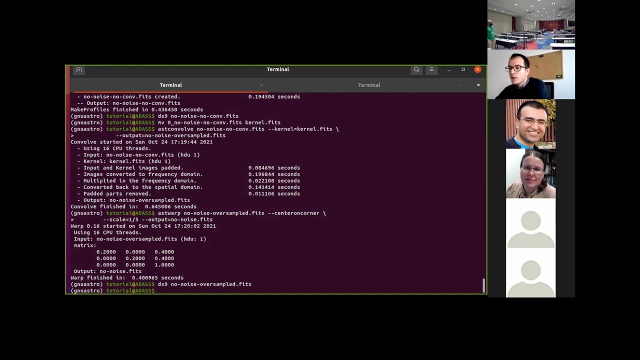 we have simulated some, let's say, some real condition of the observation, So we have resampled the image and so on, And now we are going to add, or we are going to add that noise. So in AST arithmetic we have that, the possibility of doing that with, with the 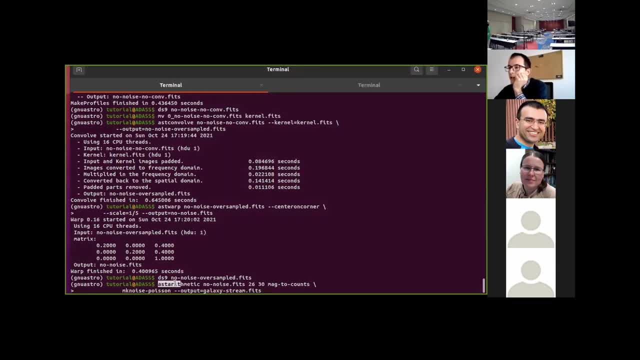 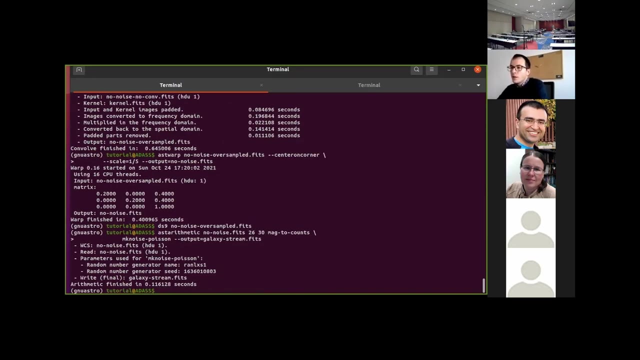 operator make noise. So with arithmetic I am giving us an input, the image that I have just created. I am going to transfer the nine to two counts and then make twice Poissonian noise And then the output, as you can see here, will be somehow a realistic observation of this. 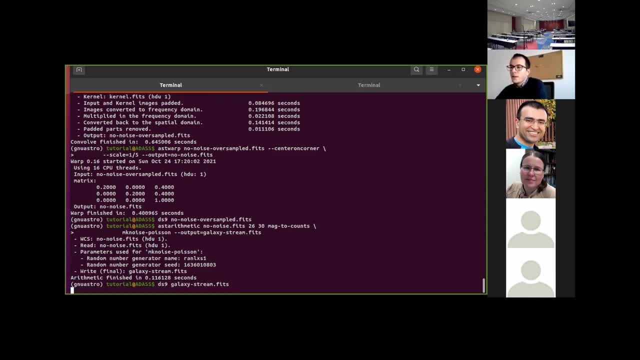 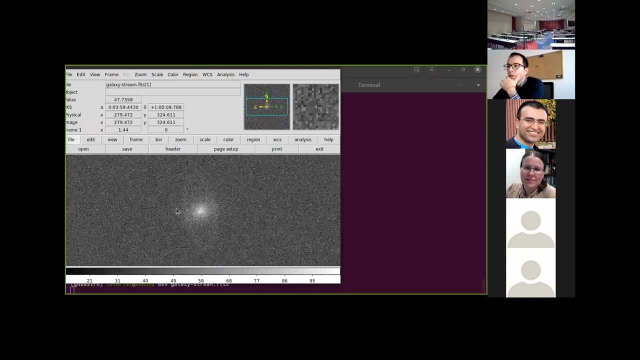 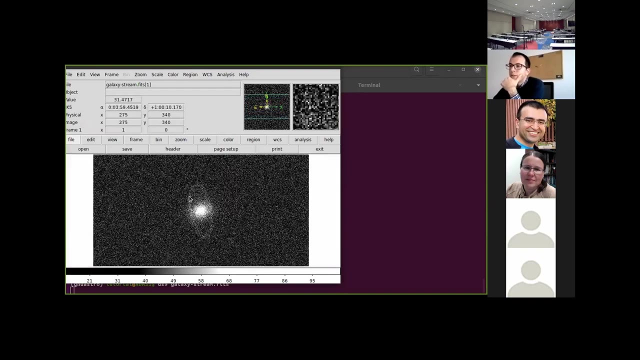 of this galaxy, galaxy, And this is the kind of simulation that you can do. Of course, this is very simple, But here you can see, oh, we have simulated a galaxy with a stream around this galaxy, And now we can start playing, for example, with no chisel for making the detection, or 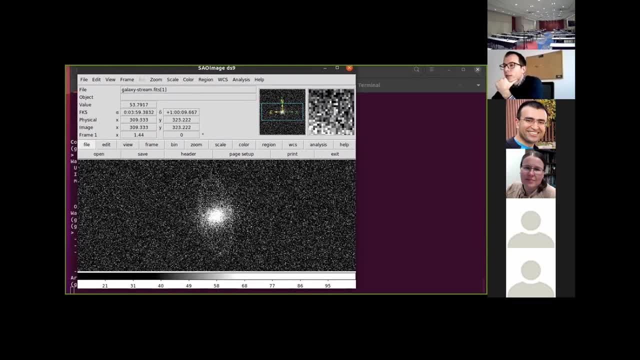 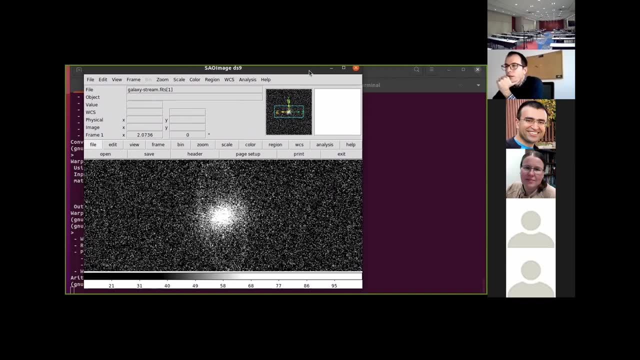 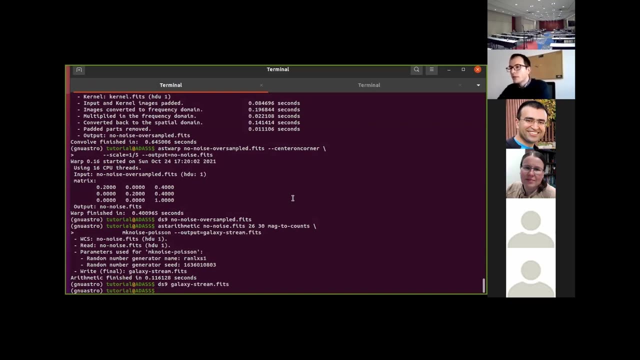 comparing our techniques with another different catalyst. Okay, and more or less this is all that they wanted to show, just to let you know that, of course, we have something that are not programs yet. So, AST, we have to review almost all the different programs. 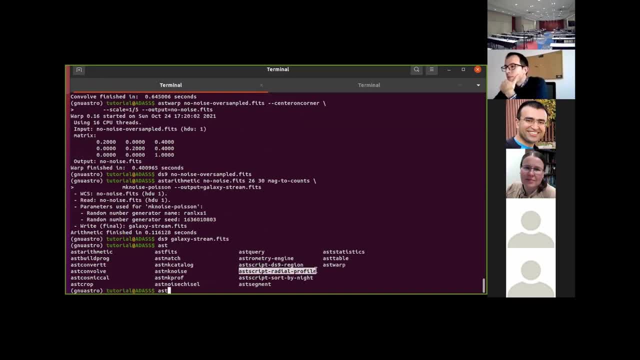 But then we have some scripts that, as I say before, they are high, higher level scripts. they actual script, as you can see here. So let's have a look. for example, if you type here which AST script, radial profile, this is a script for making the radial profile of astronomical images. 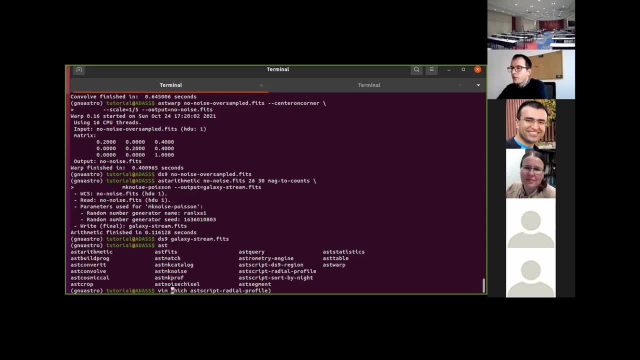 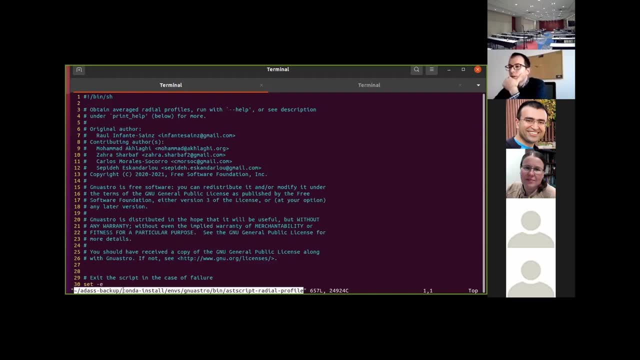 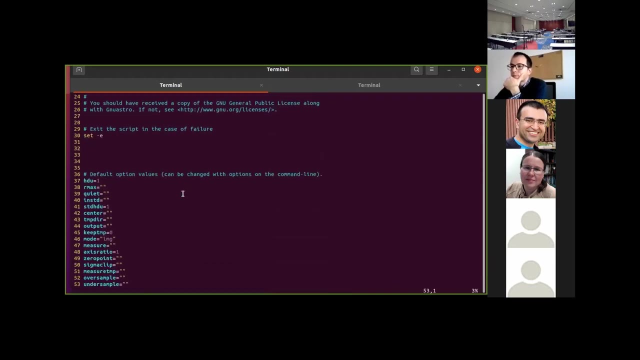 given a particular position on the sky. So if we have a look actually at the script, so it installed, as you can see here in this direction in the conda environment and this is actually a shell script, and you can see that we have developed this using many 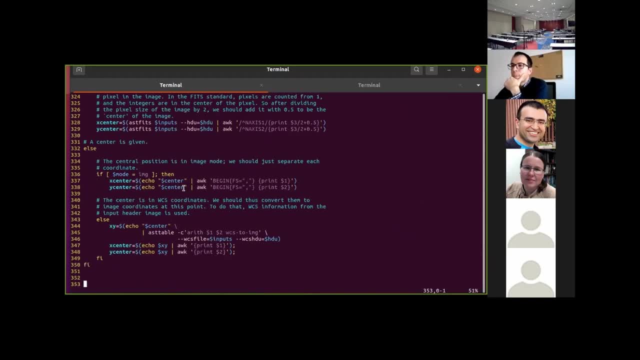 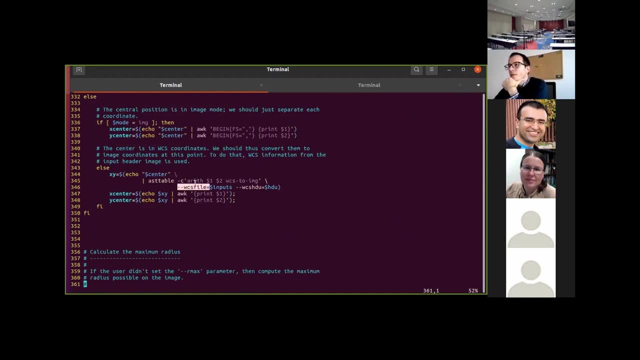 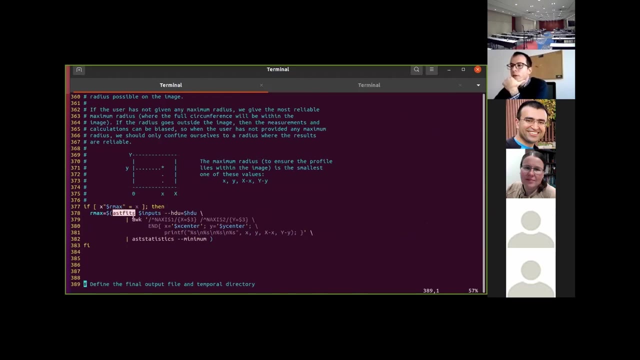 different GNU Astro programs. So here you will see that, for example, for computing the center, we are using AST table with the WCS parameters that we have previously used. For example, here for obtaining some parameters we are using AST feeds, then AST statistics for making the 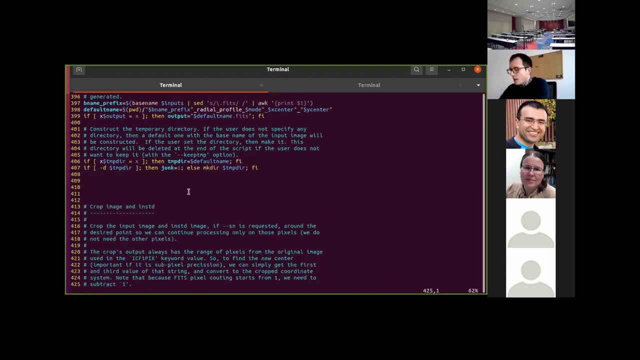 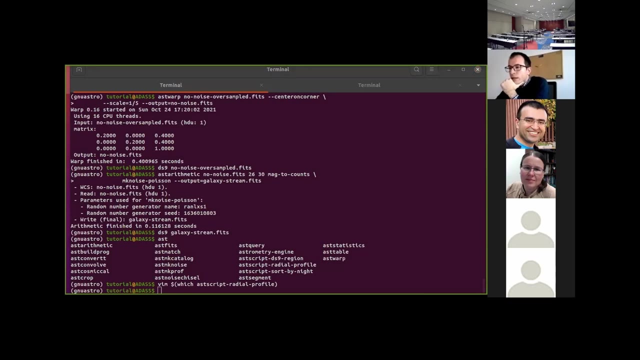 calculation of some parameters, and so on. So this is actually an example on how you can use the different GNU Astro programs to put all of them together into one single script for making the analysis that you want to obtain. Okay, and now, just to finish, let me say to you: okay, this is the notes that 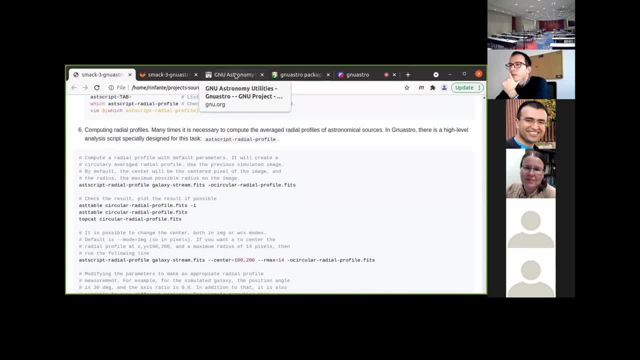 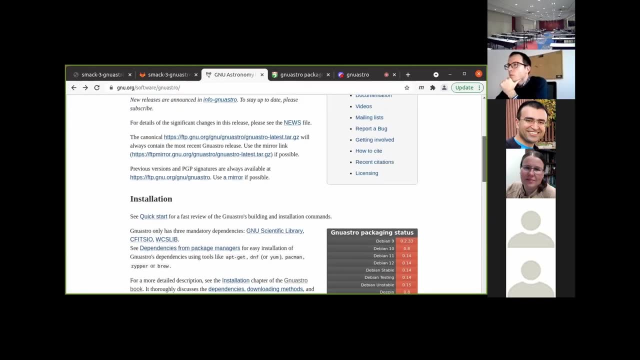 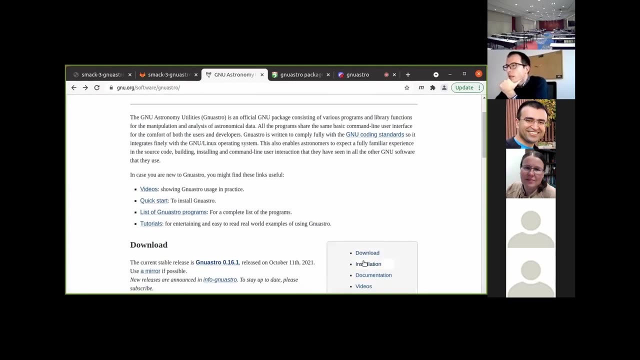 I have been following. You have all of them into the Discord channel, into the web page And just to finish, let me have a look at the GNU Astro book, Just to say to you that, even though we have used in this tutorial the conda installation, 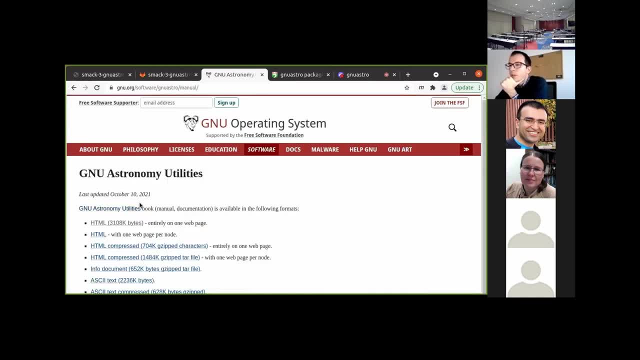 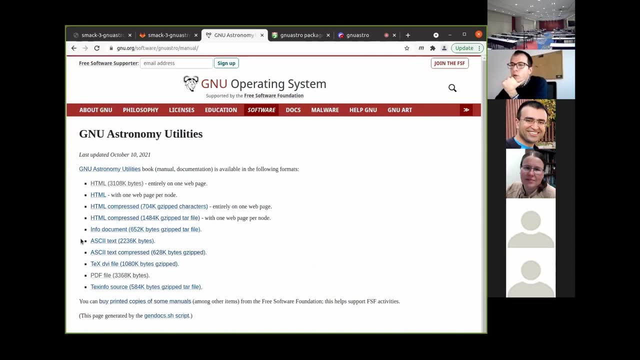 you will see that the GNU Astro has very few dependencies, So let me make this window a bit bigger. So here you have all of the different formats in which you can have a look at the documentation in HTML directly on the website. So you have here. 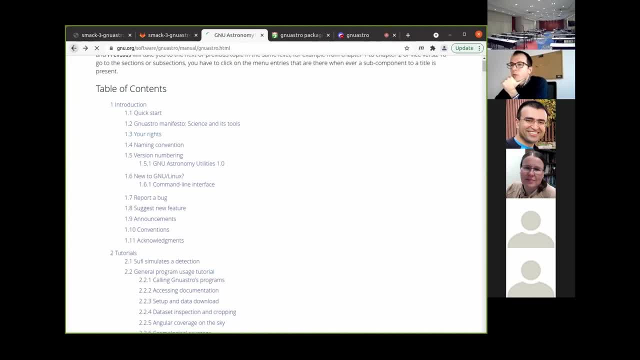 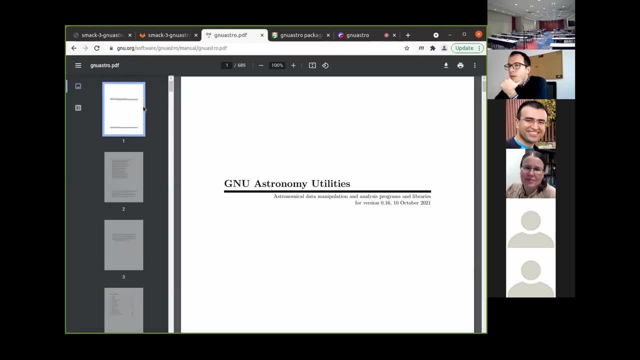 the index, the table of contents, but of course you also have the PDF, the already compiled PDF, in which you can have a look here. So this is the PDF. As you can see, here we have different sections. We have a very wonderful section in which you can start playing with nice tutorial. 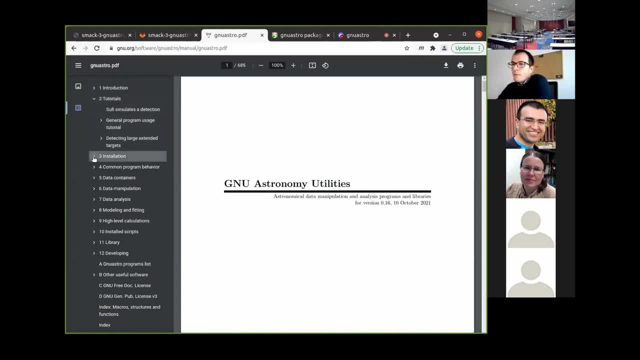 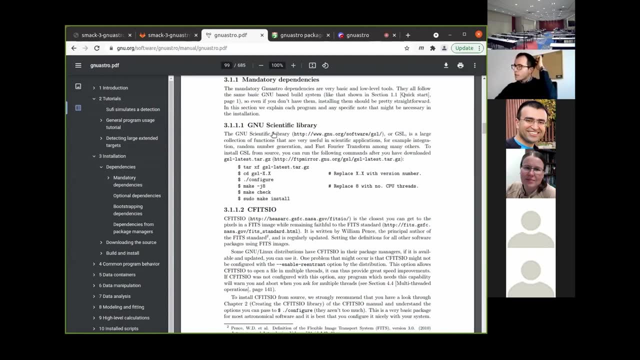 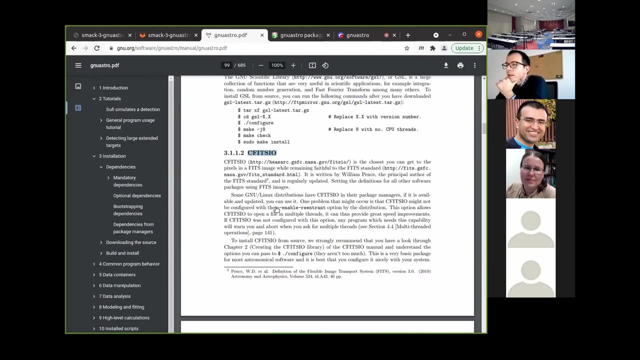 from the very beginning. Okay, and then about the installation. you will see that, depending on the dependencies, that we have to install GNU Astro from scratch, there are just three. The first one is the GNU scientific library, Cfitzio, and then the GNU- sorry- the WCS library. 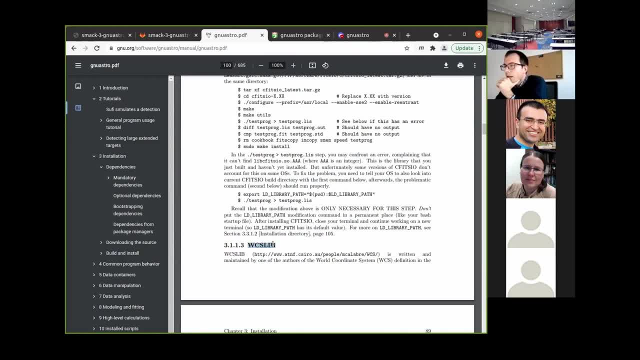 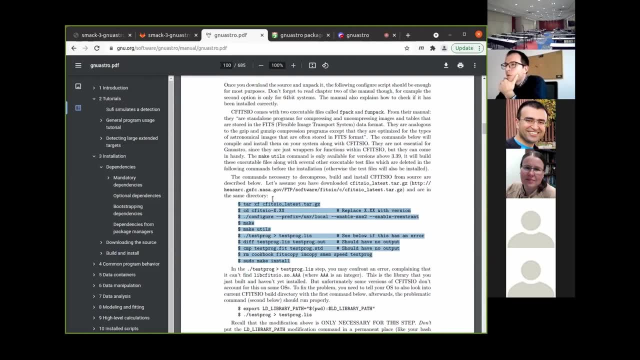 that you can see here. All of them are explained here in detail and actually you can see here that you have the different steps that you need to run on the command-line for installing all of them And of course also GNUwebio also has control pages and other things, comments, So I'm just going. 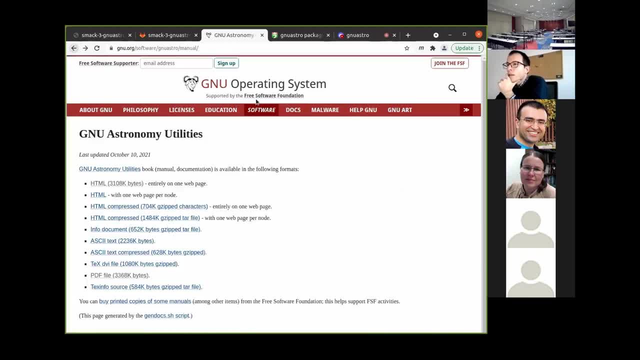 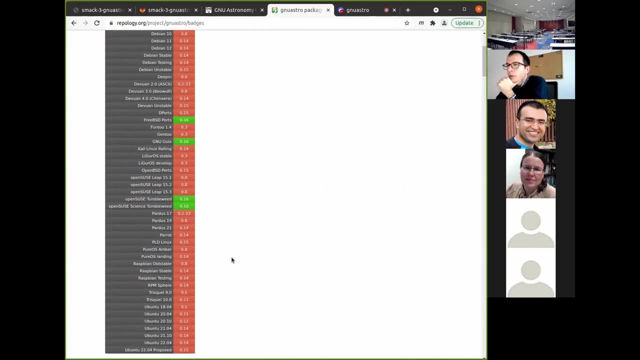 GNU Astro itself from scratch. So, since it has a very few dependencies, it is possible that many different Linux distributions have already compiled GNU Astro. You can see here the list of all of the different GNU Linux distribution that has already compiled GNU Astro. So, for example, compared with AstroPy. 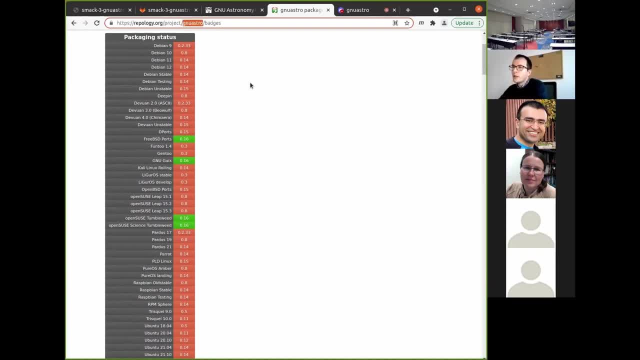 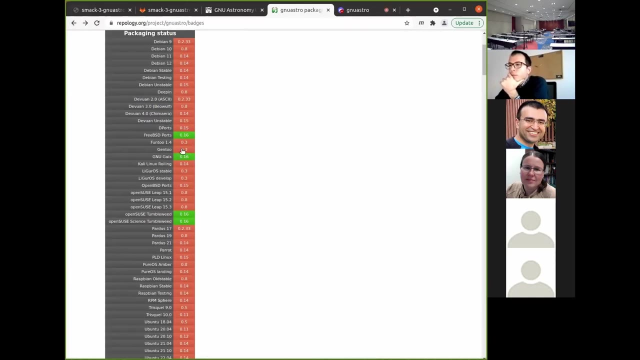 and because AstroPy have many different dependencies, some of the Linux distribution are not able to compile them as easy as GNU Astro right Py, you will see that the list is much smaller And actually some of them, some of the distribution has already the latest version. 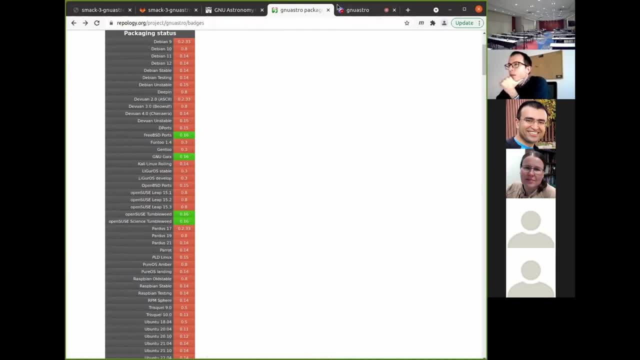 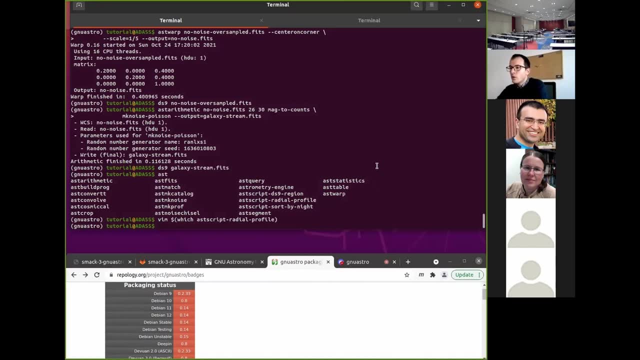 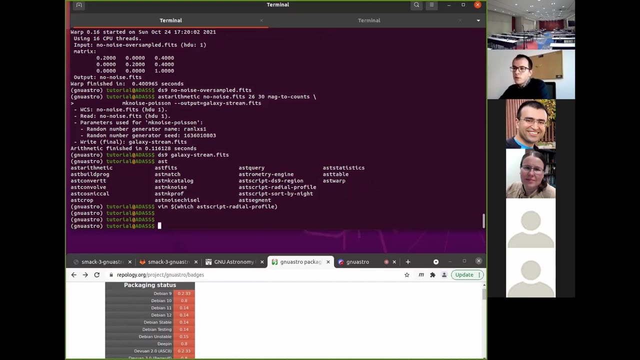 of GNU Astro, as you can see here. And then just let me finish showing that, of course, if you find the GNU Astro is useful for your particular research, you can use the feature Cite. So, for example, imagine that you are using noise chisel. 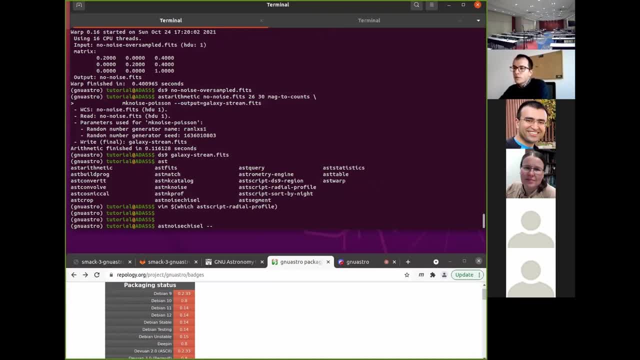 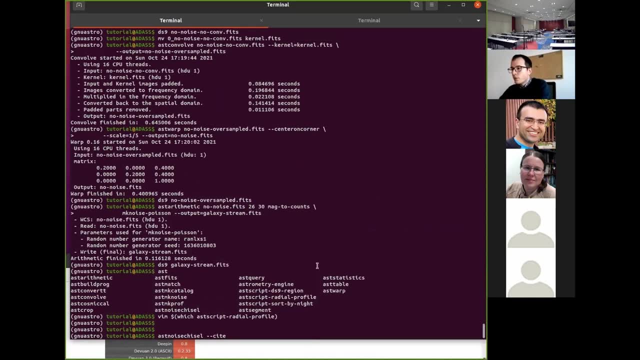 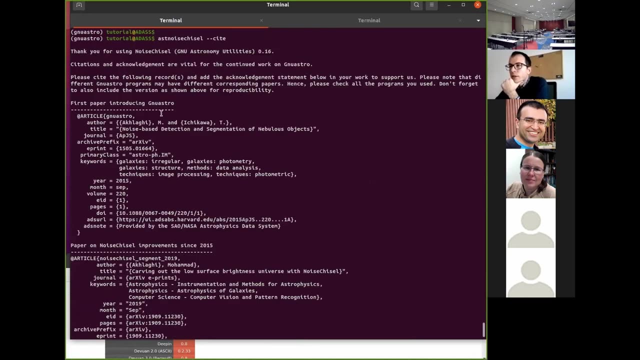 I used the noise chisel. You have the option dash, dash, Cite, sorry, Cite- to have a look at which paper, which documents do you have to cite in order to acknowledge, for example, this particular program which is GNU Astro? 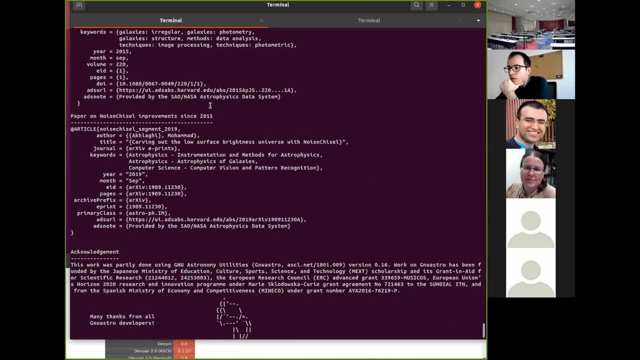 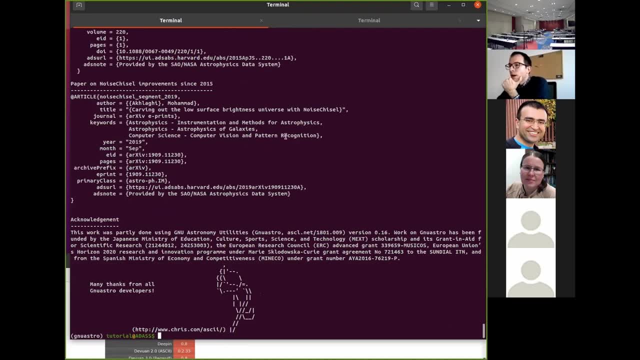 So I will finish here. I think we have time for a couple of questions. So thank you very much to all of you to attend for attending to this tutorial. I hope you have enjoyed it. Thank you very much. Oh, and Mohamed, thank you so much. 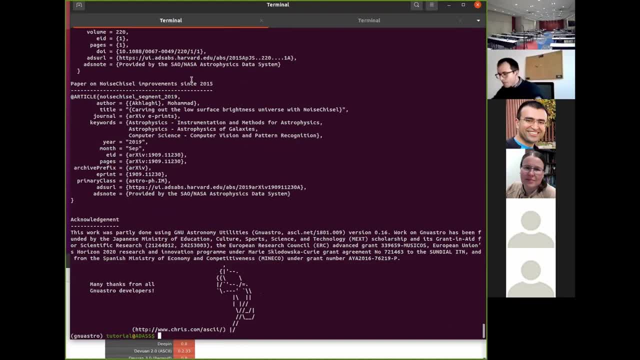 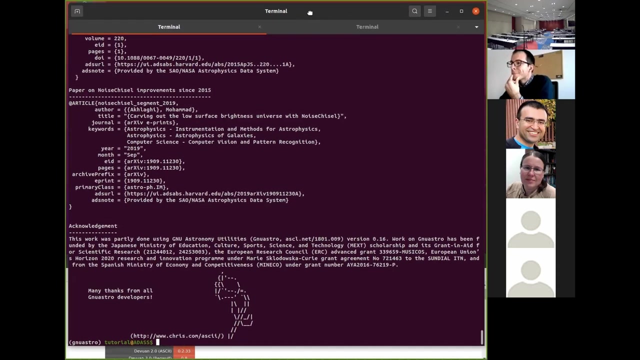 That's a great talk. I think we can give them a round of applause here. Thank you. I don't know if the the participants here in attendance have been following this call, but that's been very active. Is there any questions from the group here in person? 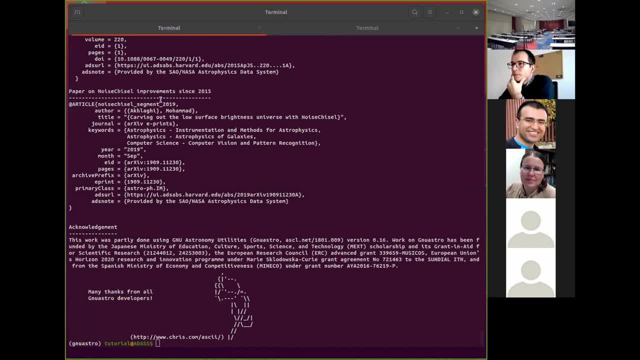 that we can ask or we can use the microphone here. if you have any questions, You can come up. Yeah, sure, So I think somebody is talking, but I cannot hear. Some of you are hearing something. No, no, we don't hear. 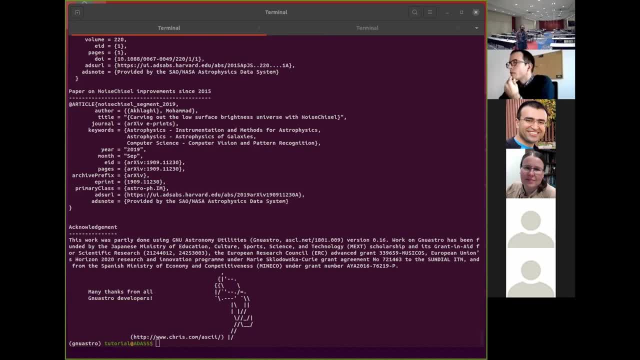 We don't hear anything. So, Mohamed, please feel free to ask. answer the question if you think No. no, I see in the video that someone is talking, but I don't hear anything. Okay, And now? Oh, yes. 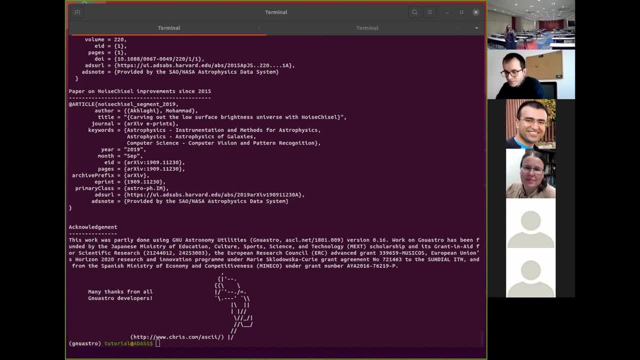 Yes, Okay, cool, Thanks. So I was particularly interested in the feature that creates the RGB images. Is it possible with GNU Astro to then overlap with GNU Astro, to then overlap with GNU Astro, to then overlap to overlay contours of another image? 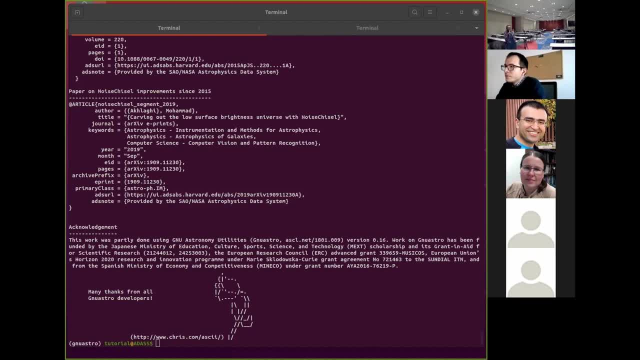 on top of that RGB image and then export it as a PDF or PNG or whatever. You know how you can do that with Apple Pie, with Fitzfigure. Is that something that's possible with GNU Astro? So you mean, for example, make some annotation. 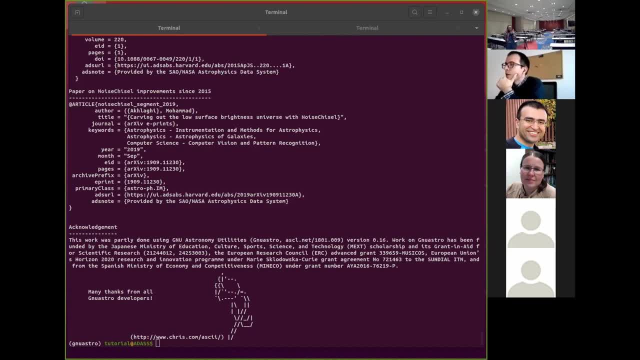 So like putting arrows or some text within the image- Yeah, some annotations or whatever it is you want to do, and then export it. Well, actually, with the programs that we have, I think it is not possible. Correct me if I am wrong, Mohammad, but it can be. 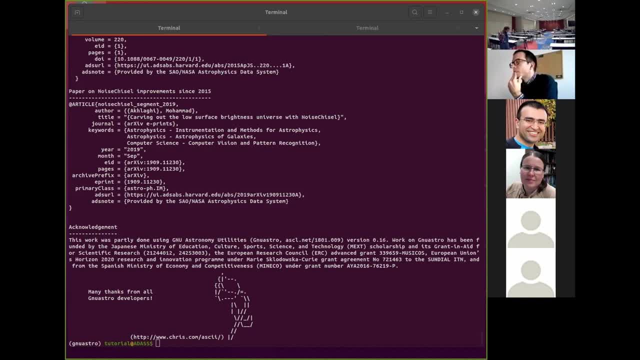 Go on, go on. No, no, go on. So the thing is that, Raul, I'll send you this link of this paper in the chat that you can show. So this is a trick. actually, It's not that we have right now. 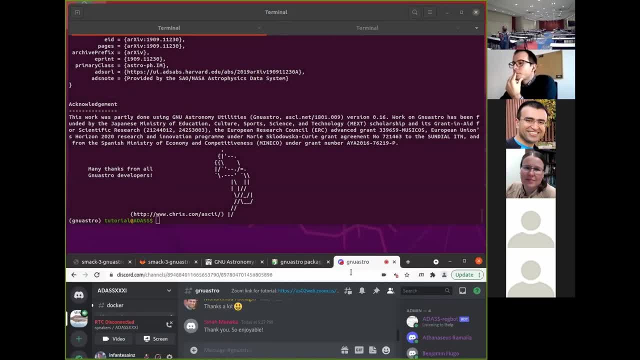 Do you have the chat in the Zoom? Yes, What I've done was to manually play with the color channels. Yes, that what I've done was to manually play with the color channels. Yes, that what I've done was to manually play with the color channels. 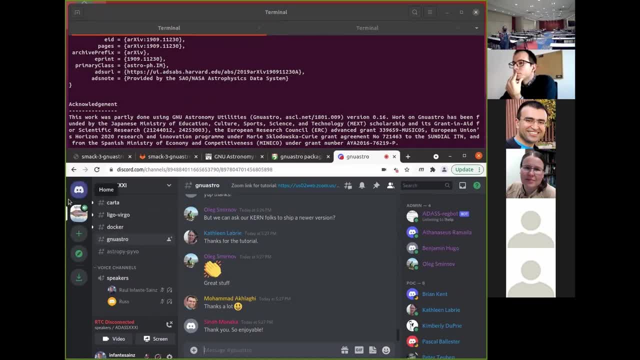 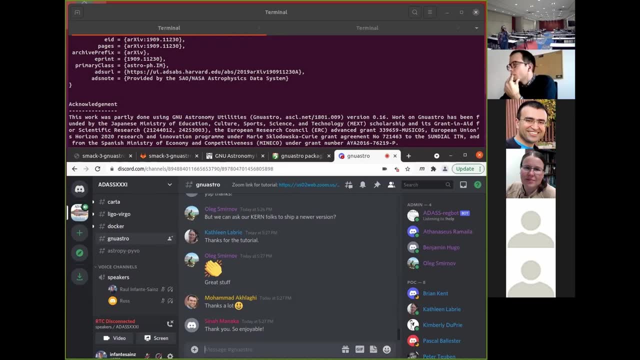 to add the contours that I wanted And you see, it works nicely. But yes, Raul, if you can show it. No, it's in the chat of Zoom. Sorry, I should have put it in, Ah, in the chat of Zoom.